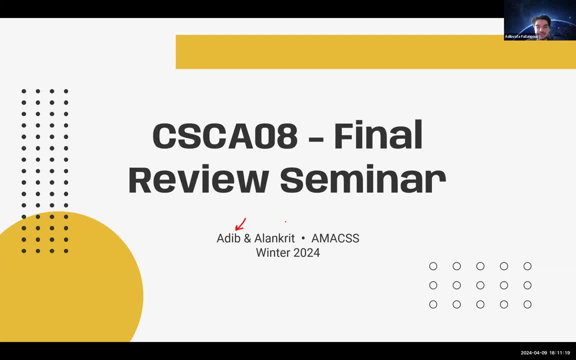 The seminar is hosted by me- this name here- and Ellen Crick, who's in the chat and will help you guys out. So if you have any questions, ask in the chat. I'll also monitor the chat. so in case you have any questions, I'll see. Now today's agenda is going through. 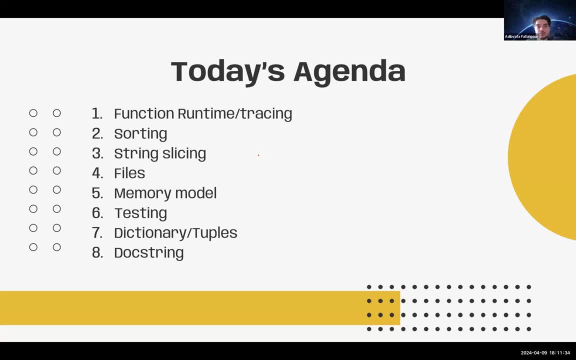 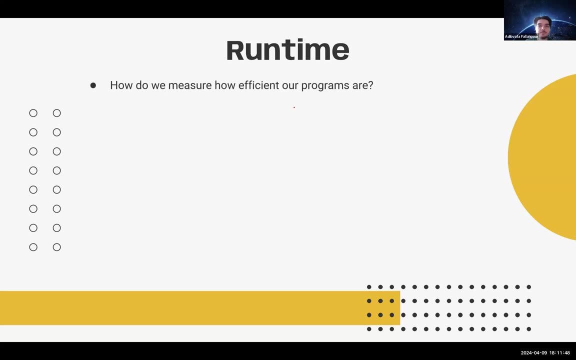 some of the most important topics of the course and we will do some past final exam questions in the main way as well, And also this is a good chance for you guys to ask your questions about anything that's missing. So first start: we're going to start with functions Now. you guys have 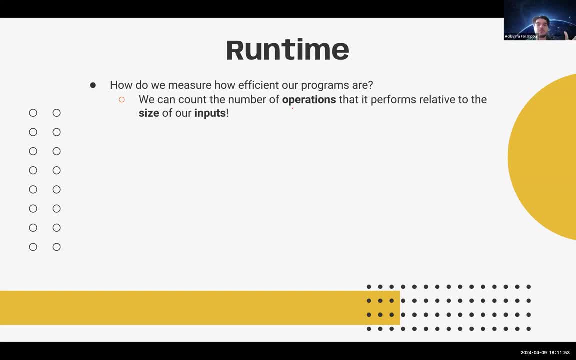 learned about function runtime. you know the function, the different number of operations and it depends on the sizes and the inputs they get, And operations are, in general, defined as anything That involves math. Is it a comparison, Is it a summation, Is it a negation? Multiplication: 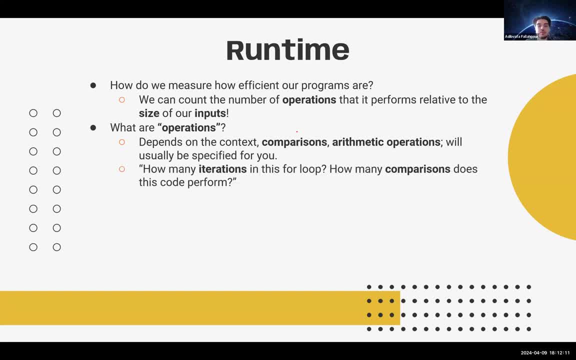 Anything is constantly in operation And, for example, the number of iterations you have in your for loop will be an extra type of operation. Your if statements are another operation, Your checks in the while loop are operations And our inputs are your data types from lists and 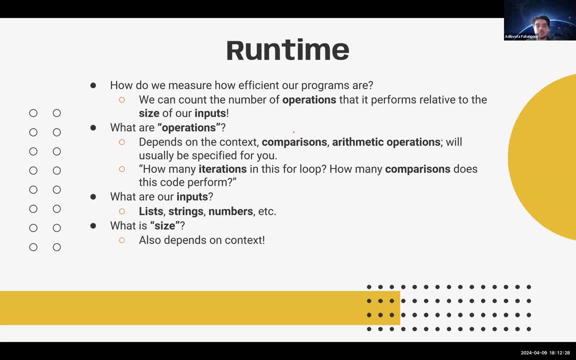 strings to numbers and integers, And size is considered to be either the length of a string or the length of a list. It could depend on what exactly the data type you have is. It was just like a quick overview of runtime. I guess you just quickly caught a bit worse And we're going to 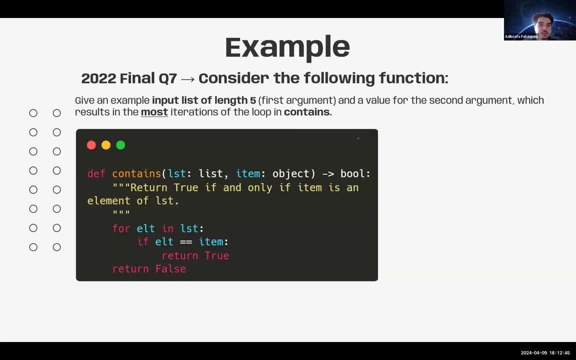 have an example from the 2022 final exam. So as we go through, we have different examples And these examples are probably easy enough for you guys to solve, But I'm going to go through them, since there's a lot of them and we don't have time. But if you have any questions or if any part of the 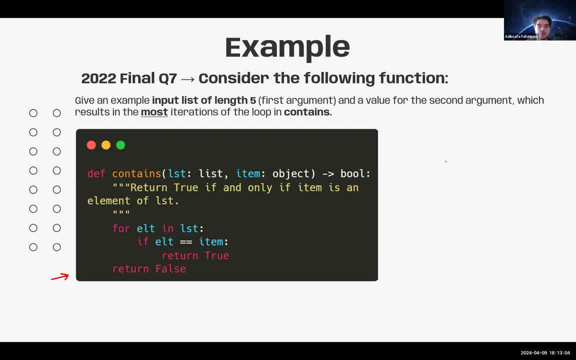 argument is not clear, definitely ask. That's the only way we can make sure you're all on the same page. So, for example, here you have a function that starts with a for loop, has an if statement somewhere in here and then ends, And now you're asked to give an example input list of that five. 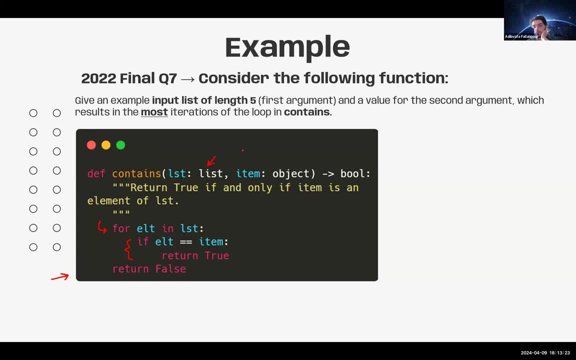 and a value for the second argument, which results in the most iteration of the loops. So does anyone have any answer? Just for warm up, That was like a spoiler. So, for example, if you have any questions about the for loop, it's basically the most important thing to figure out is: do you want to do the same feature? 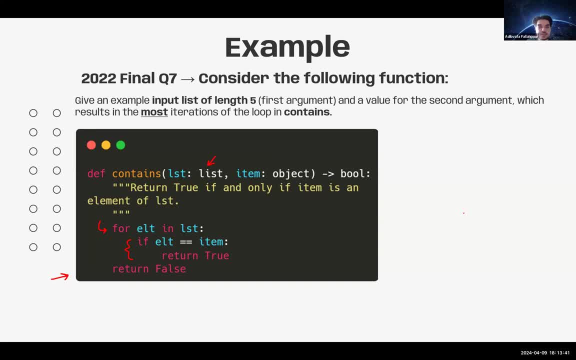 And the answer you'll get is: give me a完 Any one suggesting anything. So, basically, what you're trying to do is you're trying to give an example list as to the input of this function, such that you maximize the number of iterations this for loop gets. 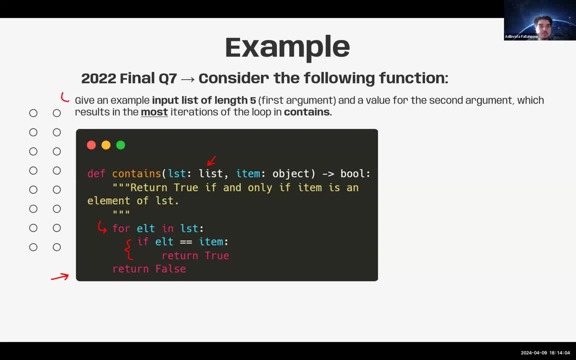 Well, the question is here. Given an example, let's say there's a list of five elements being input here and there's some item as our second argument. Now we want to have the most number of iterations of the loop. In other words, we want to have the most number. 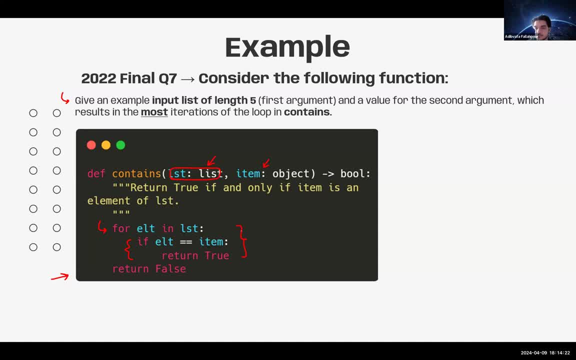 of four loops running Exactly. So, as you guys mentioned, we could have five elements and the item is not in the list. Why? Because this way, you're going to be checking through all the items in the list, You're going to also check the if statement, and it's never. 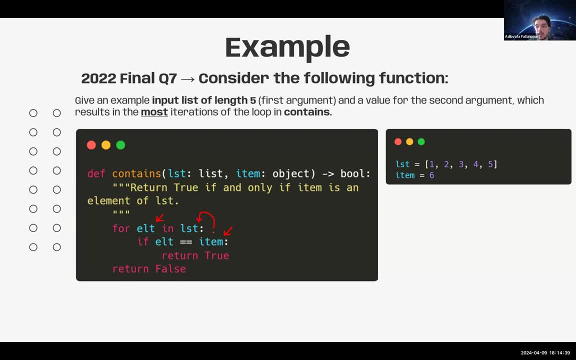 equal to true. So you're going to be just going back through the loop again. Keep in mind, if the item number six, for example, was inside the list like this was six, then your for loop would terminate here. So once you see if last is equal to this item, it. 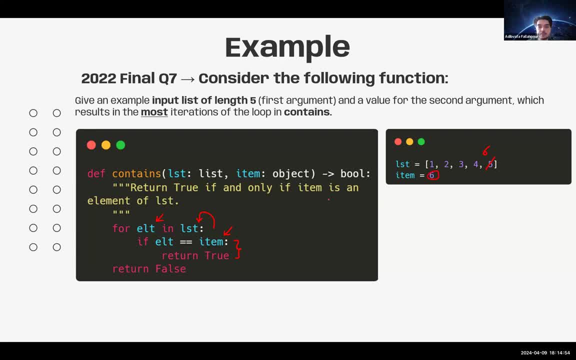 will return true. However, if six is outside, it will go outside the loop. So it will return true, Not execute return true. It will go back and it will execute return false. So putting six inside the end of the loop will not make any difference. Like it will have the same. 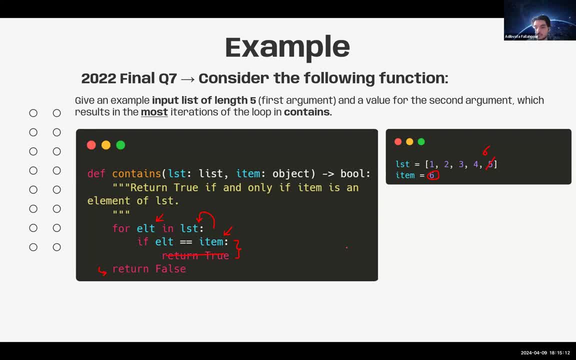 number of if statements being considered. Yes, if item is in the end of the list, it works. So there are different examples and this is one of them, But the key idea here is that you want your item to be either in the end of the list or not in the list. You 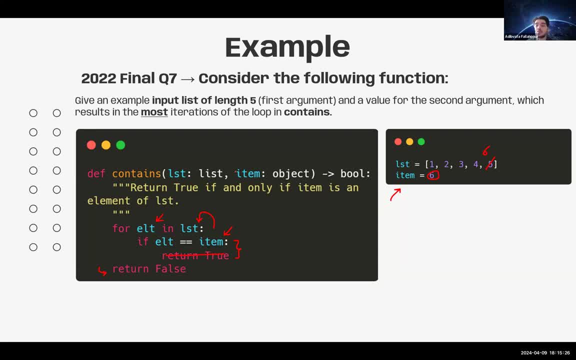 don't want it to be in the middle or in the beginning, And this was a final example question, So you can see it's pretty easy. Again, a lot of you just gave me correct answers, So please be confident. Like you know, if you're going to exam, be happy, Have some shine around. 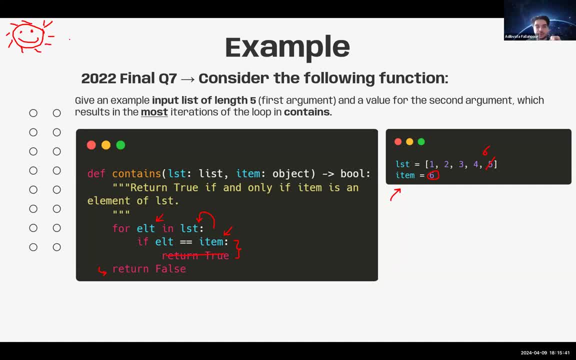 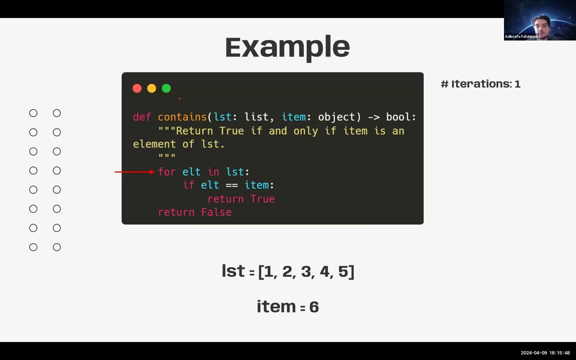 you, You know, go for the exam, Take all your strength to it and make sure you get the marks for these easy questions like the one here. Now, this is a visualization of the iterations, just to be on the safe side. So you know the first iteration you check for. 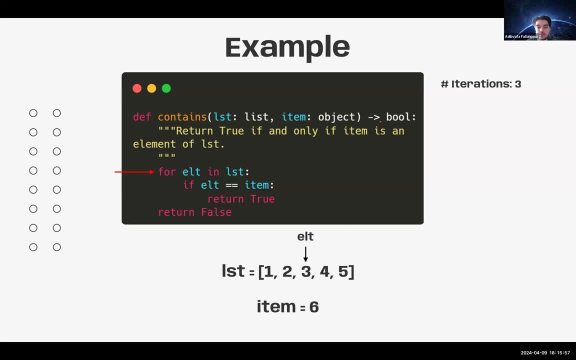 number one, Then on the second one you check for number two, Then you check for three, Then for four, Then for five, And ultimately you just return false. If this was six here, for example, then you would just return true, So it won't. 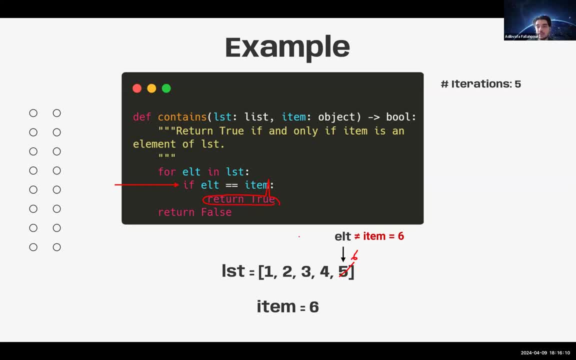 really matter if it's six or five, But what matters is it's not in the beginning of the list. Yes, the quote will definitely work, because you know we are having two different return statements, based on if the item's inside the list or not. No, If the item is. 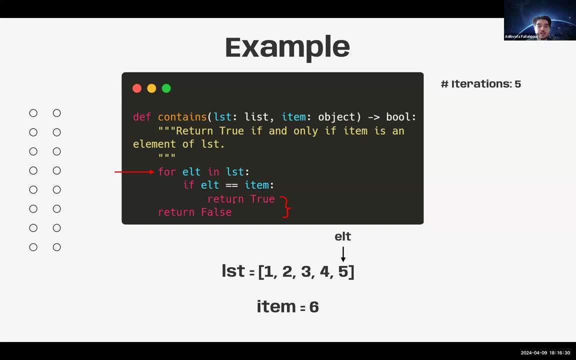 not inside the list. we will not do a six iteration. The reason for that is the for loop here will only run for the items in the list. How many items do we have? We have five items, so it will run five times. It doesn't care what is inside, It doesn't care what's. 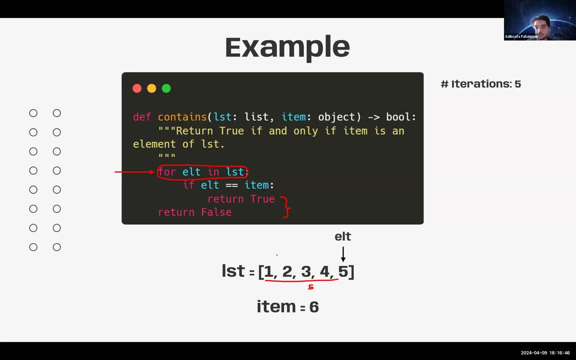 happening. As long as you have five items, it will run five times. Now, if this was a while loop like we had while you know well this won't be correct, but like if you had some while loop saying while you have not yet found, 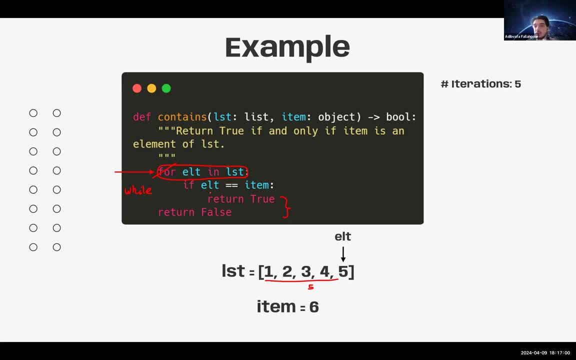 ELT in the list, et cetera, et cetera, then this will keep running for eternity. But this is a for loop, so it will not run for more than five times, So don't be tricked by these type of things. And here you see that the last time just returned, true or false, depending. 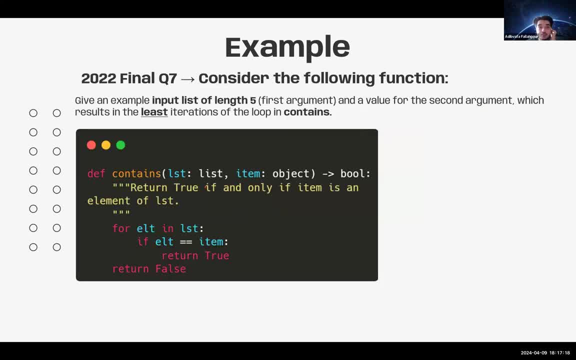 on the outcome Now, just to re-trigger what we went through. So a for loop will only run for, let's say, five times. Okay, Let's say finite amount of time, Like you know how many times it's going to run In. 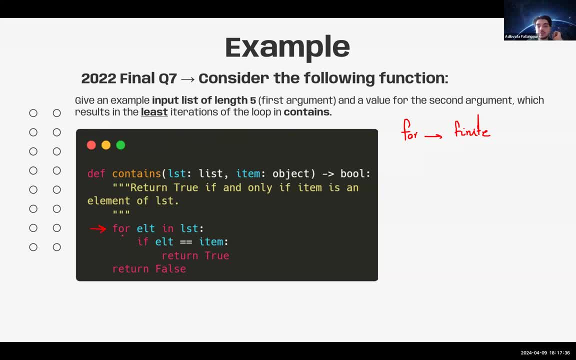 the first line that you call for loop. that's where you already know how many times the for loop is going to run. But a while loop will run until there's a condition, And that condition could be never satisfied And your for loop, your while loop, will just go all. 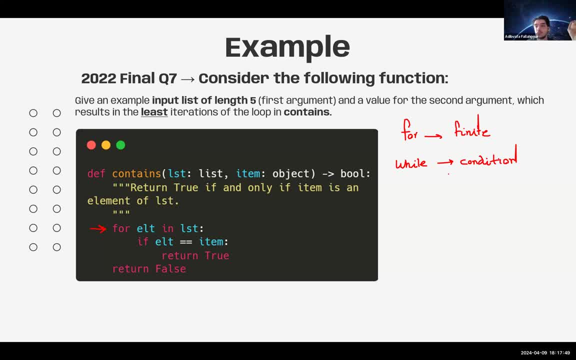 the way to infinity, Or that condition could be satisfied in the first iteration. so we're done, And that's a key difference. If you do not know how many times your loop should run, you should use a while loop. If you know how many times it should run, you should use 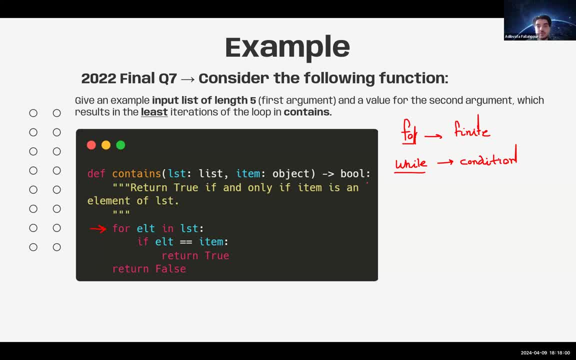 a for loop. So make sure you know the difference between these two because it could get tricky. Now the same example. Here we want to do the least number of iterations Instead of why does it jump. So we are trying to do the least number of iterations. I'm pretty sure you. 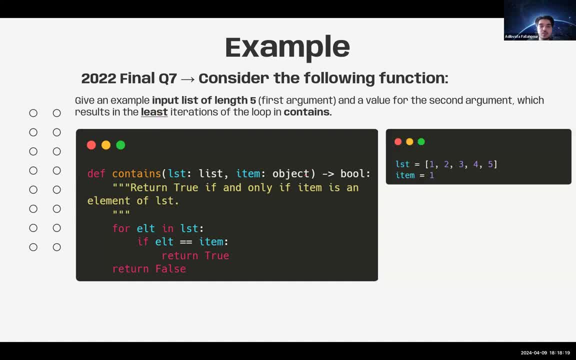 guys can quickly answer this, so I'm going to go through it. If you want to do the least number of iterations, the first item in the list will be equal to what we are looking for This way. the first time we go through a for loop, this if statement will be true. 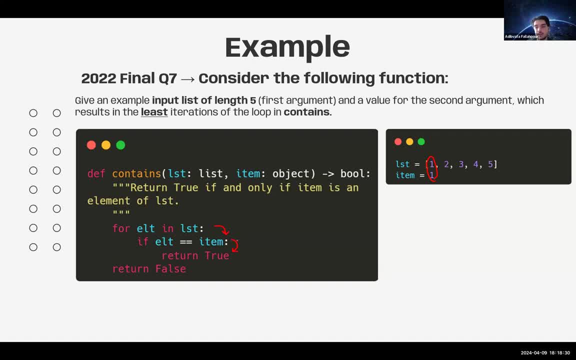 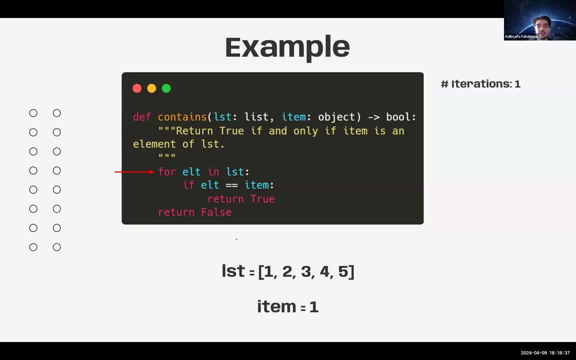 Because we found the item And it will return true, And so the function is done. And here is a demonstration of the first iteration: You check if it is inside the list, It is. So return true And done One iteration, And this is an example we went through. So this 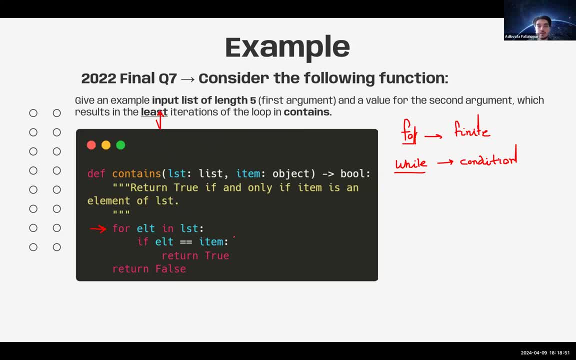 is a pretty easy example, but you can find harder types of questions with the same idea. And please practice, Find being able to trace through a program without actually running it And just look for it. So if you are going through it in your brain, it is important Whether you are checking. 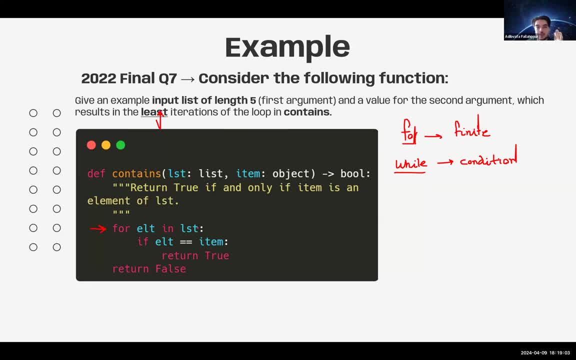 your code, whether you are trying to understand how many iterations it will have, etc. all of them together will define your skill as a programmer to be able to think before writing a code. Someone asked if this is an empty list. there will be no iterations, right? So, for example, 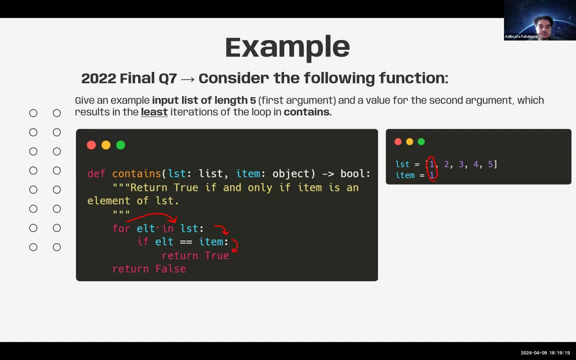 if you are saying for any item in an empty list, it could get tricky. I don't remember if it gives you an error because you don't have anything in the list or it won't run. I don't remember on the top of my head which one occurs, But yeah, if this is running. 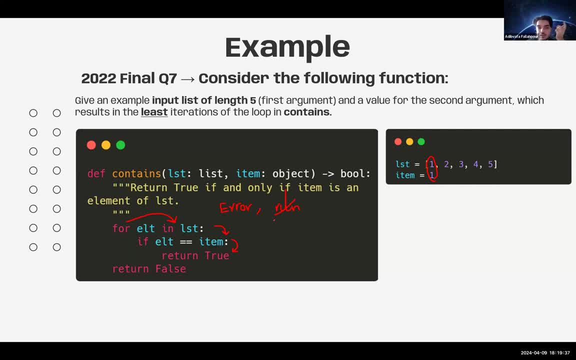 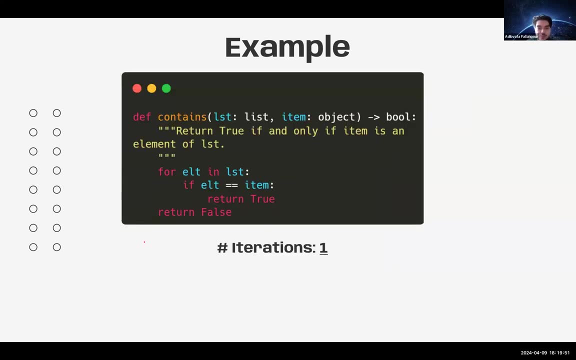 it will skip the form, But I think it will give you an error because there's nothing in the list. Oh, it satisfies. Okay, that's good. So it will just finish in the first row, All right, Moving on Here. So this is the same function we've been seeing before. So it is going to. 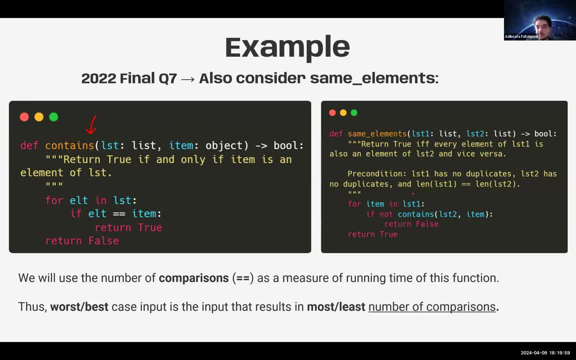 give me an error. This is going to give me an error And if you are going to get an error, the contains function and bring the chat lower so I can see. and I have a second function called sameElements, and this function gets two lists, list one and list two, and for each item in the list one, 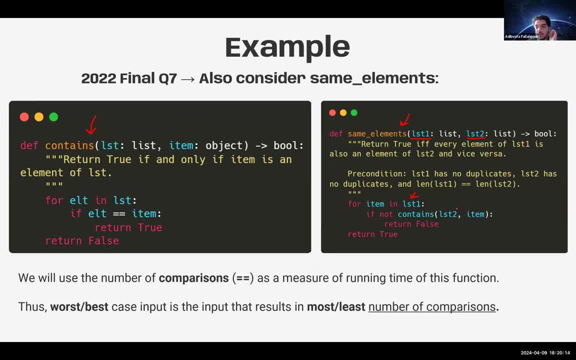 it will check if that item is inside list two. it does not find any item. so you know, if it sees that that item is not inside list two, the moment that happens it will return false. and the reason for that is: even if one of the items is not matching, then they do not have the same elements, right? 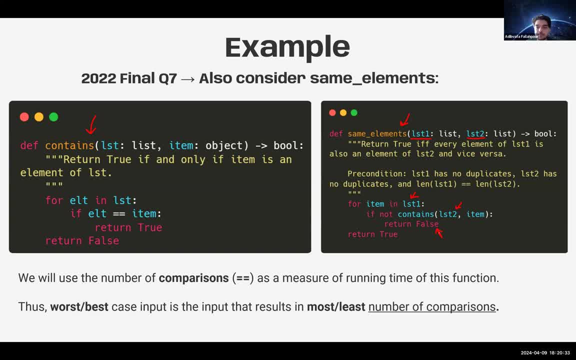 there's at least one item that's not in the list two. so you're done. otherwise, we'll just keep checking all the items and once it reaches a point that all the items in list one have been checked and all of them are contained in list two, then you just return true, every item in this one is. 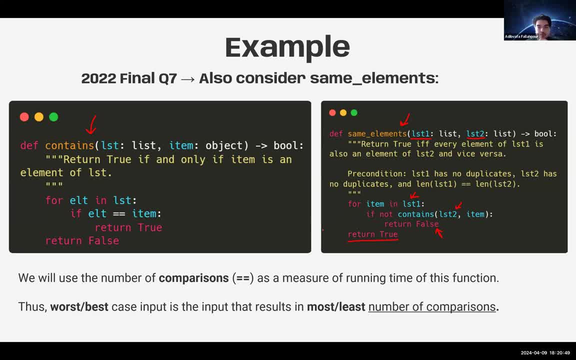 inside list. so I'm going to ask a random quick question from you guys. let's say, let's say, let's say have list1 equal to 1 and 2, and list2 equal to 3,, 2, and 1.. Now these two lists are not equal. 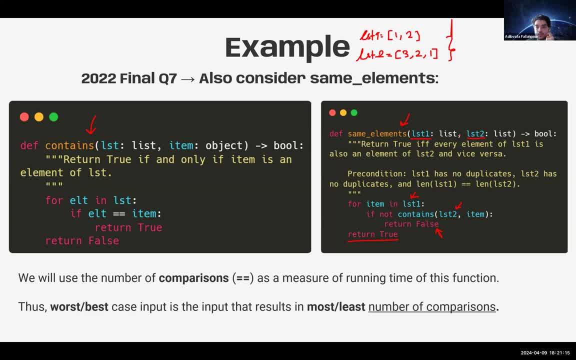 If I call same elements on list1 and list2, do I get true or do I get false? It's false, true, false. Which one should I believe? So you can trace through the program. right, You're going through each item of list1.. 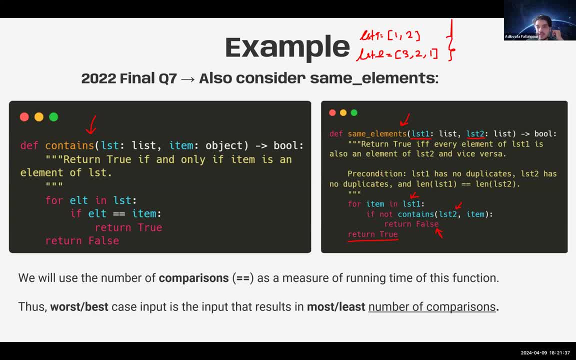 Yeah, that does. Well, you could argue that there's no precondition. Let's ignore precondition for now. That's all. Let's assume there's no precondition And you're running this. Do we get true or do we get false? 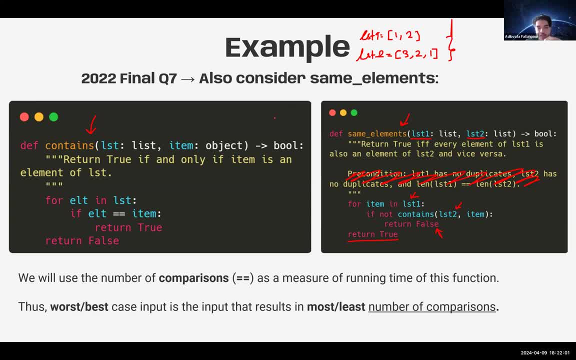 Your list1 is number 1 and 2.. Exactly, That's true. Why? Because we'll check item1.. Item1 is inside list2.. We'll check item2.. Item2 is inside list2.. So you're done. You've returned true. 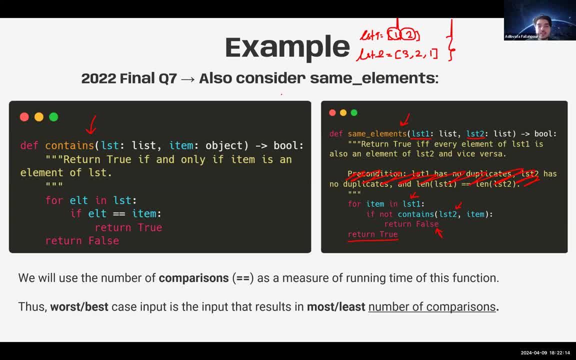 So same elements is only checking if list1 is a subset of list2, not if it's equal. That's why we add a condition here that their length should be equal to. Now, since their length should definitely be equal to, we cannot have list2 being larger than. 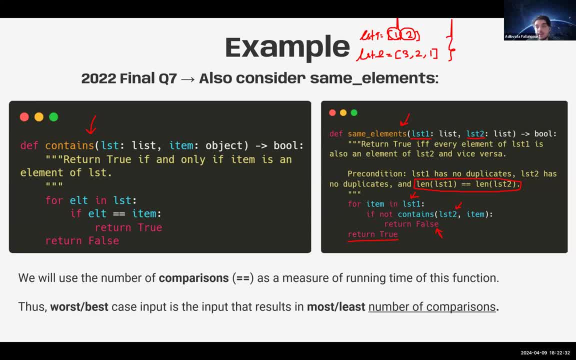 list1.. In other words, this will not be a valid example And if you want to make it valid, you have to get rid of tree And, as a result, now same elements is in fact checking for the fact that these two lists are equal. So you can see that our function is not defined like that. With a 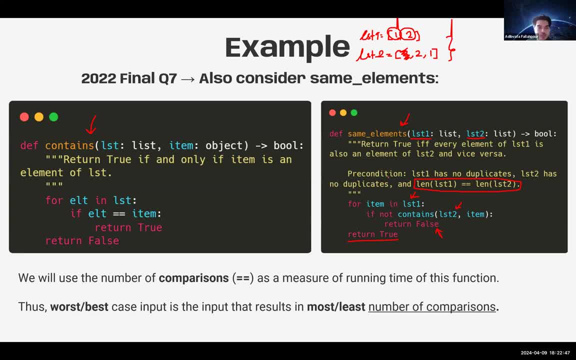 precondition we are able to satisfy the property. Well, anyways, that was just a quick example. So, as you saw, we used the comparison operator as a way to understand. if you know, the length is equal here And the worst case and best case. 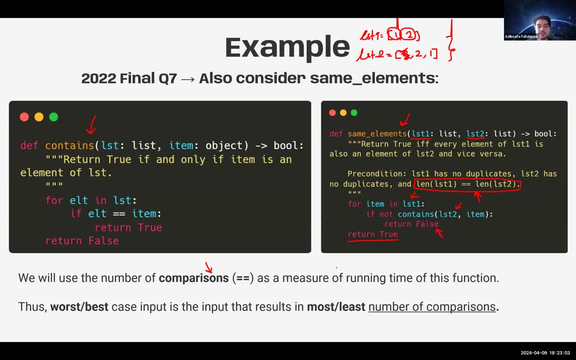 is. you know, if you think about it, the best case is the one that you quickly exit. The worst case is the one that you just keep going through the forward, And that's how you can find your most and least number of comparisons. Now the question is here: given links1,, 2, and 3,. 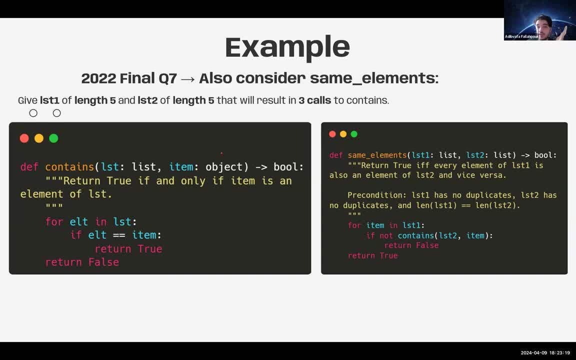 the question is here: given links1, length5, links2, length5, so the length is matching- what will result in tree calls in the content- And there are a lot of examples for this one, but the key idea is, if you just want to make three calls, you want the first two calls. 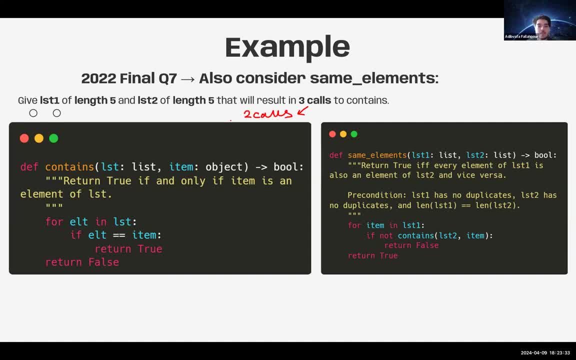 the first two items that you'reassadors that you're checking, to say yes, I'm contained. In other words, you want these two ones to be contained and your third call, the last call. you do not want the third call or the third item to be in the list. 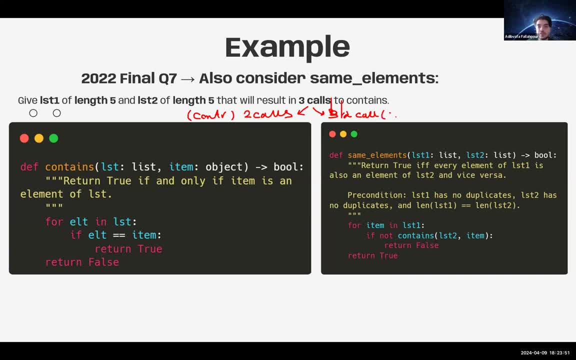 because you want to exit. so the third one is: is not in the list. what you want to visualize it here is list one, list two: this one's first item is in the list. this one second item is also there, but the third item is not. as a result, you will run this. 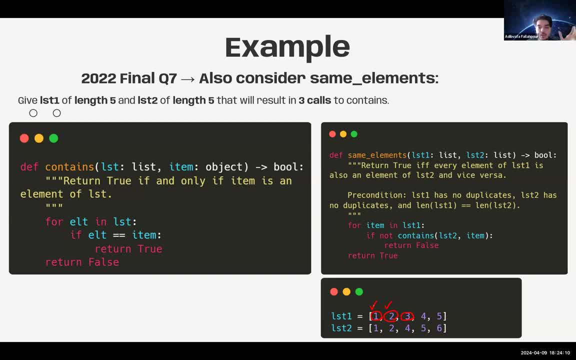 okay, next iteration, you will also run this. okay, next iteration and you will run this one. but it will fail and you return false again. so you went through the loop three times and, as a result, you satisfy three calls to your contains function. exactly the order of items in list two doesn't matter because 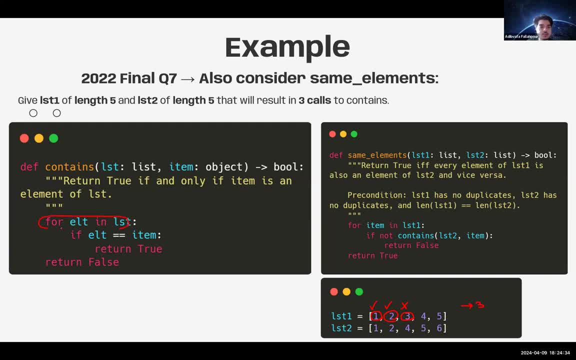 contains is checking for all the elements right? what, what contains? does it exactly? the order of items in list two doesn't matter, because the order of items in list two doesn't matter because goes through every single element of these two to see if it matches the current item at hand. 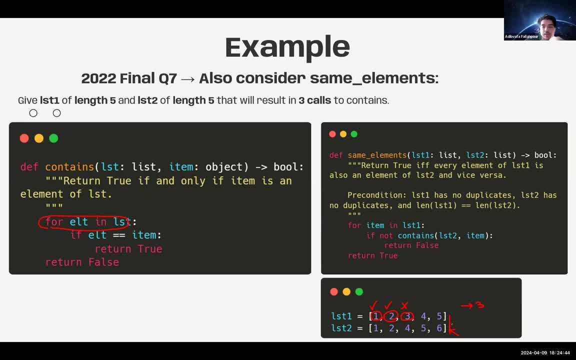 so the order doesn't matter. now it will probably affect the speed a bit, like here. it will be a bit faster because one is right in the beginning, two is also right in the beginning, so we quickly find this in these two and we're done. uh, if one and two are in the end of these, two will take a bit longer. 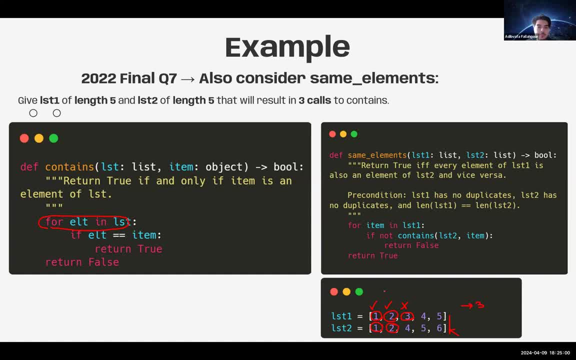 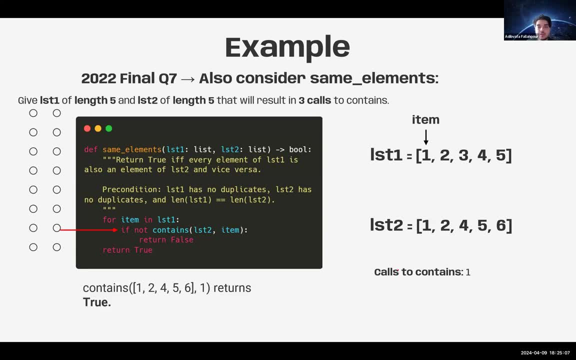 but the result is still the same. great question, let's move on um. this is just an example we went through again. item one checks it is. item two checks it's in. item three checks it's not in. so we return false and we run through the loop three times. so that's three. 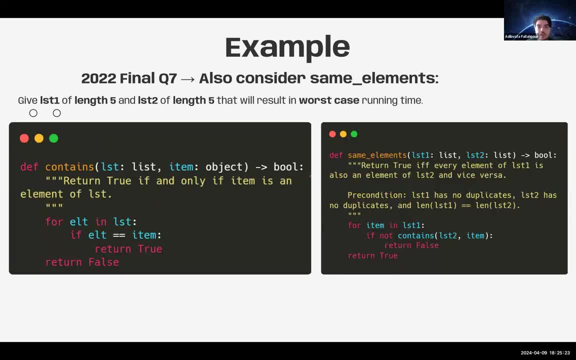 now we can again play with the same idea, right, you have this one length five, this two length five, and now we're going to have a worst case product. do you guys have any suggestions? same function, but new in new inputs, such that we will have the worst case right. 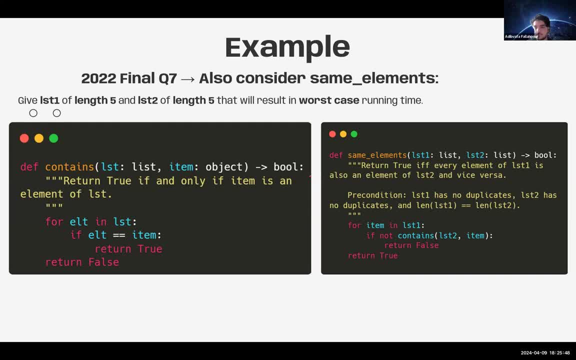 uh, they're opposite order to each other. but you, yeah, that's, that should work. yeah, that works, but like the order doesn't really matter. like like i guess, um, like your example will work, you and make YouTube headsets better, too famous, but the order doesn't. 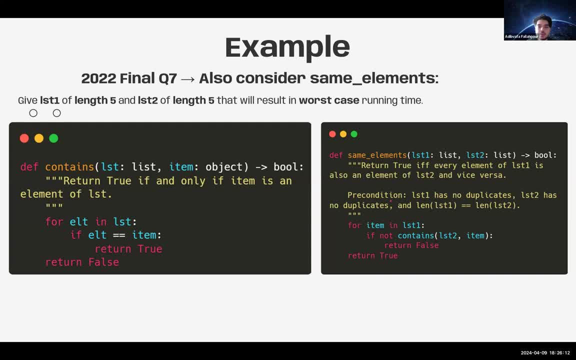 work exactly. so there are two scenarios either. um the wan- yes, it will return- was submitted. there are two scenarios. one of them is, as one of your id to is meaningful, different than the other your friends mentioned. the lists are equal, like you don't even need to change the order. 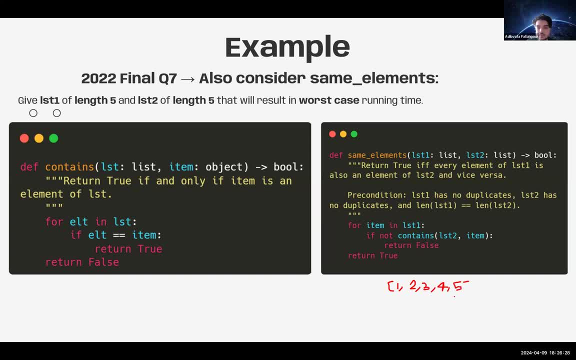 let's say list one is one, two, three, four, five. this is lst one. lst2 is again one, two, three, four, five. no need to change any order. what happens is your function is trying to see if all the elements of list one are inside list two, so it has to run for all of them until one of them fails, but here none. 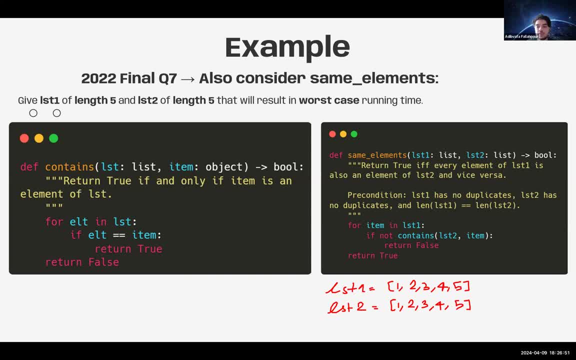 of the numbers will fail. all of them will be. yeah, i mean here, they're good. to the next one, go to the next one. so we'll run for one, it will run for two, for three, for four, for five, and then it will return. true, in the end. that's one approach. the second approach is, as one of you guys mentioned in. 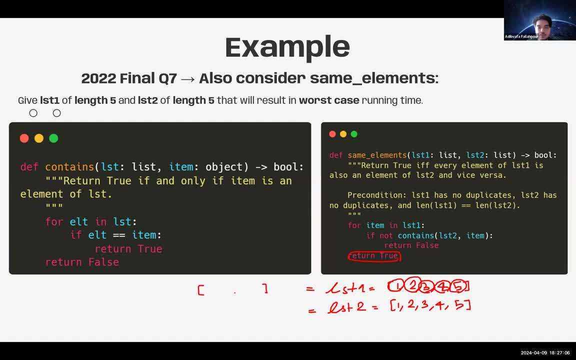 private- is ignoring the last one. in other words, we have the same thing- one, two, three, four- but let's say here we have 10 and list two is again one, two, three, five. this will also work well because the first four elements that we are checking in list one are all included in these two. so we'll 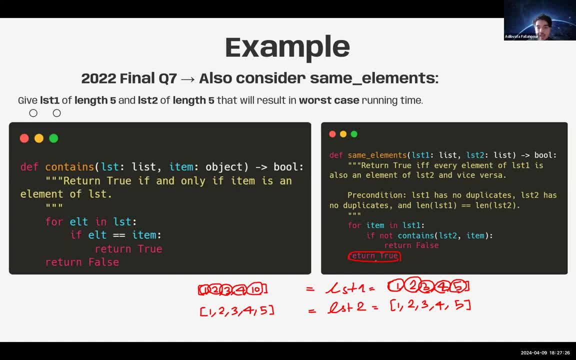 run four times and once we reach 10 we'll also run again, and in that scenario we just return false, but we still go through the fifth iteration because you have to check number 10. so both of these approaches will run five times. the key here is the first four elements should be: 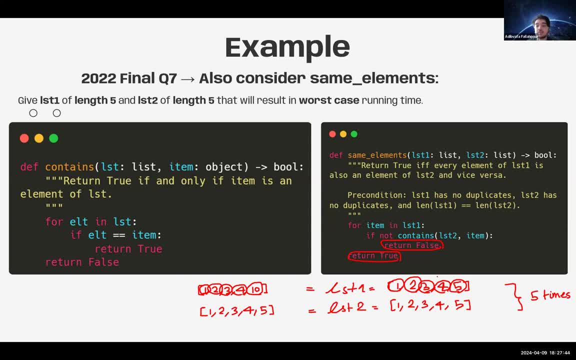 the same. or let's say this way: the first four elements of list one should be inside list two. it doesn't. it doesn't matter where they are located in list two, as long as they are there, and we keep going. but the last element of this one could be anything, it won't matter, it just. 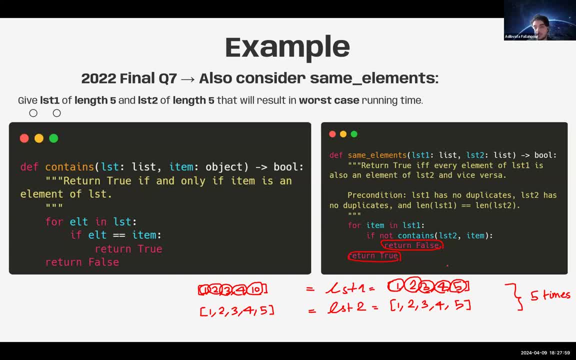 affects the output. but the worst case- running time- stays the same. now, if you really really want to make it the worst case, you can run it five times and run it four times, and run it five times, and run it five times and then, yeah, as your friend mentioned, you want to change the orders. 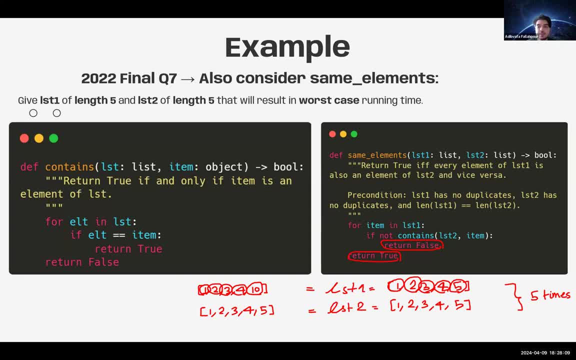 like you know, if you want to put one in the end, like, do nasty things to make it last longer, but in the end of the day, the number of iterations is usually the most important thing, right? yes, the function will return for us immediately once it finds an element in. 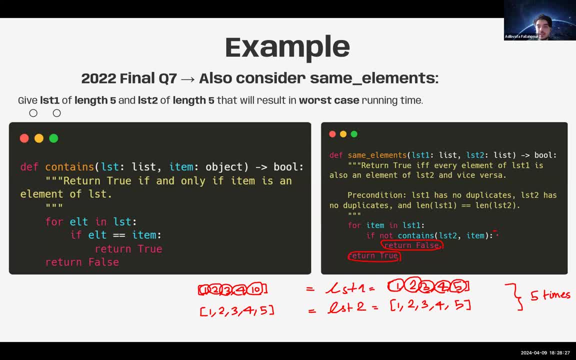 list one that's not in list two, because that will not satisfy contains. so if not, contains will be satisfied, and so you'll return false and once you return and the function is done, we'll go to sleep. okay, are we all on the same page? has anyone went to the meditation rooms? no, okay, that's good. 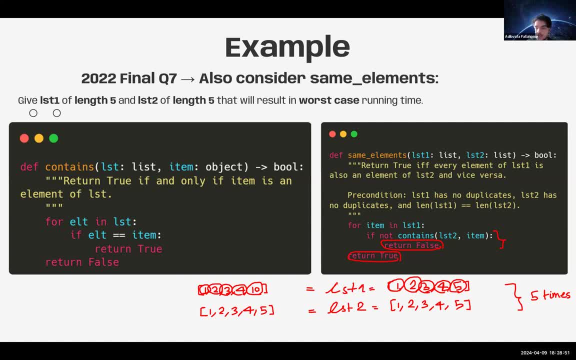 right, do you guys want to move forward? am i too slow, too fast? can you guys hear me? am i muted? one one: okay, good speed, nice, good speed with the like: okay, let's go. yes, that's. i love that enthusiasm, and this is an example here we just went through. now, just to wrap it this up: if you want to have, 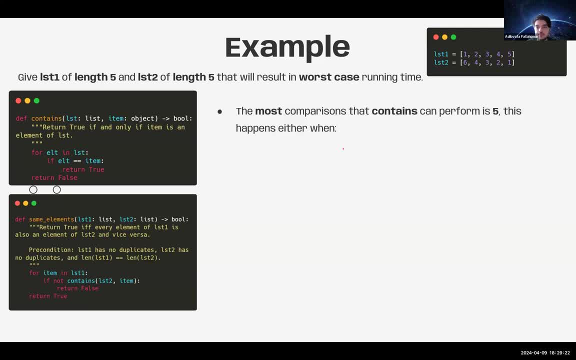 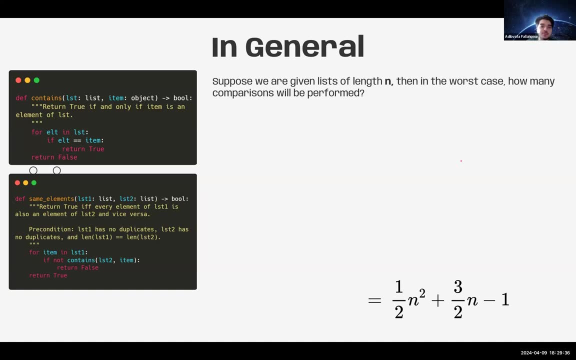 the worst case, running time. all you'll do is, you know, what matters is the first four. so either lsd does not contain the item in the end or it just has it, as the last element does not matter, and that's how you keep going. so, in general, uh, if you want to put it with some math, which is 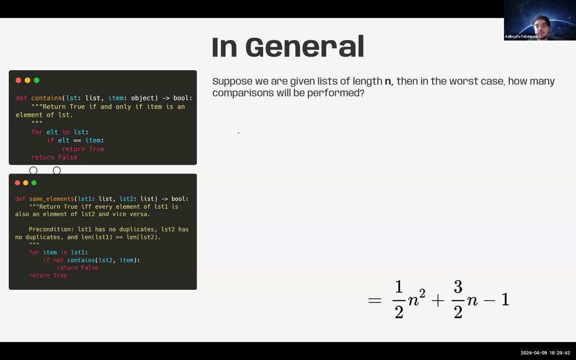 kind of funny. if you have two lists of length n, then in the worst case, how many comparisons will you do? so in the worst case, what you'll end up doing is for for any element in list one, you have to check all the elements in list two, right? so in other words, 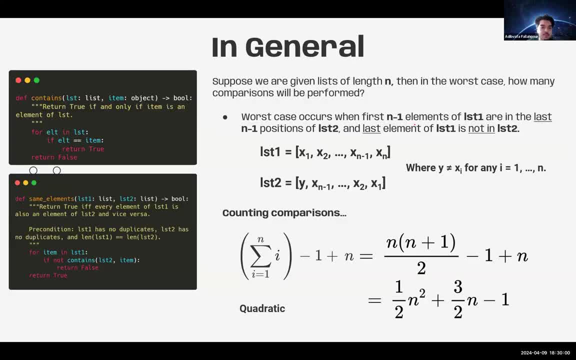 um, oh, there's a lot of math here. uh, let me first just give you the intuition: like nothing here matters. the only thing that really matters is n squared. i want you guys to just think about the idea that if you have list one here, let's say your list one. i'm going to show it as a line, right? 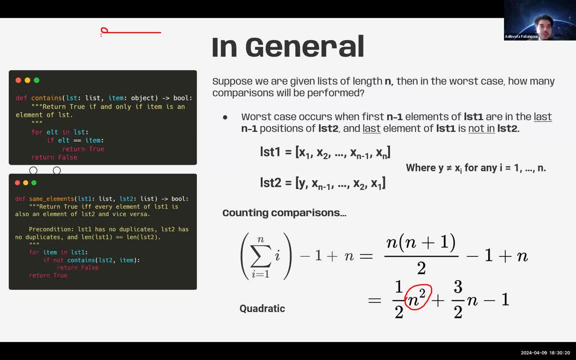 for any element of list one, you have to check it in list two. so if this is lsd1 and this is lsd2, for any element of LST1, you have to check: is it this one in LST2?? Is it that one? Is it this one? Is it? 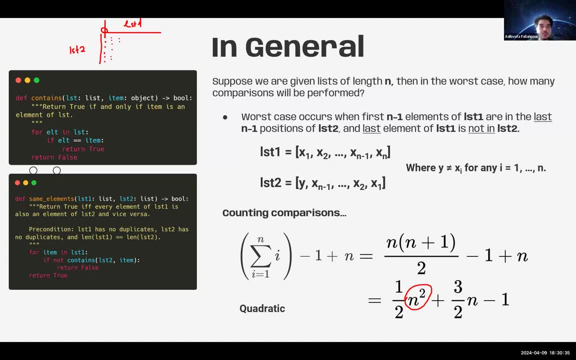 this one? Is it this one? No, no, You just keep going right. So if you think about it, if LST1 has n elements and LST2 has also n elements, you're going to have a general comparison to the. 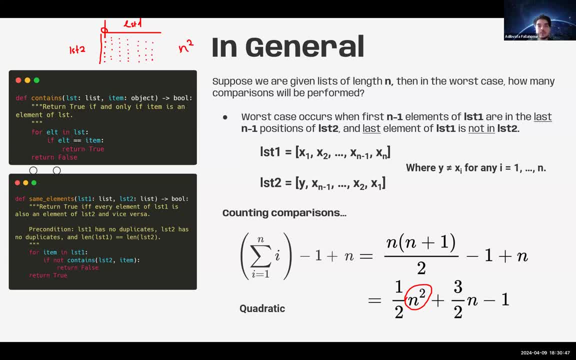 power to the order of n squared. right, Because for any element in LST1, you're going to compare to all elements in LST2.. So you have n elements times n elements, which gives you n squared, And that's all that matters, Because in the end of the day, is it 1n squared, Is it 2n squared? 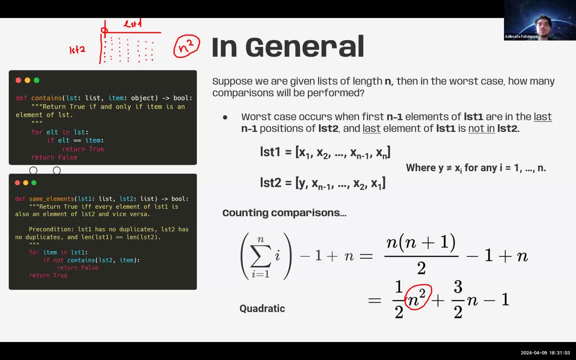 It doesn't matter. n squared is the big factor. Like if n is in the order of millions, n squared is much bigger than n or anything else. Now how do we calculate it exactly? is the next: Does everyone okay on the intuition of why it's around n squared? 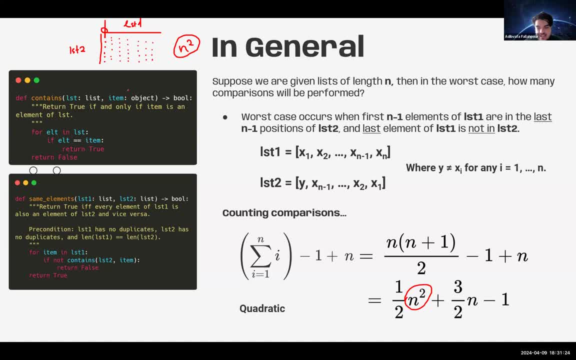 Awesome. Now, if you remember, one of your friends mentioned something nasty, which is: we don't want the function to be done quickly, right? We want the first element that LST1 is checking to be like in the end, right? So it takes a lot of time to go through these one by. 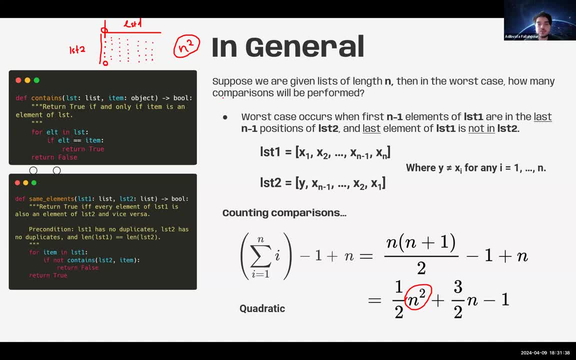 one. In other words, what we want to do is we want to have them to have reverse order. So the first item of LST1 should be the n of LST2.. So we do a lot of comparisons. The second one should be: 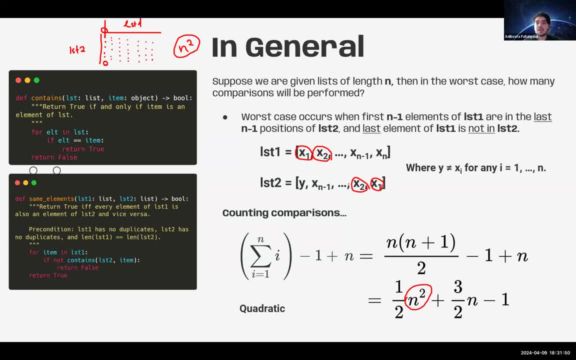 again pretty close to the n. So we do a lot of comparisons Now. this will squeeze in a bit more, you know time, because the model has to go through more checks and checks, So that will result in you having more checks compared. 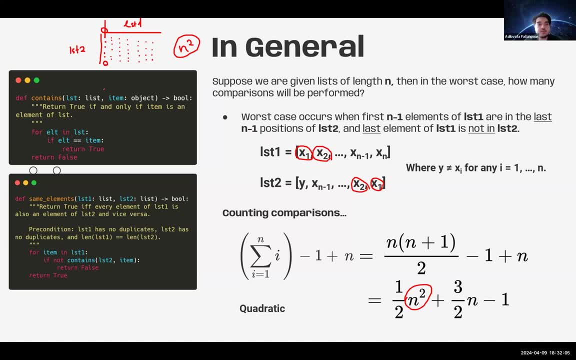 to just n squared. Now how do we get n squared again? If you remember what the function is doing is for any element in LST1, it's checking it over all the elements in LST2.. For example, if you're at x1, it's going to say: is x1 the first element? No, Is it the second element? No. 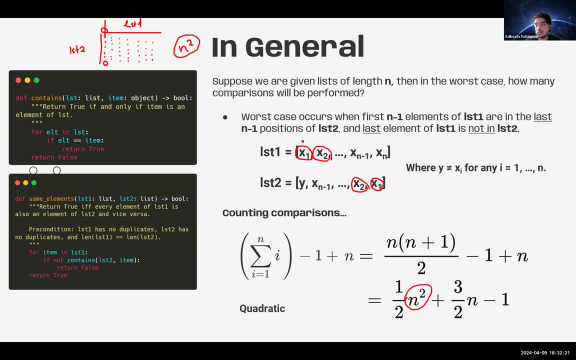 Is it the third one, And so on. So it's going to check it n times. And the same thing for x2 and x1. So since for any number in LST1, you're checking it, for any number in LST2, you have an. 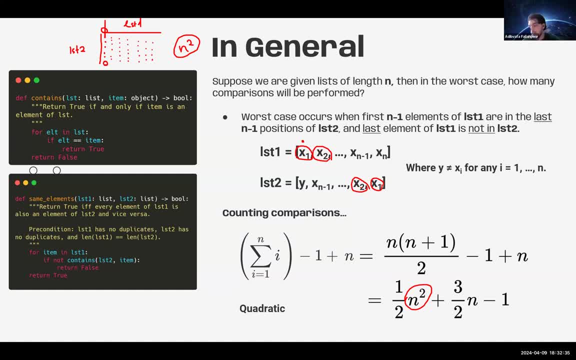 order of n squared. Now, this is not exactly n squared, And the reason for that is, for example, some element in the middle. if it also exists in the middle of LST2, you don't need to check all the elements, because the moment you reach here, you're done. You know that the element 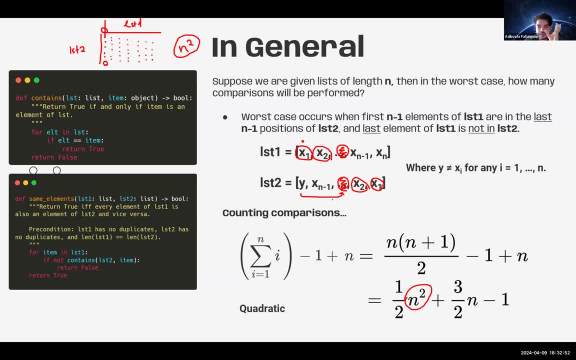 exists in place two. So if you think about it on average, you're not going to check for all the n elements. It's going to be some portion of those n elements And that's why it's not n squared, It's half of n squared, But the intuition that it's about n squared is more. 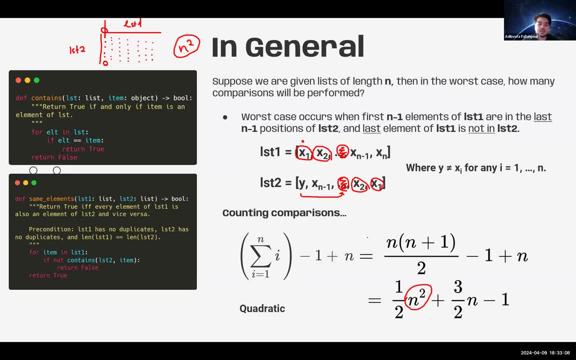 important. Now, how do we count the exact number of comparisons in the scenario that LST1 and LST2 are the same list, just in reverse orders? It's pretty easy How? Let's just do it by normal count For x1,. you're going to do n comparisons, right? You're going to check the. 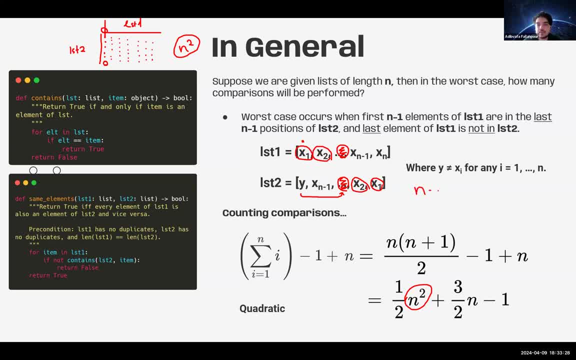 first element, second element, all the way in the end. So you have n For x2, you're going to do the same thing, But the moment you reach x2 here you're done. In other words, you're going to have: 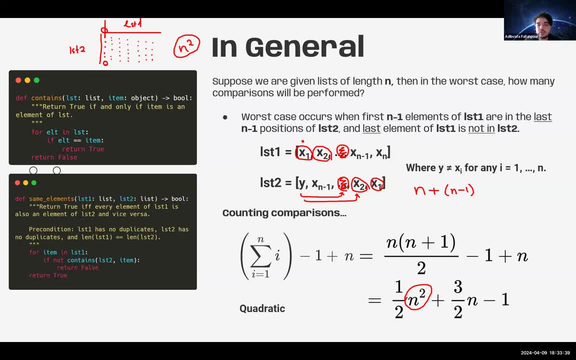 only n minus 1 checks, because you never reach the last element. And if you follow the same order, then you'll see that this next one will only be checked for n minus 2 times, And this will keep going until the last element. 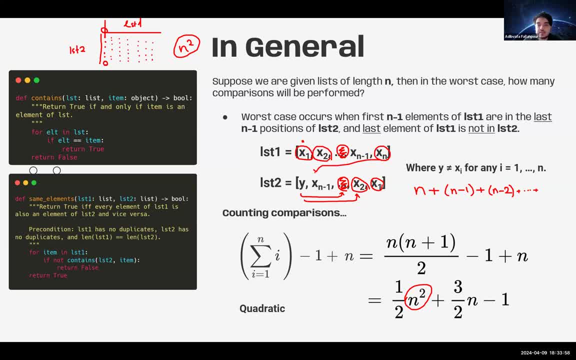 element is xn, right? xn is not in the list. So you have to keep checking as we go. Remember, if xn is not in the list, you will check the first one no. second one, no. third one: no. 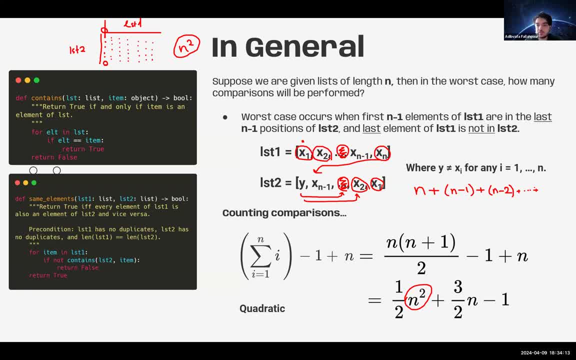 you'll keep going. So if I do the last one, if you think about it you might say: oh, if xn was in the beginning of LST2, then I just needed one check. But we could do a trick here, We could put: 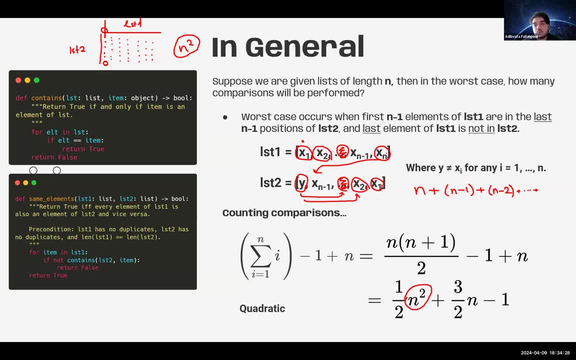 as an element that's not in LST2.. And the reason we can do that is because this is the last one right. It doesn't matter if this is inside LST1 or not inside LST2, we are done. We are done with. 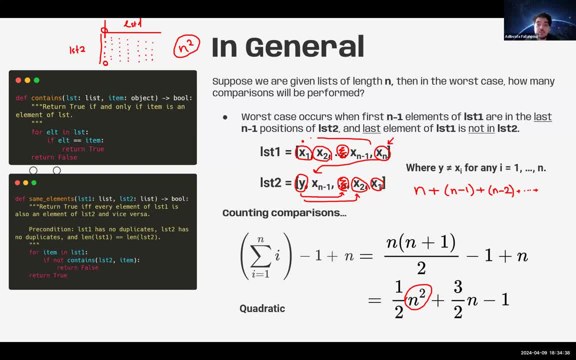 the function. We need any element prior to xn to be in LST2 to ensure that the function will keep running. But the last one is not important. So 1 minus last one, the xn minus 1, will be having two comparisons And instead of reaching 1, we suddenly reach n. 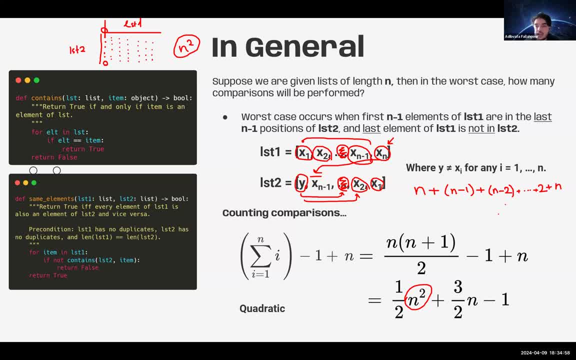 Because we could change this pattern for the last one, And if you keep counting these, you'll reach what it is in the bottom. You will have n times n plus 1 over 2, minus 1 plus n. If you sum these. 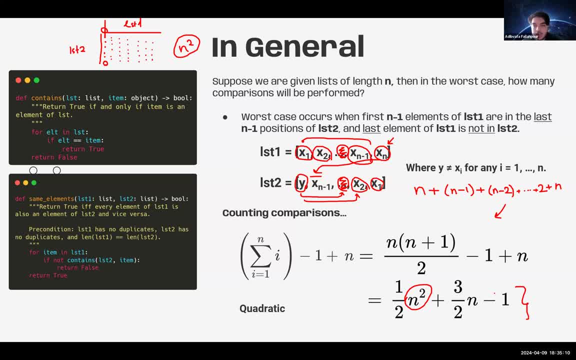 up. you get this as a math, which will be then this. Now, this example is, you know, a nice generalization of what we went through. right, We started from contains, we also went through same elements and we did a lot of good progress. 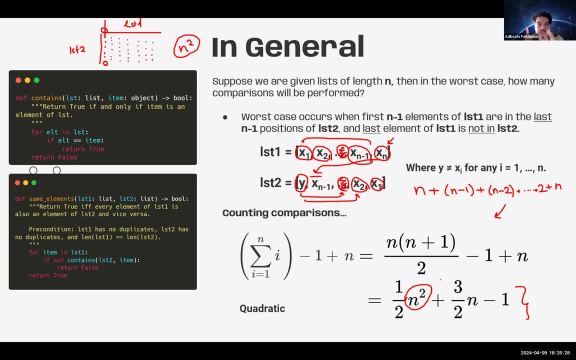 Through these functions And I'm now sure you guys have a better sense of how you can trace through these different small mini functions and understand their worst case and their best case scenarios, along with also counting the exact number of comparisons. Is everyone clear on this? 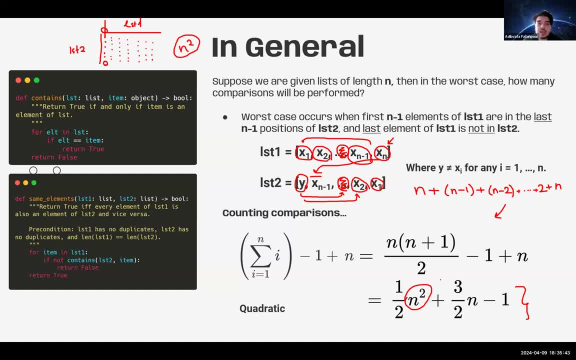 one. Everything good. It depends. If in the exam they ask you what is the order Like, what is the general idea, What is the pattern, Then it's in order of n squared, because that's the most important part of this. 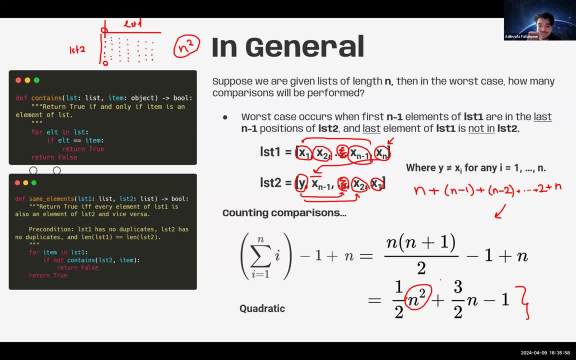 mathematical state. But if they say no, write the exact number of comparisons. then you have to do what I've done here. No, no, this is not a proof at all, Like this is just counting, right, Like we're doing counting, but we're doing it in a really, you know, fashioned way to make our job. 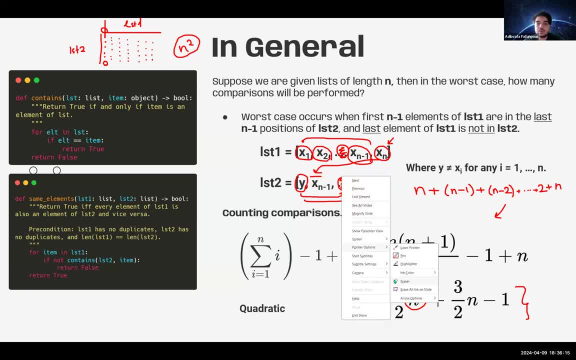 easier. If you think about it. the only thing we're really doing is just tracing through our program. Yeah, you're just saying: hey, let's start from x1.. Okay, I'll check you n times. So this is n for x2.. 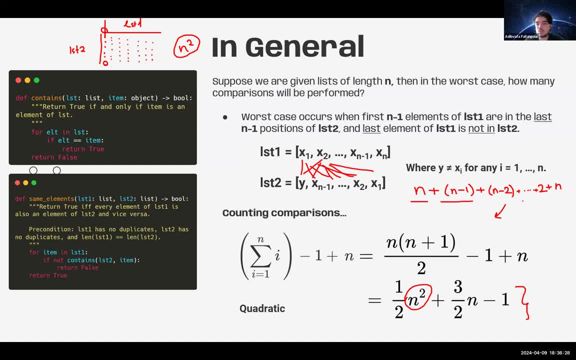 I'm going to check you n minus 1 times, and so on and so forth until you reach 2.. And for the last one I have to check all of them, because it's not inside this 2, so it becomes n. That's how it goes. 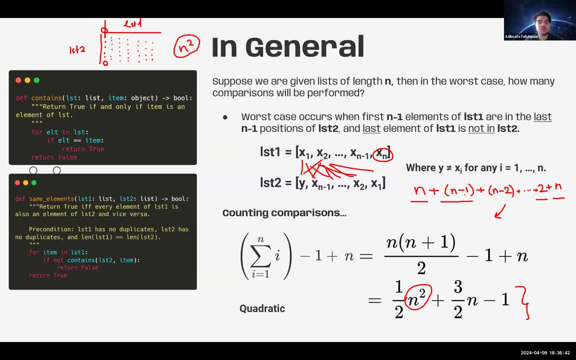 It's not really a proof. Rather, I think let's think of it as just counting. but you're counting, you know really. good order to make your job easier. Everyone good on the same page. Yeah, Good, The last one would be 1 if xn was the first element. So if, instead of having y in less, 2,. 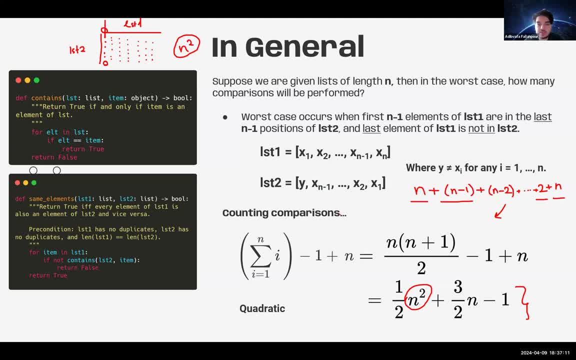 you had xn, Like if these two were the exact opposite. instead of having y, you had like xn here. And then, yes, instead of n times, we'll just check xn once and boom, it's here. 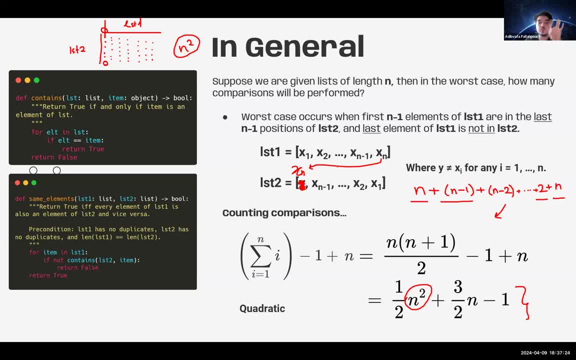 And so, in order to make it really, really worse, we are just going to exclude xn from these two. We're just going to have something else, like y or whatever, such that we have to count n times rather than 1 time. But that's just a small part of it, Like. 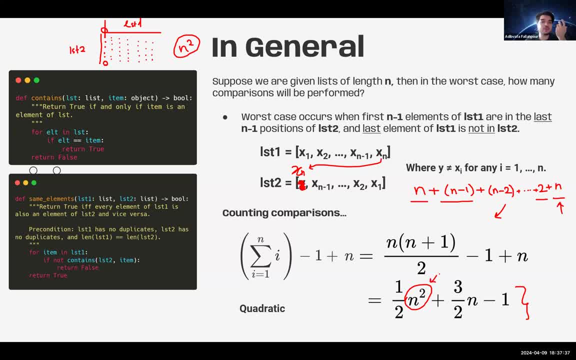 the main idea is this: n squared. Well, because this will get repeated over and over And if you're really curious to see where does n squared come in, if you think about it, here we have for loop, and this is running contains which is defined using another for loop. 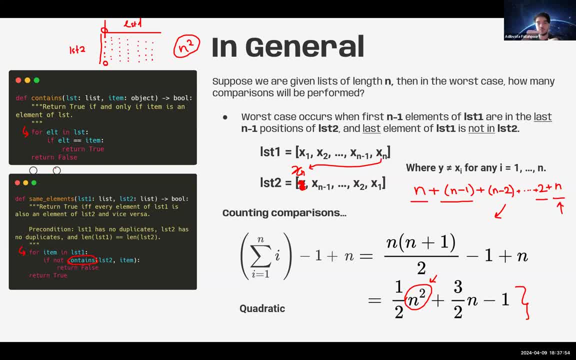 So, even though it's separate, we have a nested for loop, So a for loop inside a for loop, And each of them are running for about n elements, maybe lower on average, since you could finish quickly, But you know on average. 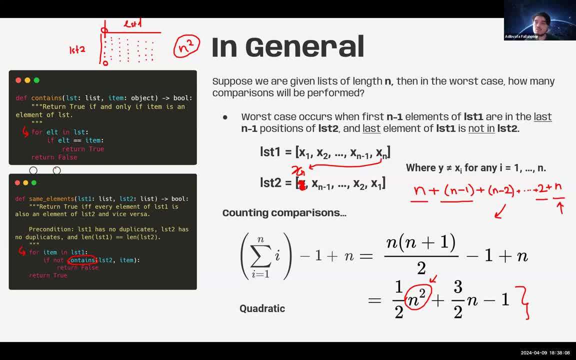 n is n, so two ns being multiplied gives you n squared, And that's the type of order we're talking about. So if you see nested for loops, most of the time it's going to be multiplying your lengths and increasing the order to quadratic, to cubic, et cetera. But don't be fooled. 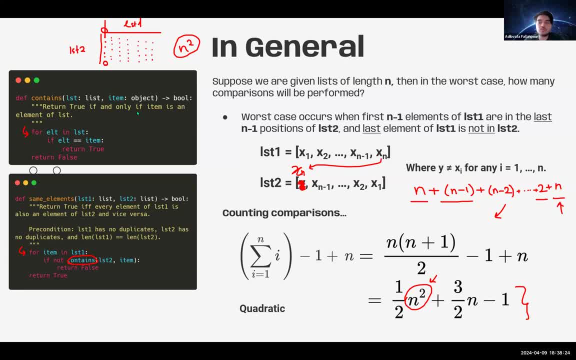 Sometimes a for loop might just run for 5n times And if you're really curious to see where this is going to come in, it's going to be 5 times always. It doesn't really matter if you increase the length or not, So it depends on your example. 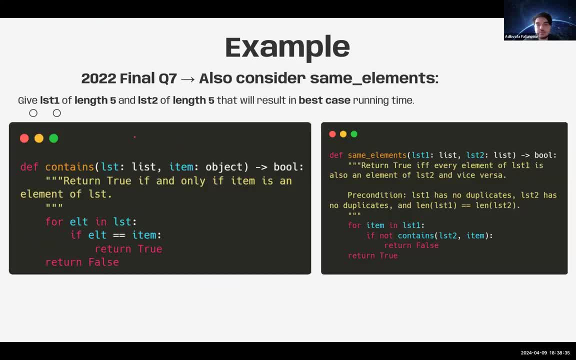 Already moving on. so this was the example we talked about. And just to wrap it up, what is the best case? We've already talked about it. The best case is in which the first element does not exist. right, Because that's the first element we check. We do not have it contained, so we return. 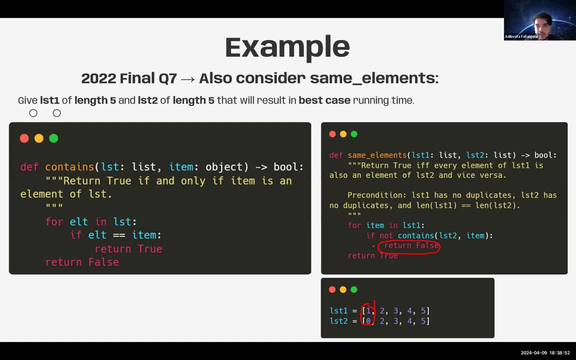 false and we're done. Yes, this function needs length To be equal to, Because if you think about it, you know if length of LST2 is bigger than LST1, then you have to do more comparisons if your items are in the end of LST2.. So you could just 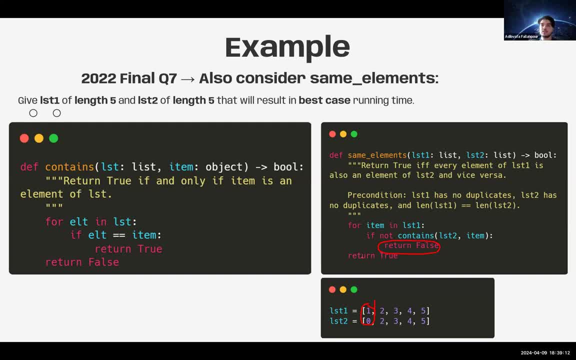 make everything worse and worse as you go. So it could be a good practice to see if your length of LST2 is m and length of LST1 is n. what is the order? But that's going to be a bit challenging. 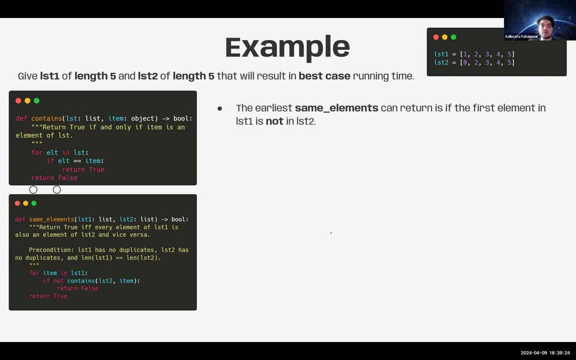 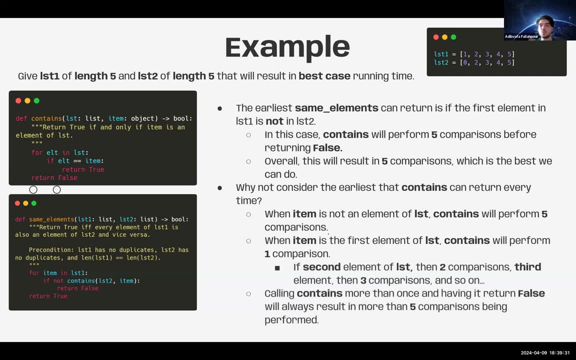 Anyway. so the best case, running time is easy. The first item: it's not in the list, so we just return false and we're done. Right, You just do one for loop, one iteration, one if statement and we're done. 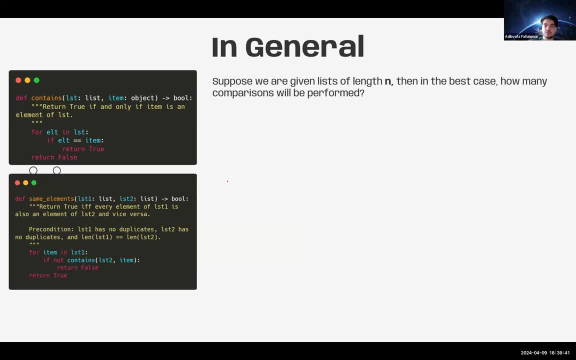 Now the generalization of the best case is interesting. So what is your answer, guys? If you are given lists of length n, like they're both the same length and they're both length n, what is the number of comparisons we'll do in the best case? 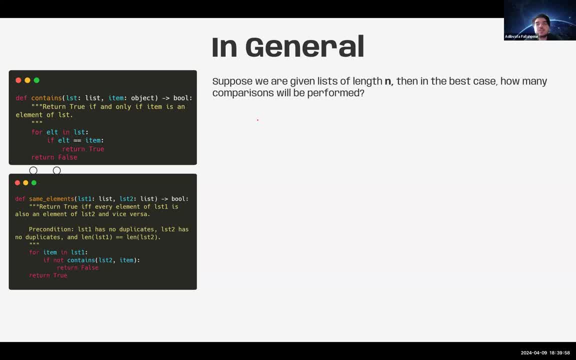 What is like the exact number? What is the order? Is it n? squared n. cubed. order of n. What could it be? I'm going to see a couple answers before I disclose it, But really careful, right. 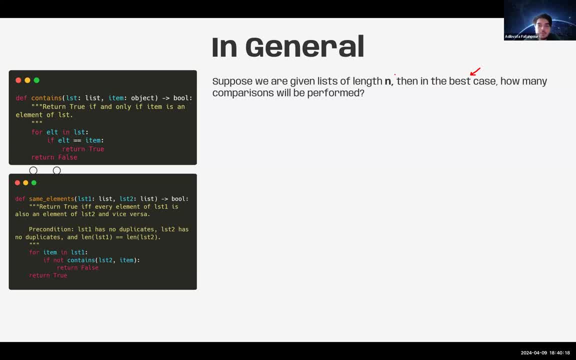 We're in the best case, which means we want to exit as soon as possible. Both are going to be length 1.. Okay, one person says constant. one person says order of n. The third person will close the deal. What Exactly? So the best case occurs when the first element is not in list 2, which means 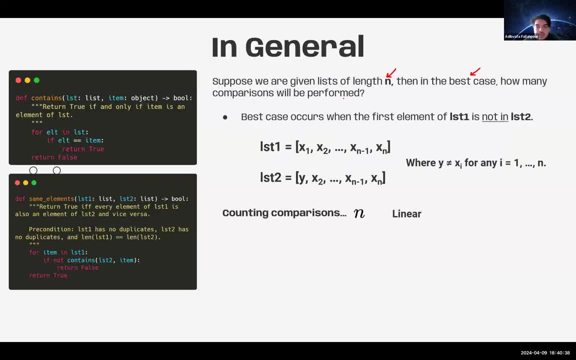 it's just 1, right, It's linear. Now again, this is n. I'm going to explain why this is n, But the best case is just 1.. Your first element is not here, so you're just going to keep checking. 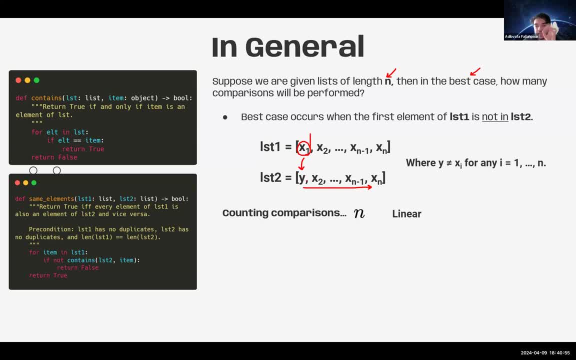 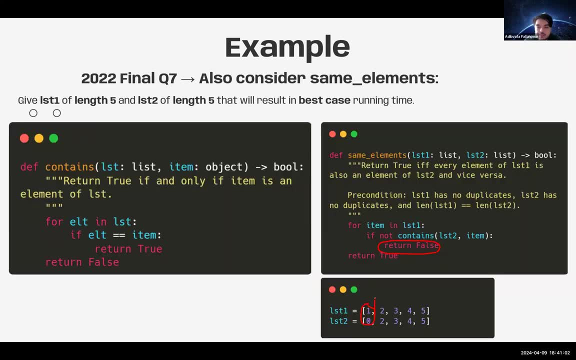 Now, something that's tricky here, that you guys say want, is the difference of this example with the previous one. Because if you think about it in the previous one, what happens is you're going to keep number 1.. You're going to see, the first element is 0.. 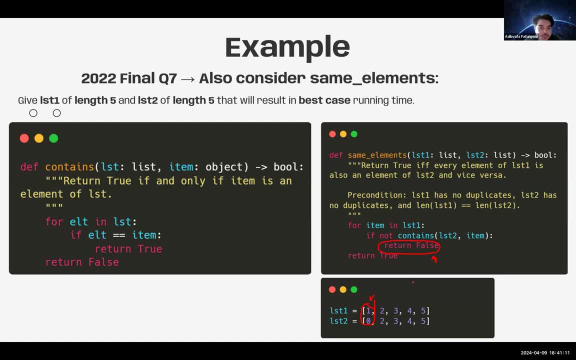 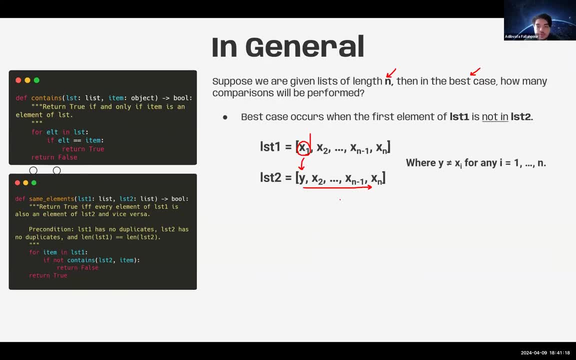 So it's not contained and you're going to return false right, And that's one of the reasons this is going to be constant. So again, just to summarize it, what happens is you know you're going to apply an x1.. 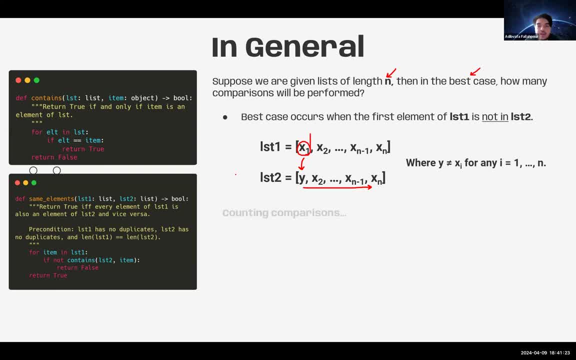 You're going to check, x1 is not in y, So these two cannot have the same element And this will be 1.. Okay, sounds good. This is a typo. No, yours truly, This is 1.. Okay, I hope the example is understood by everyone. This is a pretty fun exercise to do. 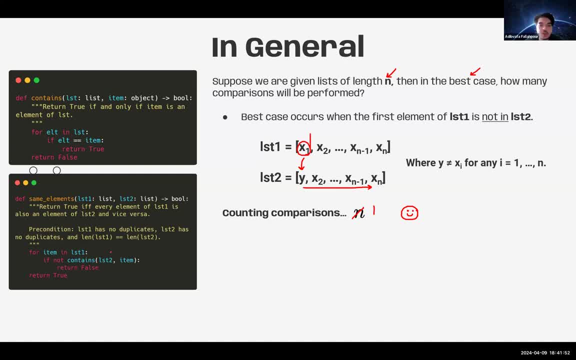 So the thing is, the first element is not contained in list 2, right. So the first element is not contained in list 2, right. So the first element is not contained in list 2, right. So the first element is not contained in list 2, right. 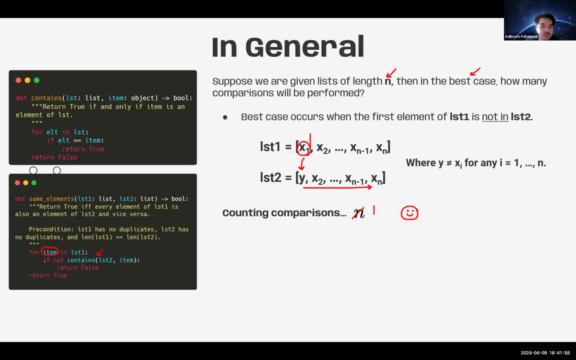 element we find in this for loop. this is not contained And so this is non-contained, which means these two lists could not have the same elements anymore. If the first one is not contained, then we just have to return false right Now. I guess the reason for this confusion. 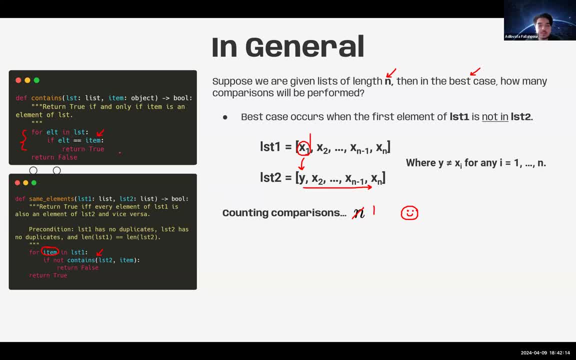 is the way we've defined. contains is checking through all the elements, right? So I suppose, yes, this should be n Check it. Let me see, because the confusion comes from these. Yeah, so the number of comparisons for list 1 will be 1,. 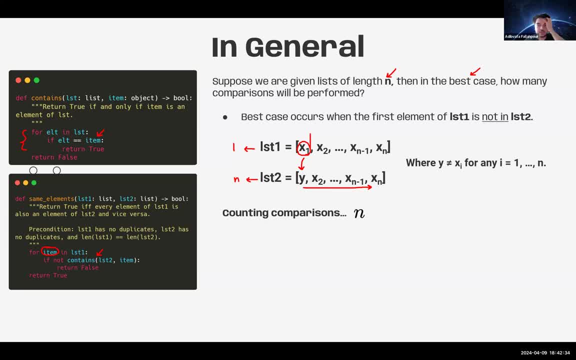 and for list 2 will be n, because now this will clear, right? So for the first element of list 1, you're gonna keep checking through all the elements in list 2 because it does not exist. then you're gonna return false. So if you're looking for the 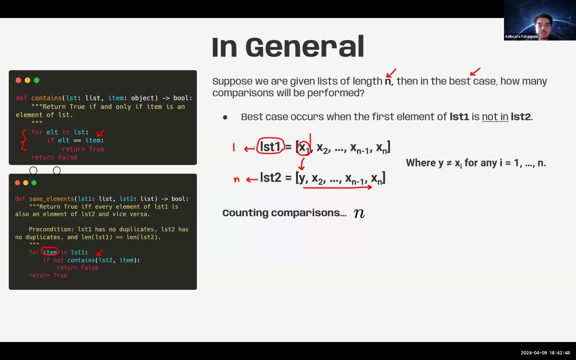 complexity in terms of Swift. you can do that and I'm gonna return false. I'm gonna return false and then I'm going to return false. So, if you're looking for the complexity in terms of how many comparisons we're going to have for this, one element should be for list, two will be n. 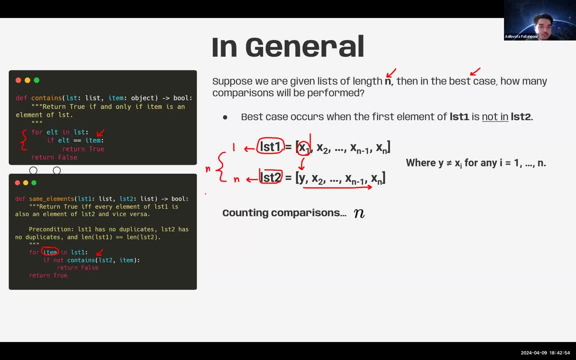 but i assume overall you have to multiply so you get n back. does it make sense? so it's more about how you formulate the question right, like if your formulation is how many elements of list one will we go through, then it's one always. how many elements of this two will we go through? it's going to be n. so overall you're going to have an n by 1. 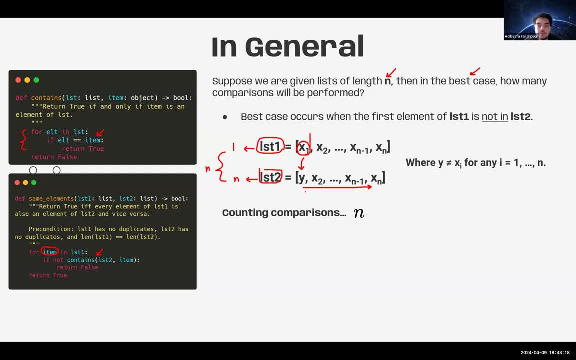 multiplication, so you have n comparisons and then your order will also be n, which is not constant, which is going to be lean. yeah, does it make sense? now? i also got confused. it's pretty fun, amazing. it's small, so let's do some smaller, easier multiple choice questions for iterations. 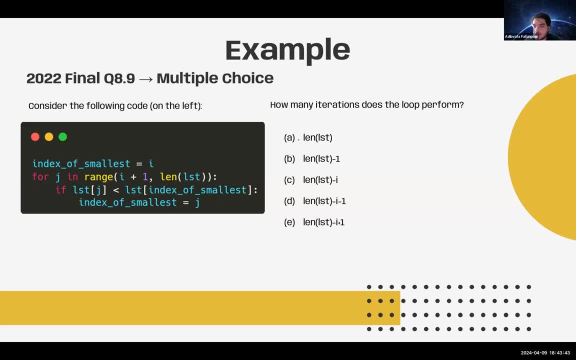 now this one is not that hard. i guess you guys can solve it with you. we have an index. we're going to set it to i for j in range i plus 1 to the end of list. we're going to do an if comparison is the jth element of list less than the basically the ith. 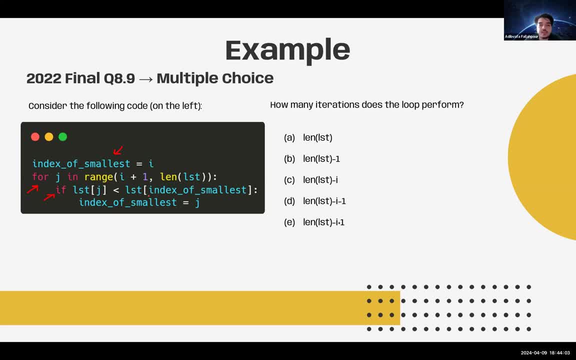 element of this. if that's so, the index of smallest will be j, which means we're going to update. right, we found a number that's smaller than i, so we're going to update our index string. so how many iterations do you provide for? and just for people who are a bit confused, let's say lst, like this list. 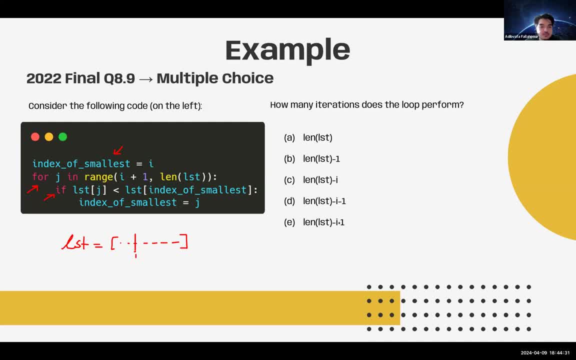 you know, has a bunch of elements. i is here and you're saying: for j in range i all the way in the length of list, if the lsd j, which means the jth element, is less than the ith element, update the index. so what is it going to be? 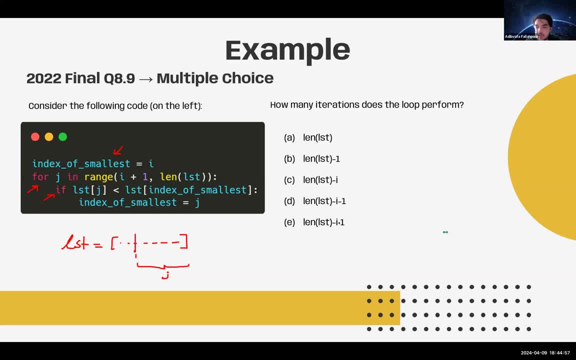 does anyone agree with, uh, the mentioned answer in the chat? okay, one person exactly. so i'm really happy that you guys understood that we have a for loop, right, so we don't really care what happens inside the for loop. we'll run for the set number of times we have. in other words, this whole thing is useless, like we don't care what's. 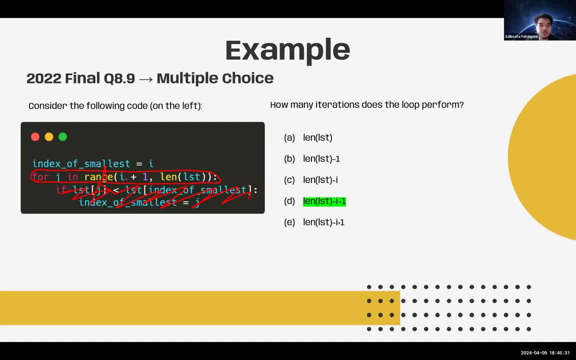 happening here and how many times that for loop will run. well, it starts from i plus one and it goes all the way to len. so it's len minus, i plus one, which will give you len minus, i minus, and that's answered. that's the function of the for loop. right? so for loop one is the function of the for loop. 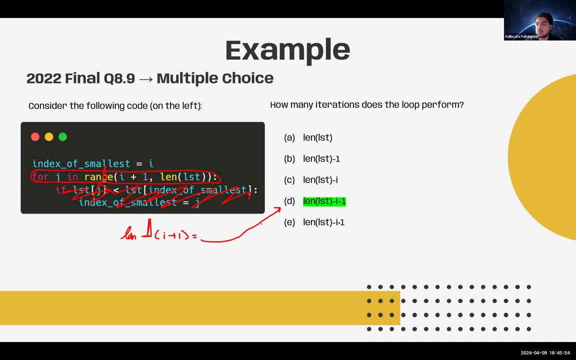 so you can just run for whatever number times it takes to be set. alright, we're done with the for loop. but you know, i'm a little bit ashamed of what i've said. i'm a little bit ashamed of running for a constant number of times. great happy you guys were able to solve this. must be tricky, but you get the right. the for loop will. 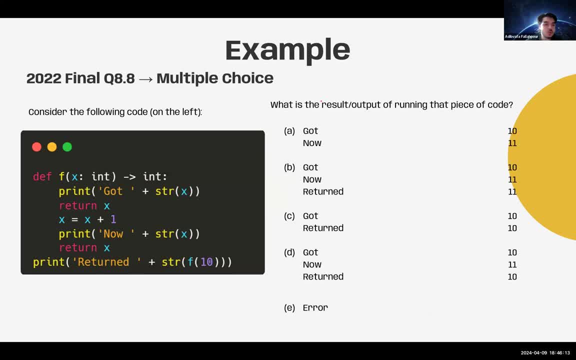 always run for any number of times that it's set. it doesn't really matter what happened inside the. a function named f and this is terrible naming for a function. Please name your function something reasonable in the exam. Like you know, f is not a good name. Maybe you can come up with a better. 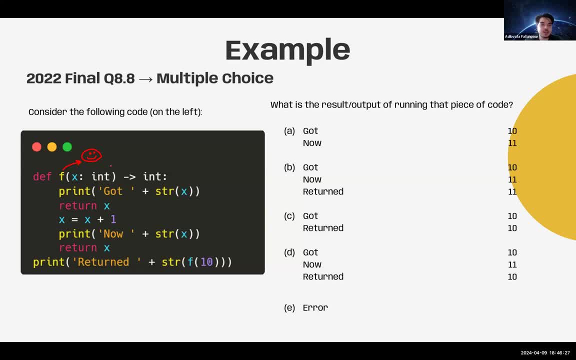 name And we have the function being run on an integer x and it returns an integer. Now we've run that on f of 10. Then we're getting the output making it a string, and then we're printing. So what is going to be the final? 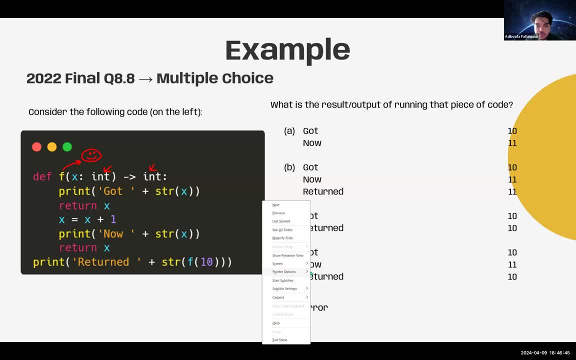 result, And this is from 2022 final exam. This space is a bit too wide. Like, consider this to be just one space. Why do we have two returns? That's a good question to ask. right, It means that the 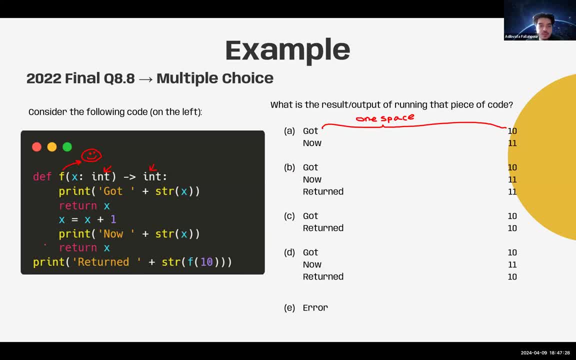 second return doesn't really matter, right? In other words, that two returns is there to trick you. It's not a good practice to have two return statements in the same part of the code. So, in other words, what your friend is saying is your friend is saying: once we reach return x. 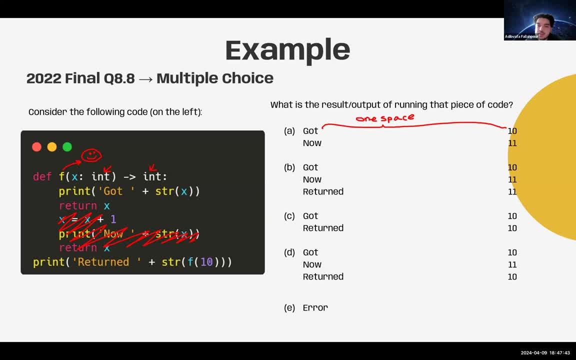 none of this code would run because we'll return the function, And that's one hint that will help you solve this question. So we do a print, we do a return and then we do another print. So what's going to be the answer, guys? 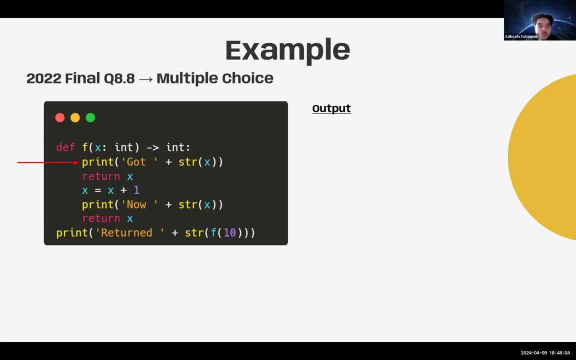 Yes, the answer is going to be C. So what do we do? We first go through it, We print: I got 10.. Then we return. So you're done with the function. So we just print the end result, which is the output. 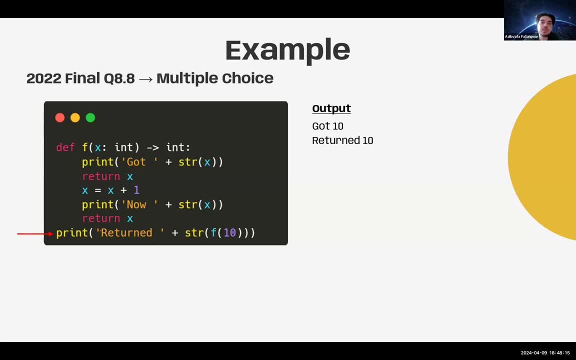 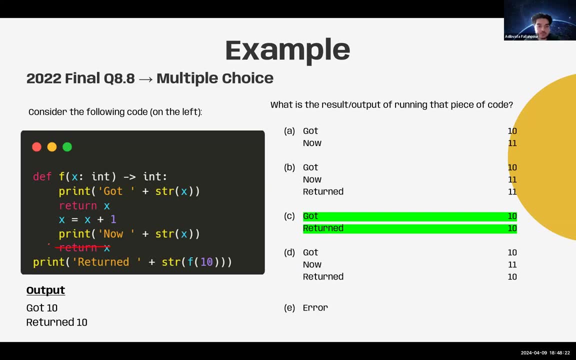 Since it returned x, which is say it returned 10.. And we do So. the answer is C. So you see, the second return will not run. That's a key, Or anything after the second. the first return will not run. That's a key observation. 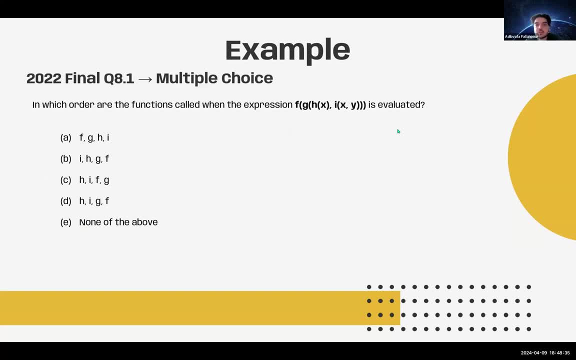 Moving on. So in which order are the functions called in the expression f, g, h, whatever is a value? So in which order are the functions called in the expression f, g, h, whatever is a value? Yes, So in other words, if your return statements are in different parts of the code? 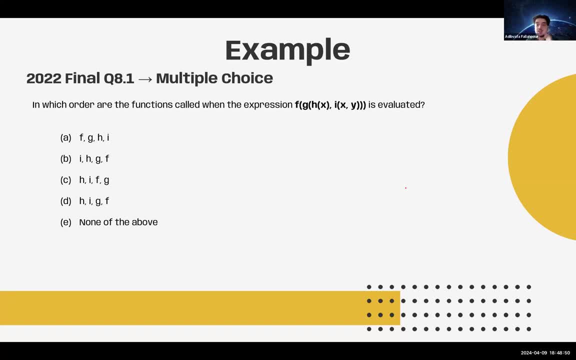 like one of them is under an if statement or one is somewhere else, then yes, maybe based on the input, this return will run. maybe that return will run. But if you're just guaranteed to run one of the returns, let's say it couldn't just be not using. if So, in your code you have. if true, 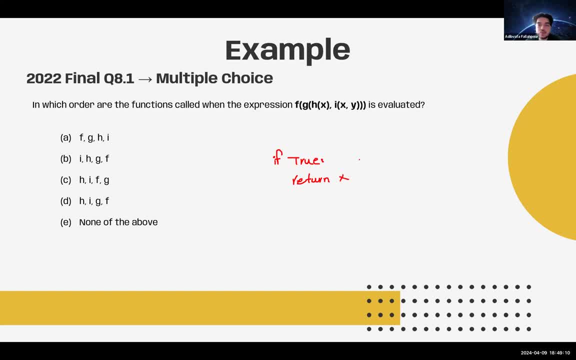 return x right? If you have this, you know, the moment you reach this if statement, you're going to be running and you're done, So any return that you have here won't matter, because you're guaranteed to return when you reach if true. 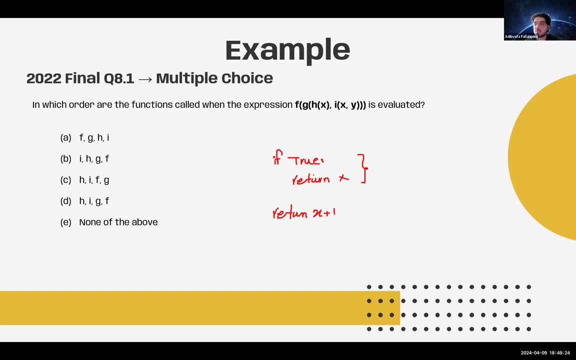 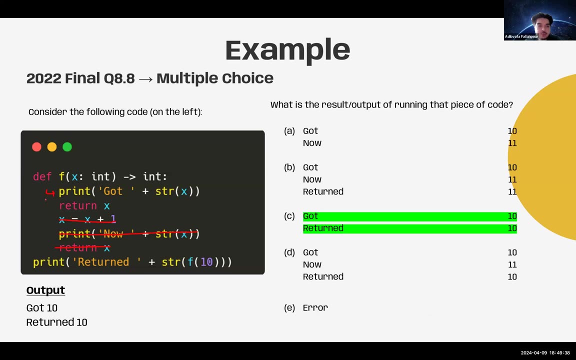 So once you're guaranteed to return something, then you're done with anything after that. And in the previous question we were done because we had a specific return statement saying you return, So that's it. It will return x. right, It will print and it will return x. It will not go through the rest of the. 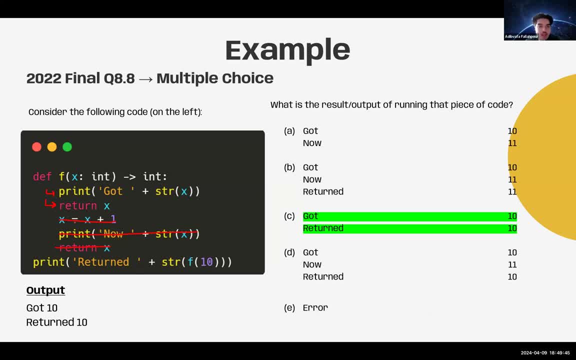 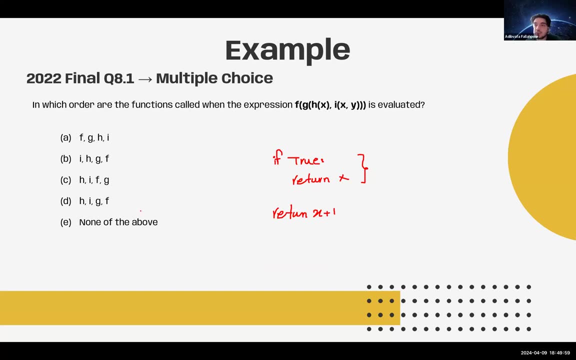 code, Because once it returns x, it will not have f anymore, like f will be done, And so it will not add something to x or print something or return it again. right, It's already returned and it's done. Your functions are one-time usable. They will not keep running Once they're done. 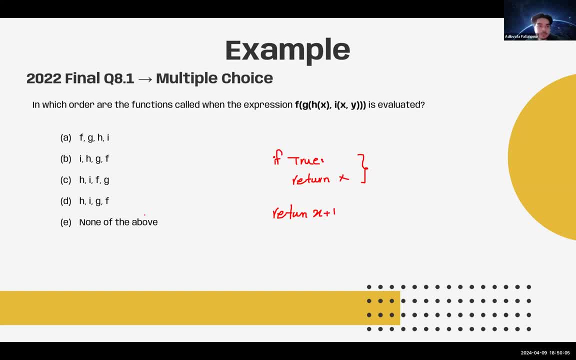 they're done. You have to rerun them again if you need to. So when you say fg of h, of x or whatever, which one is the order they're evaluated. So, as you can see, we start from the most inner part. So h is evaluated. 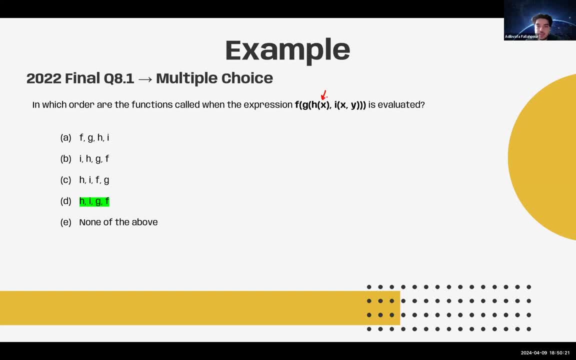 And then you keep coming out. In other words, you run h, then you run i, then run g and then f. So you just start from the most inner part and you just keep coming out. Now, why is h ran before i? This is just because it's from left to right. right, We first run h. 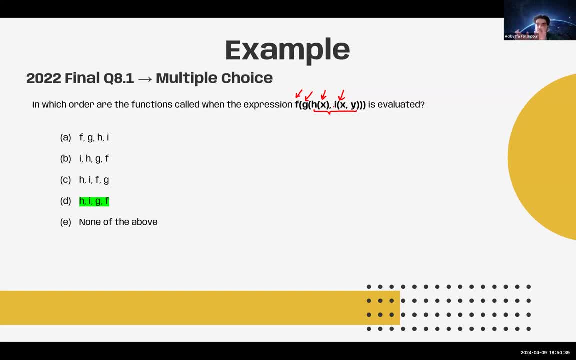 and then i. But these two are in the same heart, They're in the same middle of the code And once these two are both ran, then g and f will run. So i h, g, f is just because it's from left to right. 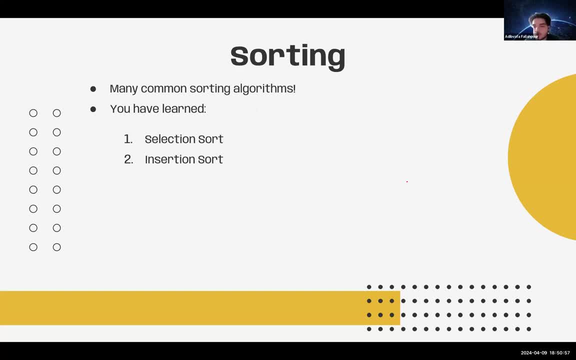 Already moving on, we have sorting. So you guys covered sorting, right, Like the selections for that insertion: Yes, No, Okay, How does everyone feel about sorting? Not good, Yeah, To be honest, sorting isI also agree it's a bit complicated And definitely the PCRS videos do not help. 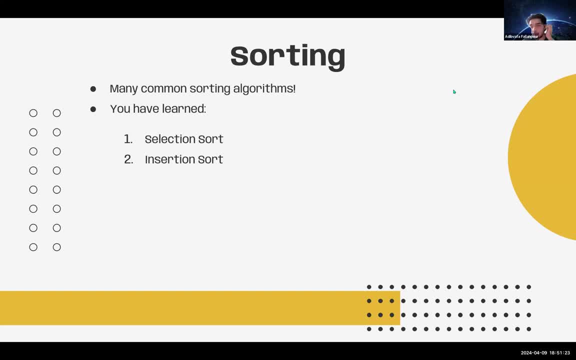 So what I do, suggest you guys do, is watch some good YouTube videos on sorting, because you really need to see good visualizations of how things are going to be able to grasp the idea of how sorting works. And if you do not have those videos in PCRS, then you have to find them from certain. 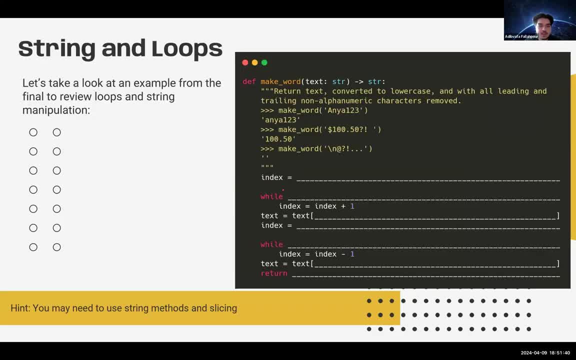 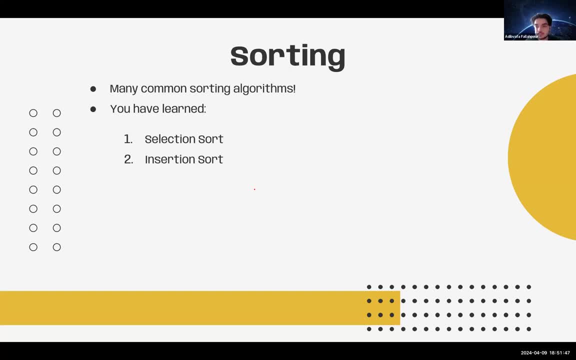 Now we have an example for sorting. I don't think we have any slides to cover how this sort of goes algorithms work and i guess the best way is really just going through. okay, um, i'll see in the break if i can bring some like good videos or good slides for sorting that. 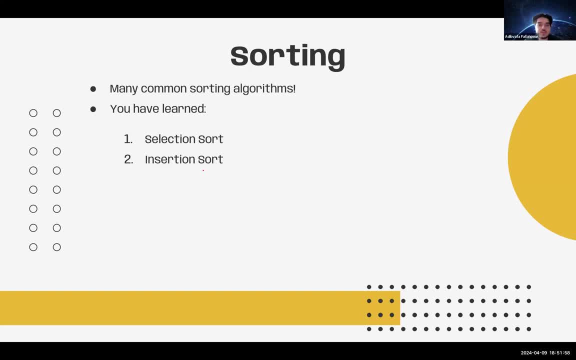 we can add, but in general definitely review sort. here you have selection and insert sort. i guess you also learn about bubble sort, which are the main tree sorting methods you learn in a8. for all of the sorting algorithms, make sure you know their best performance, their average performance and their worst performance. 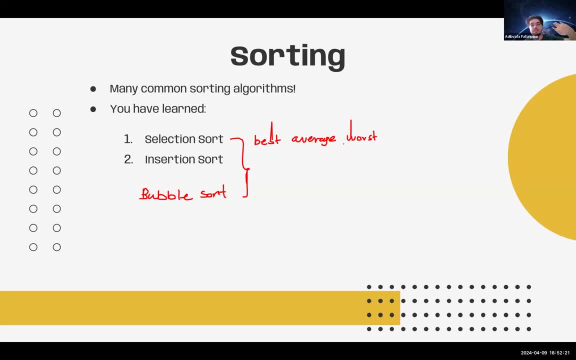 so you know the, you know order of how is the best, what is the best input, what is the average input, what is the worst input for these things- and personally i've never seen it in any final exam- they ask you to implement sorting from scratch. so if you're feeling overwhelmed, 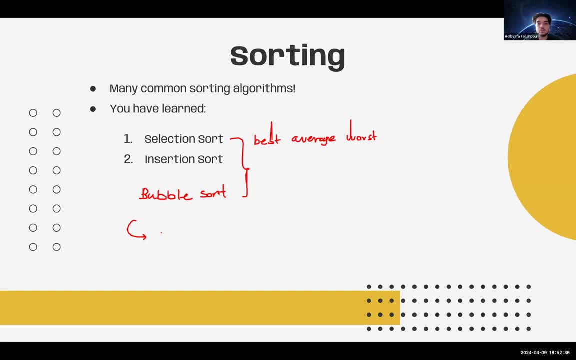 especially with insertion sort, which is pretty long. you don't need to memorize like the entire algorithm, but you should be confident that if i give you like a sorting algorithm and if mask some part of it, you say what is this line going to do? or whatever, you have to be able to fill in the gaps. 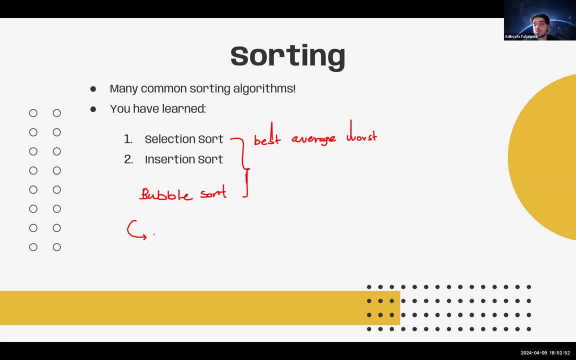 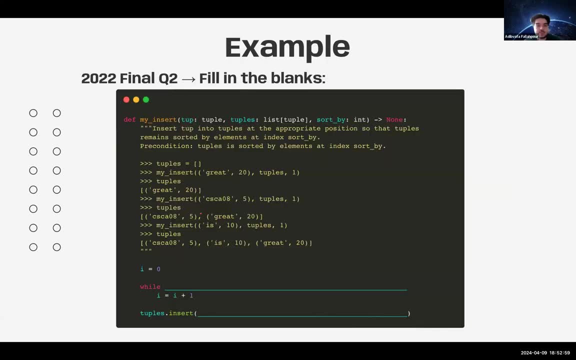 so i say, memorizing these sorting methods are good, but understanding them was more important, because that's eventually what's going to help you, okay already. so let's fill in the blanks. we just talked about filling the plants, and here's the question, and this was in cloud. 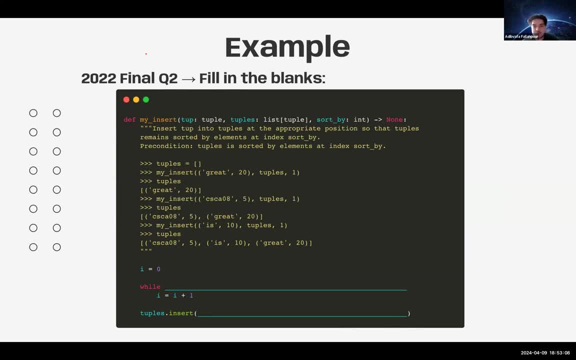 so you see, they did not ask you to do everything yourself. they give you a bit, but still you have to to know the sorting algorithm to yourself. So what is this function? This function is getting a tuple as input and a list of tuples, along with an integer. 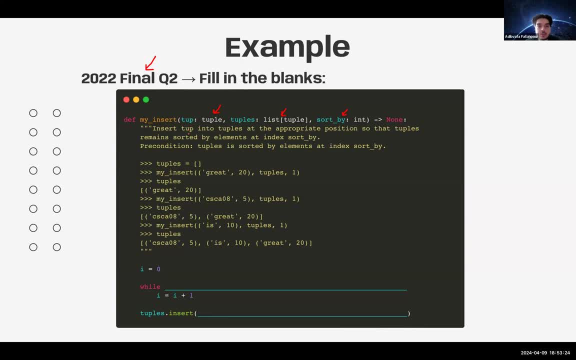 that it should be sorted, And so the goal here is to insert our tuple into the list of tuples at an appropriate position, such that the tuples remain sorted by elements at index order. So this is just examples. If your tuples is an empty list and you're saying insert, you know grade 20. 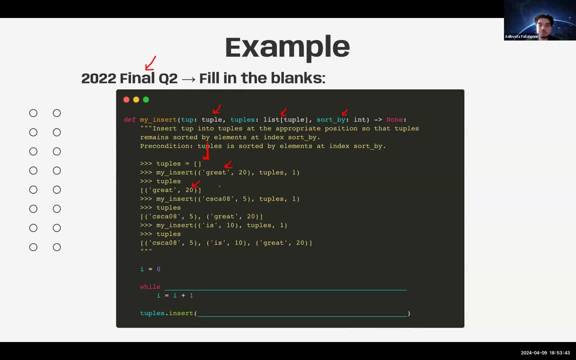 in this tuples, then it will just add pretty easy. However, now our tuples has one element. So if I say add another element with CSEO 8 and 5 and add it to index one, we will add it in the beginning. 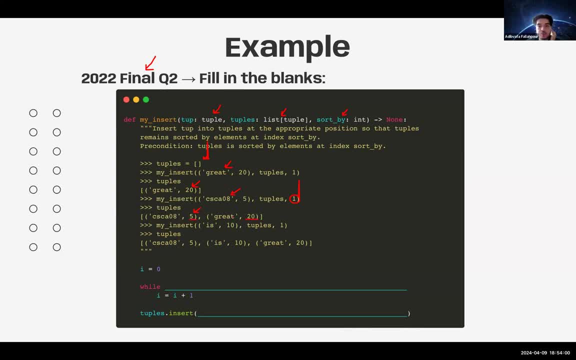 And the reason for that is number five is smaller than number 20, right? So we want CSEO 8 to come first, And if you want to do the same, if you want to do the same thing with is 10 to the same tuple, then you need to add it. 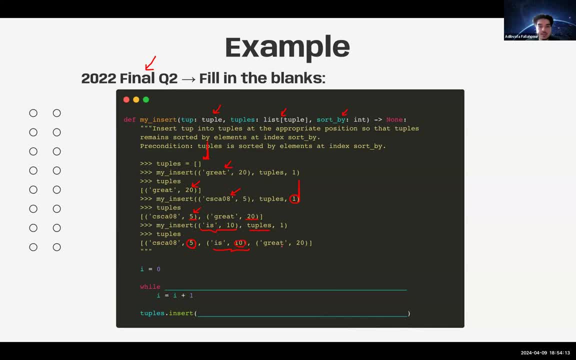 in the middle, because five is smaller than 10 and 10 is smaller than 20.. So this is not alphabetical order. This is the order that's defined by the index in the tuple. Now you might be wondering: well, how do you know? 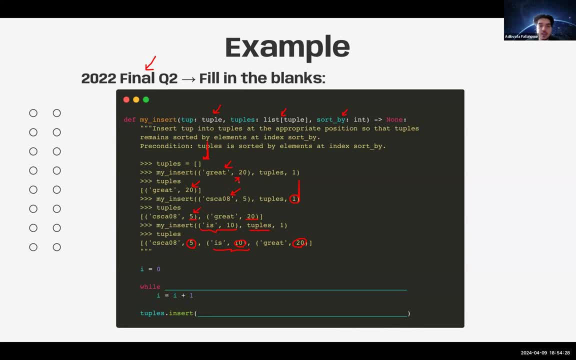 that you know, number 20 is in this first index and that is the sort by index that's given to you. That's why we have an index number one in all of these examples. It's telling us that the one element in that tuple 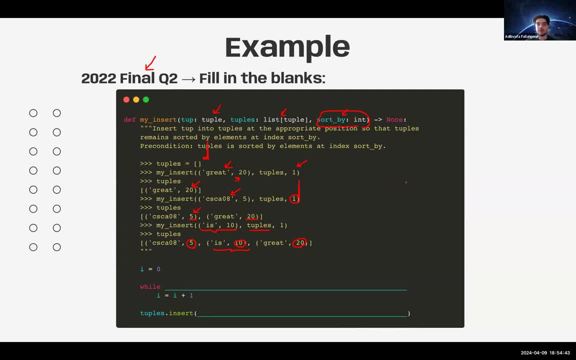 is the one that determines the index. So, for example, if you have, let's say, if you have, grade 21 as a single tuple, you will only look at the first, the third, not the first, the one index, which is this: 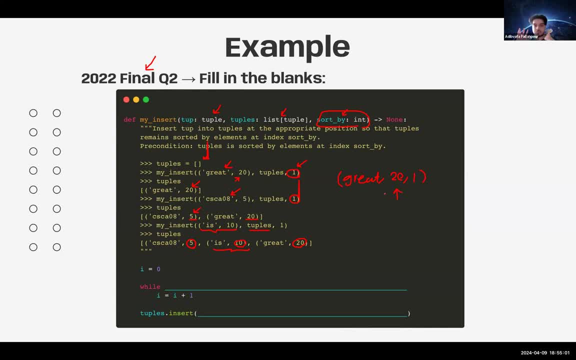 and you'll use that for certain. So are we all on the same page? Does the question make sense? No, I can go through it, but I'm going to give you guys a bit of time to actually implement this. It's not that straightforward. 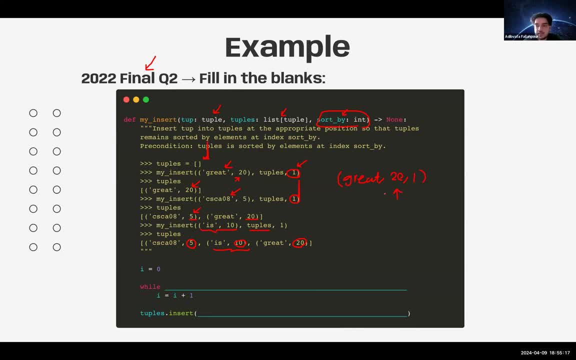 So yeah, take a couple minutes, think about how you can implement it. You start from an i equal to zero, You have a while loop and then you're inserting in your tuples, which is a list, And once you have a suggestion, write it in the chat. 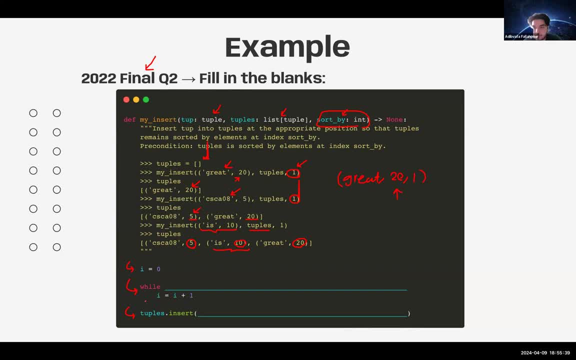 You can do that with any other endpoint. You're gonna figure out what the target is. It's gonna be a little bit more complicated in the test, but you can do it. So this is what I'm gonna do. So we have the first one. 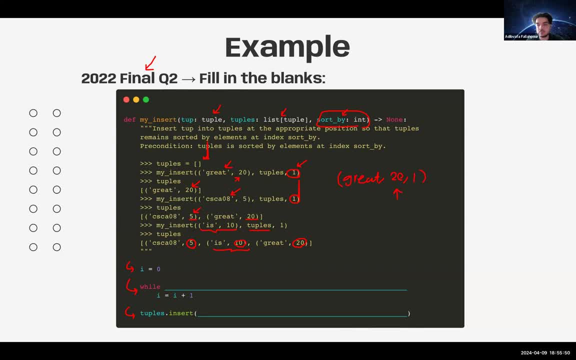 we have state class. So at the time where I'm gonna go paste really quick test and then after that I'm gonna go ahead, and I'm gonna go ahead and say I'm gonna go ahead and add it to my query. 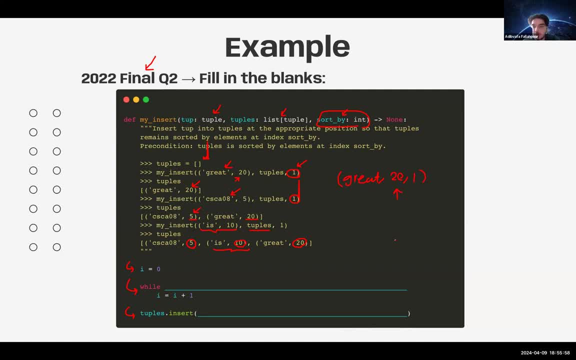 So all right, so this is the first one. Then I'm gonna make an i equal to zero, and then the second one, And then, on the last one, I'm gonna add the first to the line and I'm gonna say: 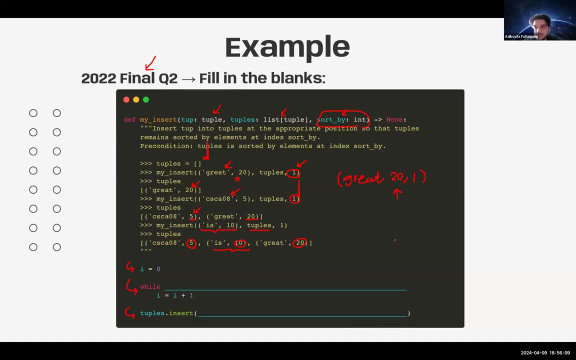 And you also have the topos that inserted it after. Now, remember, topos is a list, So it's the same insert method in the list that you guys have there. Anyone else with suggestions? I want to give you a hint In your while loop. your main goal is to update, i right? 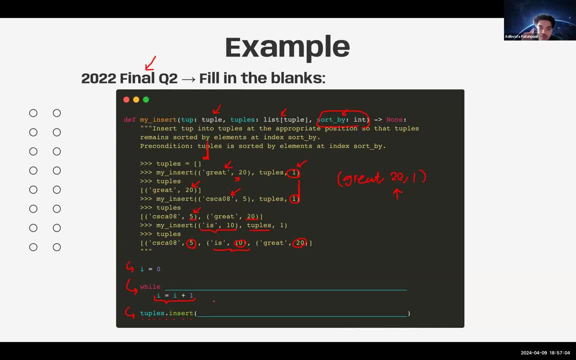 In other words, you want i to be at the right spot for insertion, So you have to check a condition that will allow you to keep increasing i up to a point that you are in the right position, And the right position is defined by that your topo is bigger than the ones before it. 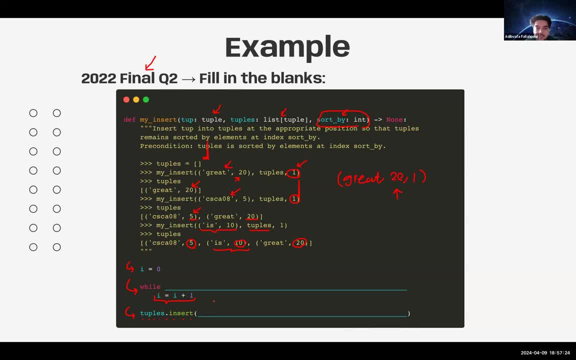 and smaller than the ones after it. If you say, while i is less than less then your, i will just go in the end. right, That will not really be sorted. It will just insert in the end. Your goal here is to use a different condition that will. 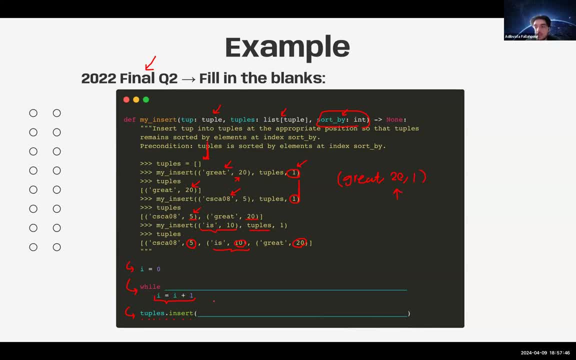 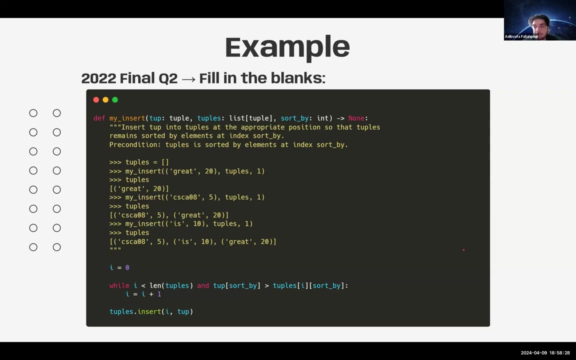 where should i stop increasing i and where should i stop increasing i? Anyone else with suggestions? All right, yes, That's, this is getting pretty good, So I guess you guys now know the correct answer. There are, in fact, two things that you need to check. 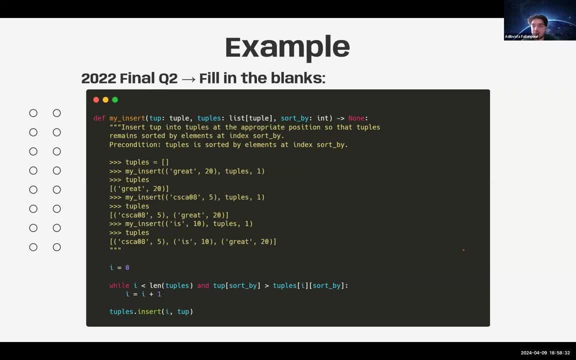 And none of you can tell me get correct answers. but if you guys collaborated on the exam you would get correct answer, but you shouldn't collaborate anyways. moving on, you need to check two things. one of them is as all of you thought about- is this: you need the- let's say the index of your tuple, let's say the. 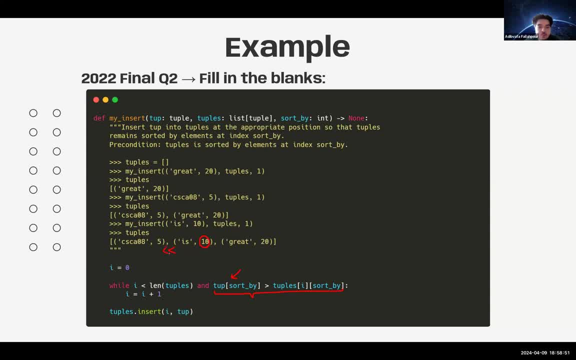 number that it's coming with to be larger than anything before. so you're going to keep checking for that. starting from i, zero, you're going to say okay, at the zeroth element: give me the current tuple and give me the number that it has. and for the current tuple that i have to put inside the 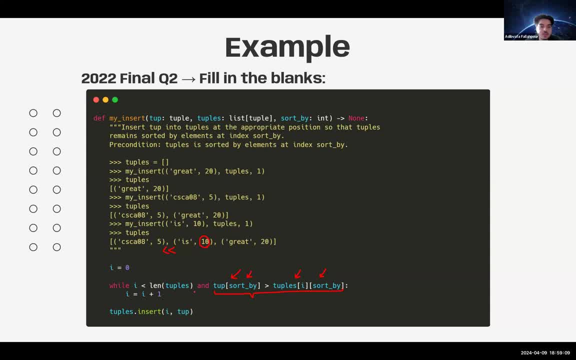 tuples list. give me the number it has and while i'm bigger than it, just keep going, keep going, one by one, until you find a sweet spot in which you know i'm bigger than anything before me. but the next item is bigger than me, so i should not move further. but you have to be careful with one thing. 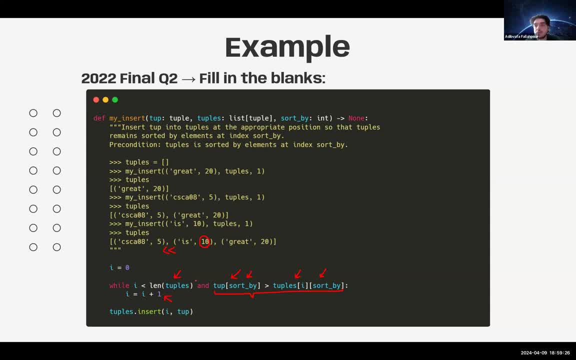 and that is, you cannot pass on the length of tuples. in other words, if you are bigger than all the elements, you have to be inserted in the end right and, as a result, once your i becomes equal to you should not keep increasing it because you've passed on, you know the border, so you have to stop the moment you 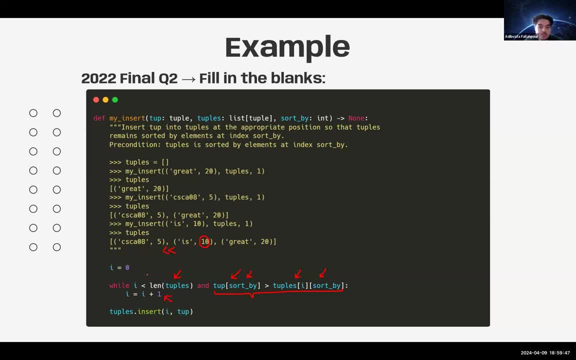 reach the last part of the list. and so in the case that, for example, let's say, you're adding tuple c with number 50 inside our list, your i will just keep getting bigger and bigger. it will be bigger than 5, will be bigger than 10, it will. 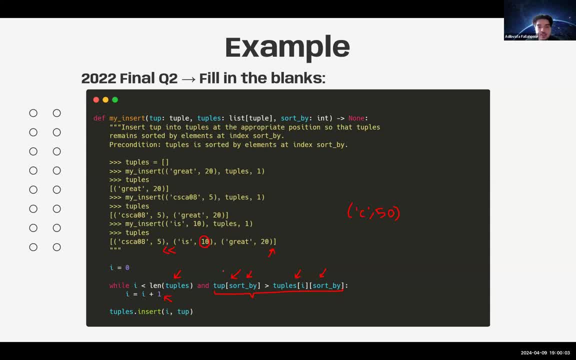 be bigger than 20. so it will be added in the end at index of you know this, for it starts from zero. this is not working. so i becomes one, i becomes two, i becomes three. it will be added at index three and the insertion is the same thing. you've seen, you know, you put the index and you put your tuple. 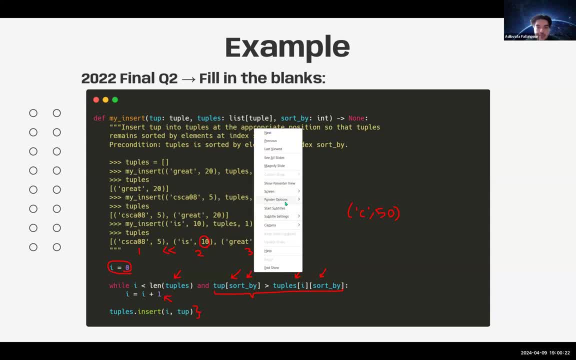 and it will be added into this. so just to summarize what happened here, there are two observations. one of them is: you want to increase your i. you want to keep going through the list to find a sweet spot, and the way you want to find that sweet spot is by comparing the element. 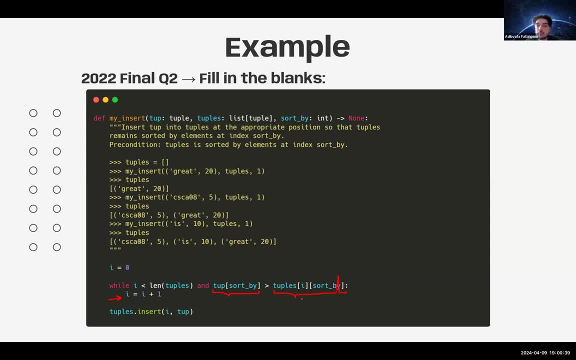 responsible for sorting to the current element in the tuples. so for our, you know, i want to sort my tuple inside this list. i'm going to just keep checking. is it bigger than the first tuple? yes. is it bigger than the second? yes. is it being the third one? no. so i found a sweet spot and that's. 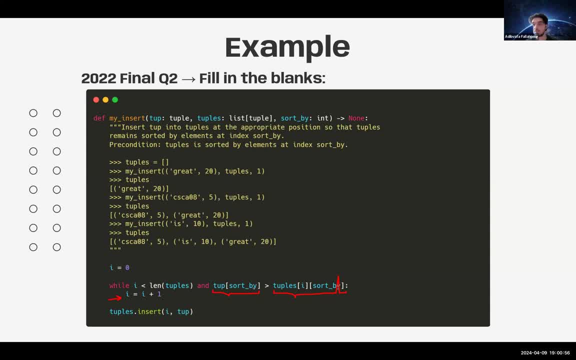 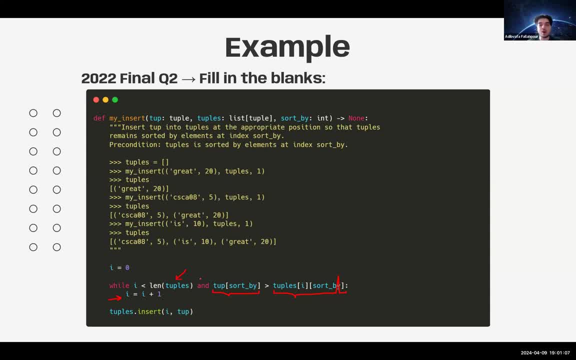 this. so i'm going to also add a second condition. at the moment you see your on out of bounds, stop and go at it in the end of the list. so this is pretty, you know, nasty the way, i would say, because many of you will probably come up with this one, but coming up with this one is a bit hard. 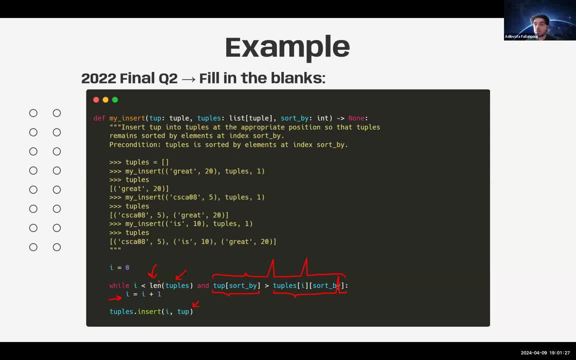 and that's one of the reasons you should really check and think about the code you're writing. does it make sense why we have two conditions that you're checking? okay, one person understands out of 65. that's progress. two people, only two. maybe some people are in the meditation room having fun, i don't know. is anyone there? 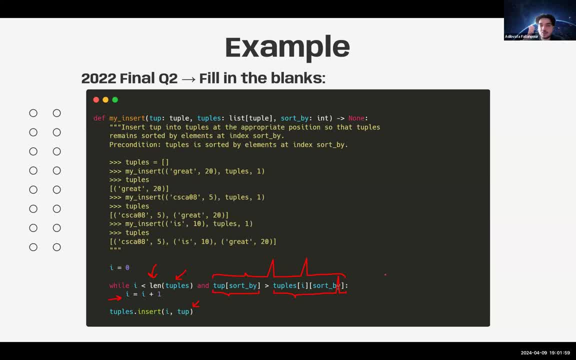 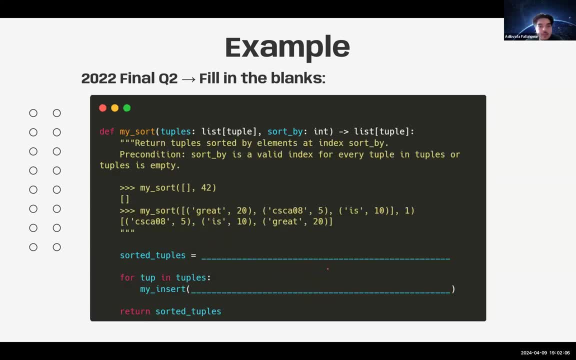 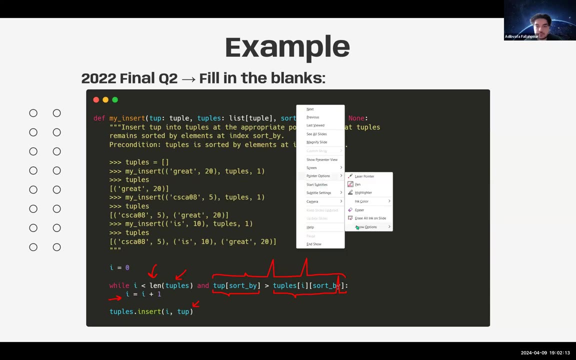 right, three people, i'm satisfied. three is good. so definitely go through these examples to make sure you understand how things are working. and we have the next one. so now you must learn about my insert. my insert was this function. the goal was again to add a tuple in a list of tuples in the right. 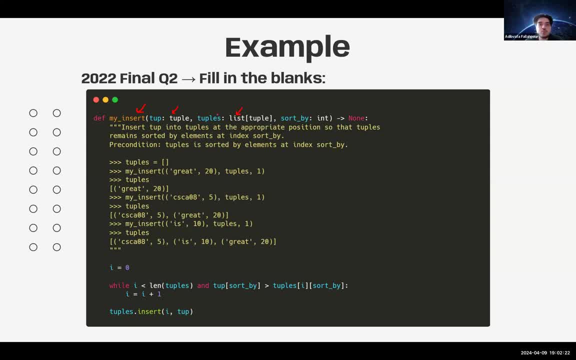 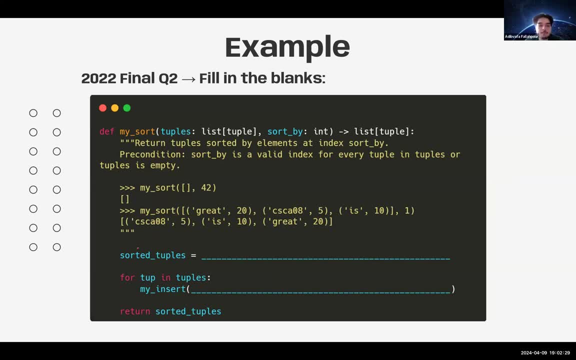 position and the element of the tuple you would choose to compare is the element at sort by index. now, what you're doing here? you're saying you're using that inside another function. now what does your bigger function is trying to do? it takes in a list of tuples and it just takes the. 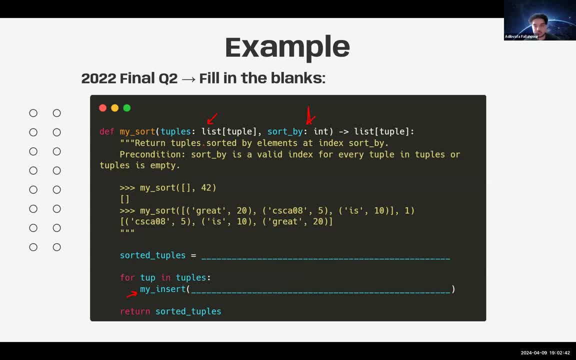 sort by integer and it will sort the tuples inside that list. in other words, you'll start from a list of tuples that might not be sorted direct. some tuples are just randomly thrown at it and you want to end up with a list of tuples that's just nicely ordered. 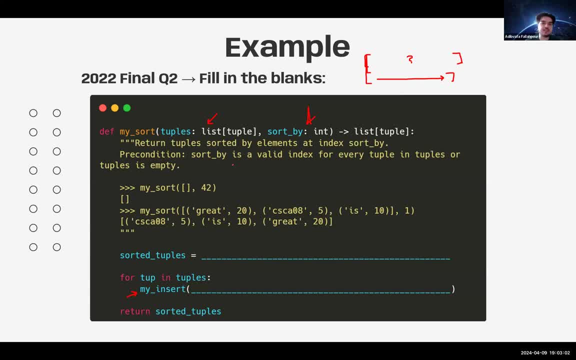 and sorted. the precondition is sort by the value, index, etc. so everything makes sense and you can see the example. if you're just trying to sort an empty list, you get an empty list, right? if you're trying to sort this list of three tuples, then you get the same list. but now they're in the correct order. 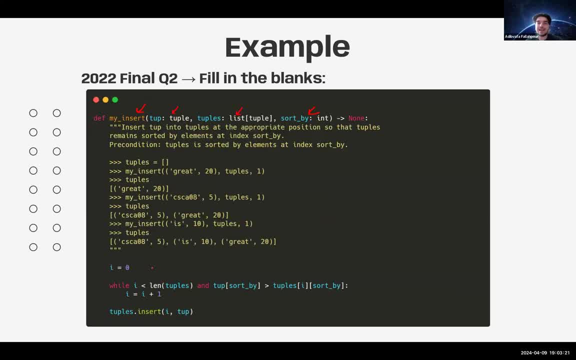 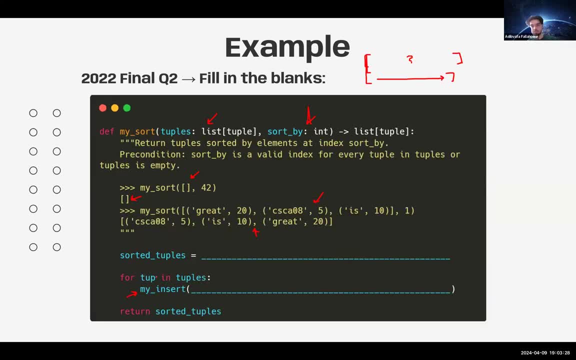 how do you use the previous function, whose job was to add a tuple into a list at the right position, to make sure all the tuples are in the right positions and just sort it in the right relation to this list. you'll see it so you can spot how you polygons this time. 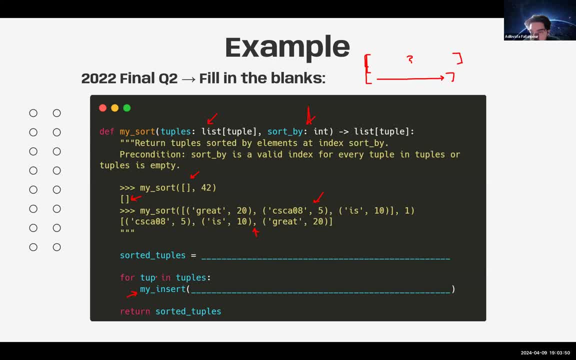 you can. Eve spoke in our left-hand他的 empty list that's going to have the sorted tuples as we go. then what do we do here? in my insert, just to remember, the first one is a tuple. then there's a list of tuples and there's the sort by. 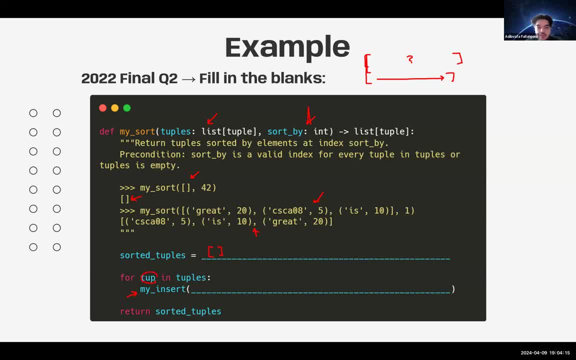 so which they're right now? we have this, have these and we have these. so we just want to bring them together exactly. so you want to say my insert starts with tuple, correct order. then you have sorted tuples, which is the list, and you have the sort by: 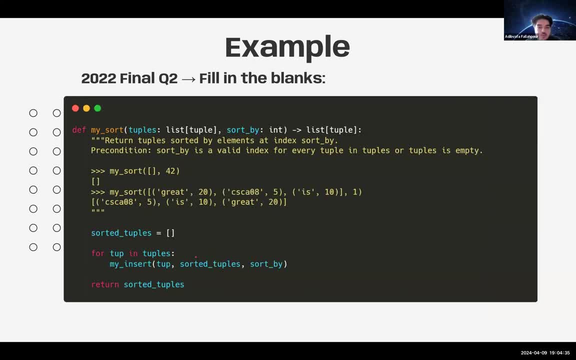 index. you're done and that's what we have here. so we start from an empty list. we add that. we go through each of the tuples, we add the first one to that empty list, we add the second one in the correct order, we add the third one in the correct order. so you're, you know, reordering everything as. 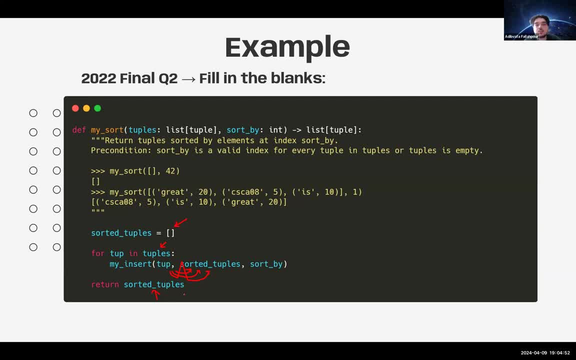 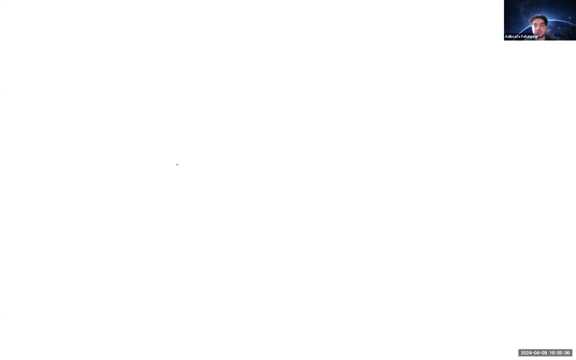 we go and then we return a new list that has all the sorted tuples. now you asked that it's so confusing to go through. you know tuples and dictionaries and lists and how we slice them. so just to do a quick summary and if you're wondering how i created a white, 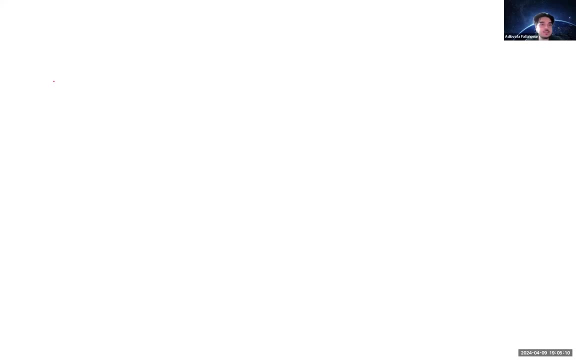 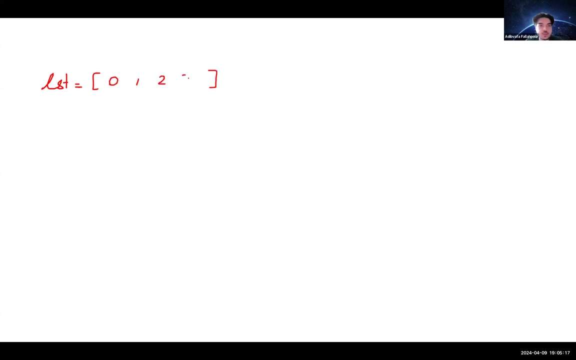 page here. it is sort of magic as you can. i guess list is something we've already got like a list. it has a bunch of elements, say zero, one, two, etc. and you can easily index it by saying which element you want. you can also slice it by saying which groups. 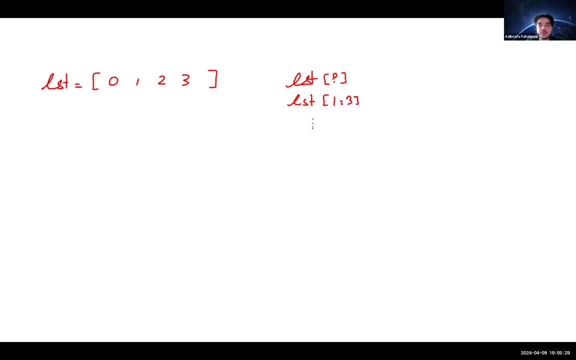 elements, for example, you want, and there are all sorts of other things you can do. that's easy. what becomes challenging is dealing with dictionaries and tops, now tuples. think of them as again similar to lists. instead of being defined by brackets, they're defined by a parenthesis. they have differences, like you know. you cannot change the items in the tuple while you. 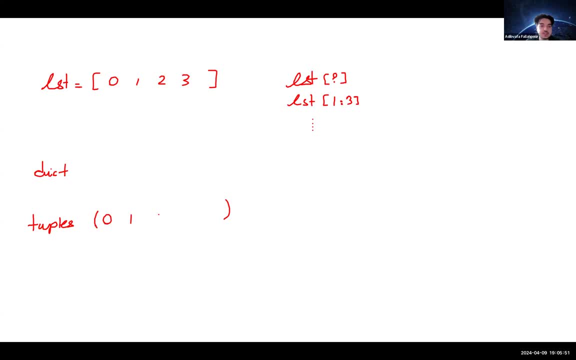 can't change the other list, etc, etc. but the slicing is still the same. you will say: my tuple with a tp, whatever elements i can strike, strike it like that and i can also slice right. so the slicing works the same. the only difference is you cannot change the values in that top. the tuple is they. 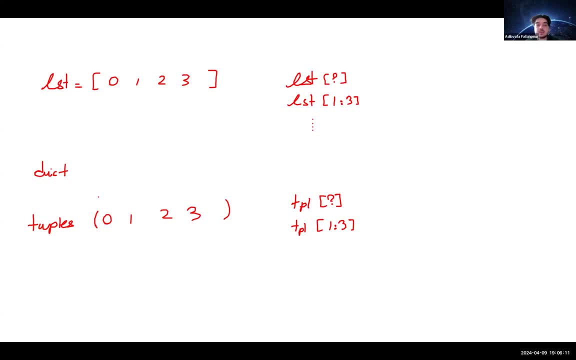 call it immutable, whatever. you cannot change the values. they're fixed on a circuit. now a dictionary is a whole new thing, because in a dictionary you don't have any internal order right. what you have is key and value pairs. you might have, you know, a name like my name. then you have my grade, which is: 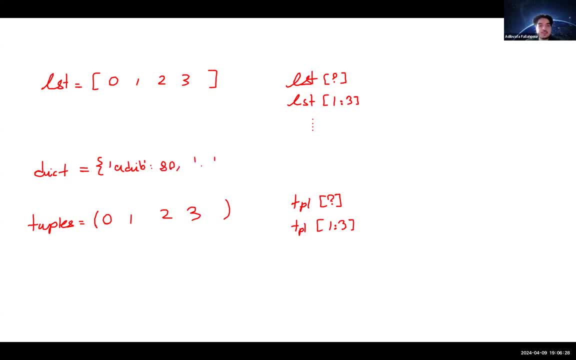 maybe 80, hopefully, and then you have a different name, maybe, maybe jacob is here and jacob's getting 100.. so this is a dictionary. now, even though you see it in a specific order, it doesn't really have an order like internally. the only thing that matters for slicing a dictionary is saying what. 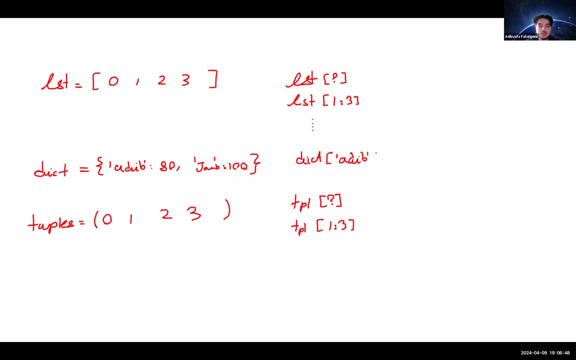 key you're referring to. are you looking for the adib key or the jacob key? and based on the key you put some, the dictionary will return to the value associated with it, which is the case a. so you could do a lot of nasty things right. you could have a dictionary of a string, but this: 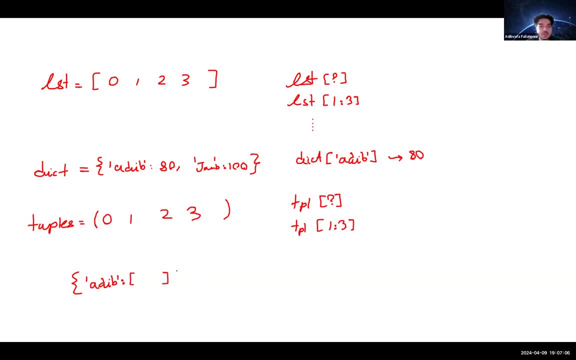 string refers to a list. right now, you might say: well, this is so confusing, like you know mixing things, but the same idea is again. well, you might say: okay, i want deep as my key and i want the first l and this should give me. now, if you go through it one by one, it will give me the list. 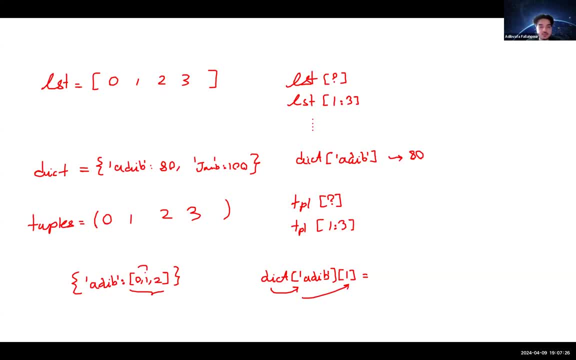 here and then it will give me the first element of that list, which is number one. so i get one right and of course we can just keep going right. you can define like a, you know, can define a list of dictionaries. we're going to do the opposite. we have a list here. 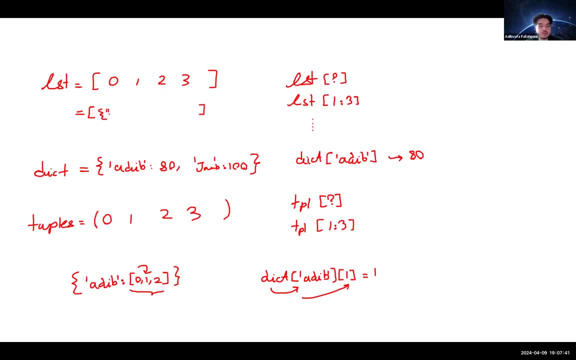 but each item is a dictionary. here is like i'm going to just make it smaller so we have space like a refers to one. that's our first dictionary. then we have a topple of you know dictionaries. so we're just going to cook something up, these two, whatever. and now i'm going to say what is lst one. 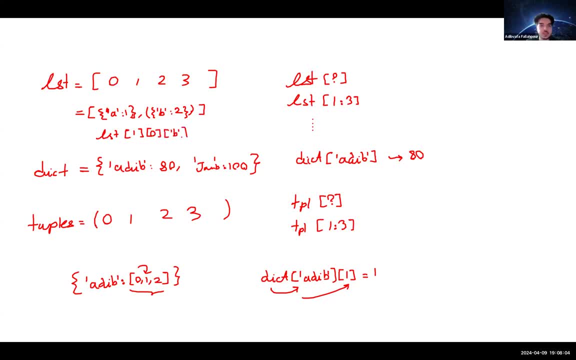 um zero b and you're going to say, oh, it's equal to two and the key to solving these types of really nasty things is just by going through it one step out. lst1 is the first element, or the first index. the zeroth of that one is the zeroth element of the topple, which is a dictionary. 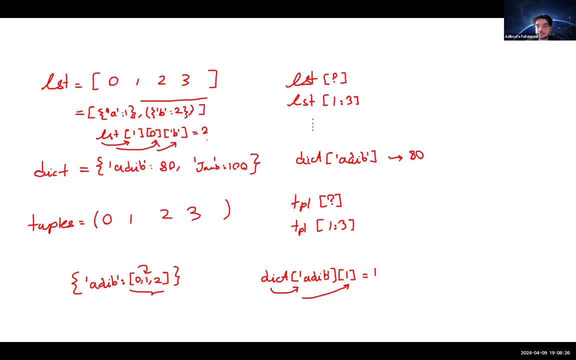 and the b of that dictionary will give me number two. now someone has this. can you use functions like a range or length for dictionary and topple like you do for this? you can't use length in general. you can use length for a lot of things, a lot of. 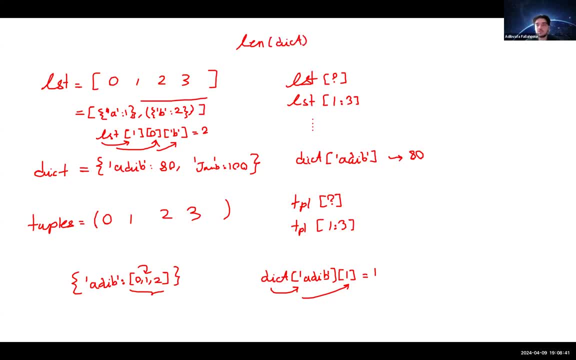 data structures like len of a dictionary will give you the total number of pairs you have. len of a topo is the same as len of a list. it will give you the number of elements in it, but range depends on how exactly you're using. so, for example, you can say for: 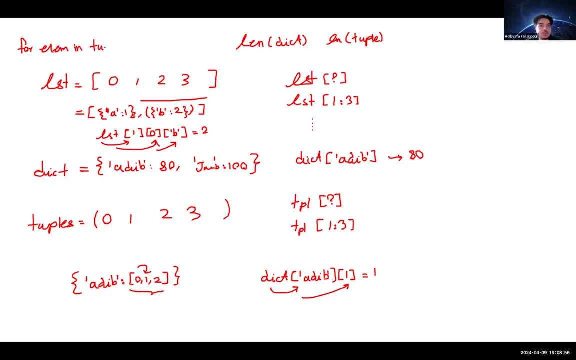 element in tuple, And that's the way you say for element in tuple, for element in list. both of them work. Just go through the elements of that top list. But you can say for element in dictionary, because dictionary doesn't have any element. 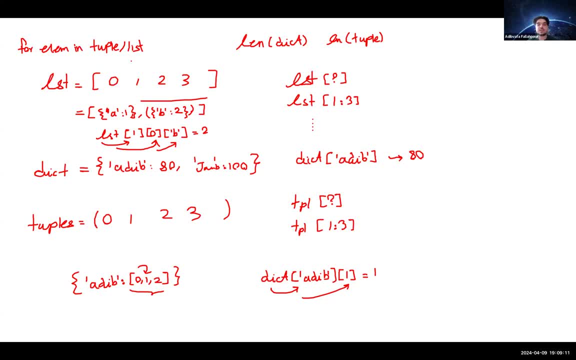 It has key value. right, Think of dictionary as a person that you give it a key gives you a value, something like that. But you might be wondering then, how do you go through the items of the dictionary? And there's a built-in function called dictitems. 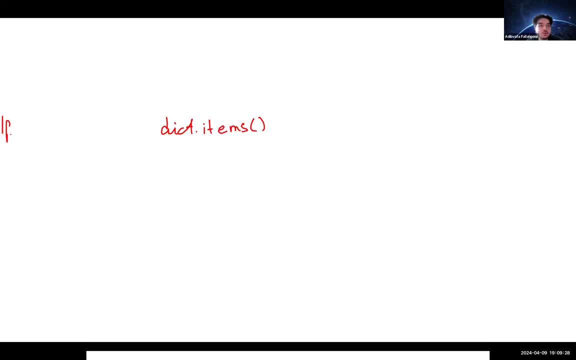 And dictitems will give you the items one by one So you can say for key value in dictitems And what it does. it goes through the items of the dictionary And each time it will assign the key to this variable here and value to this other variable. 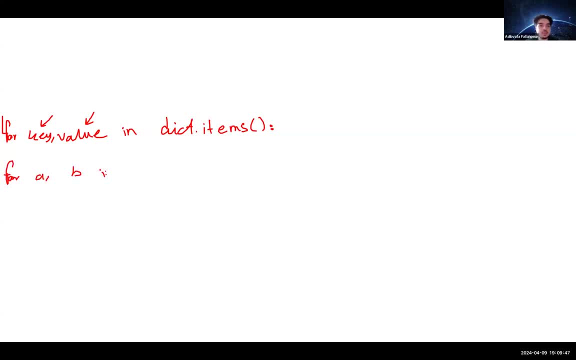 And you can call this anything You can say for A and B dictitems. It's your average for loop. Why does it have two variables? It's just because an item in a dictionary has key and value, So they're a pair. 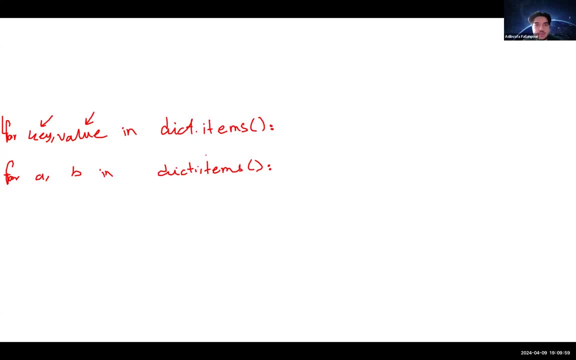 You can't just get one of them. Now you might say: well, what if I just wanted the keys in the dictionary? Then Python is like: well, you have to say dictkeys, And this will give you just the keys. So you can say: for any key inside, dictkeys. 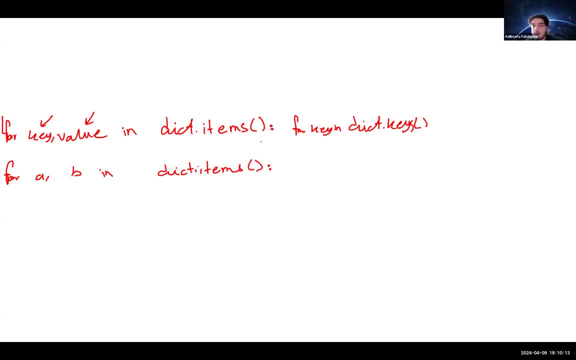 give me the keys And that's how it goes. So it's quite. you know, it seems like English And just make sure that you're comfortable with this, This idea of having two variables in your for loop. They get assigned as you go. 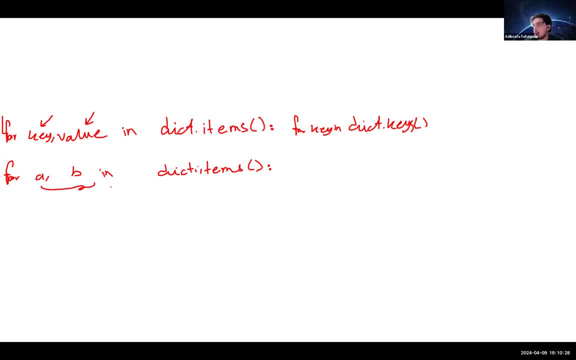 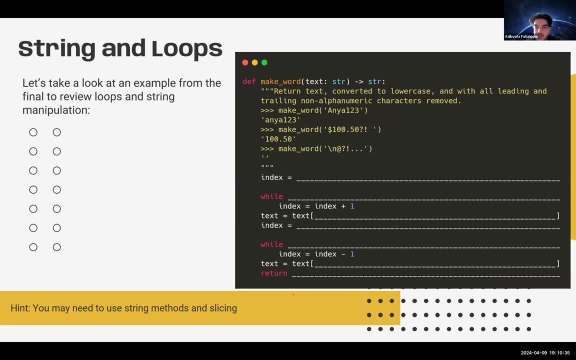 Does it make sense now? It's a quick recap And I guess this is a good time to move on to Elancrit, right? I mean when you're registering F-loops? OK, let me stop sharing. Let's take a two-minute bio break, or no five minutes. 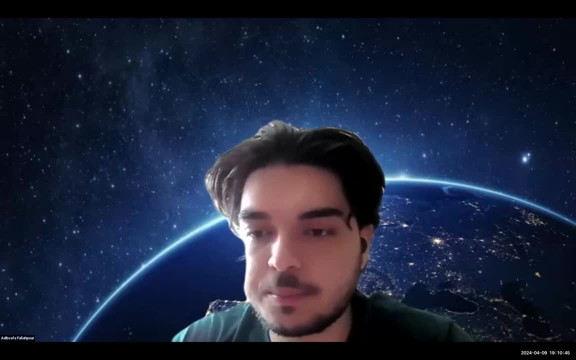 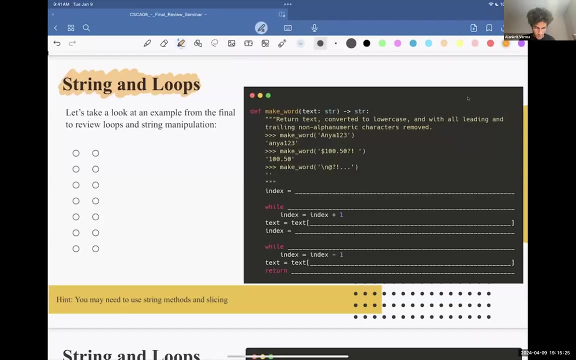 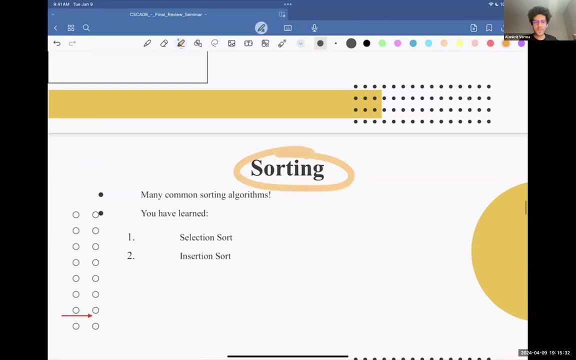 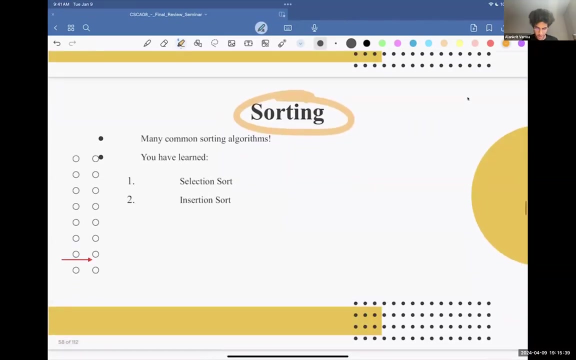 We'll be back at 7.15. And then we'll go through the rest, OK. OK, so we covered a lot of stuff about sorting. I just want to make sure. do you guys have any questions about the thing, anything about sorting? 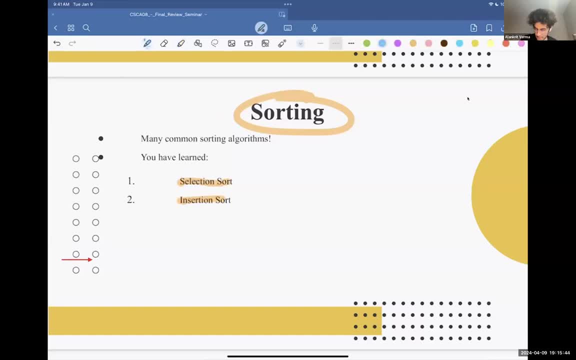 We had insertion sort and selection sort, And there's also a thing about searching. Do you guys have any questions about that? Yeah, No. If you guys have any questions, say yes, And if you don't, thumbs up Who can't see the reactions. 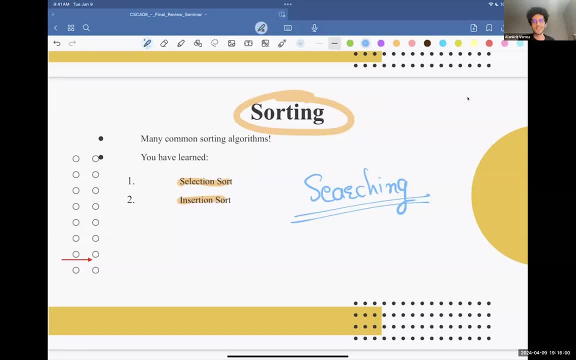 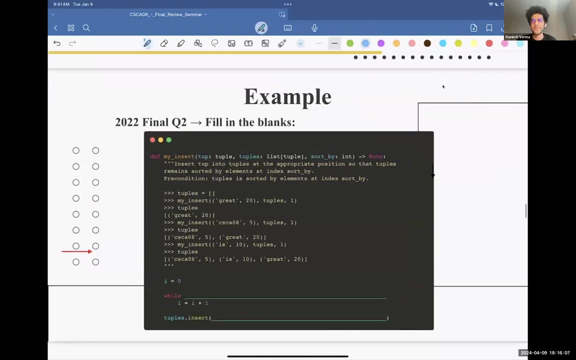 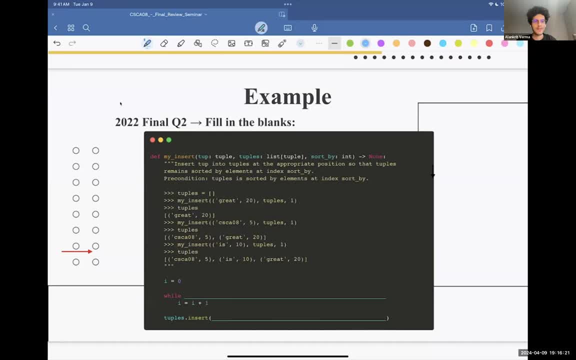 Yeah, Yeah, Yeah, Yeah Yeah. All right, Exactly, Exactly. OK, I can't see the reaction for some very reason. It would be good if you can speak or type it in the chat. Two options: speak or type it in the chat. 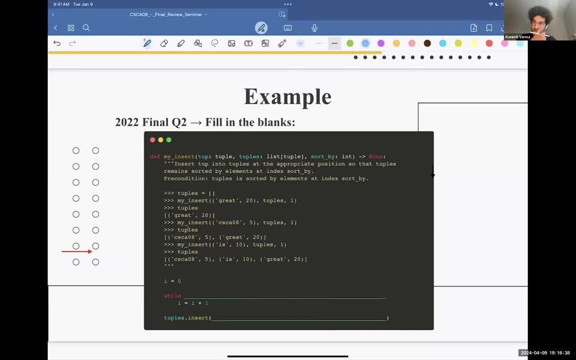 OK, So wait, what was the reaction? Can somebody just type it in the chat to tell me what the reaction were? Do you guys want me to cover it again? Or what's happening with searching for things, Or just speak up Like I'm perfectly fine with it? 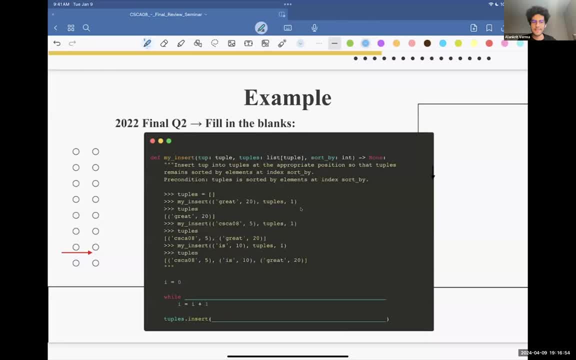 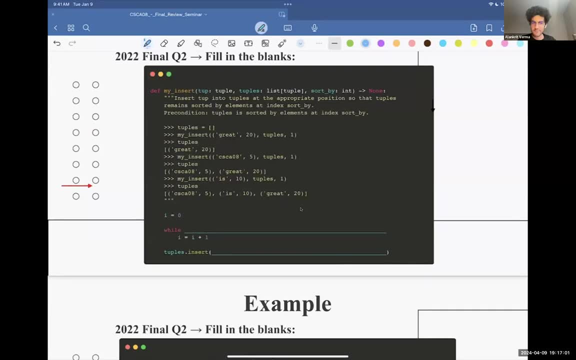 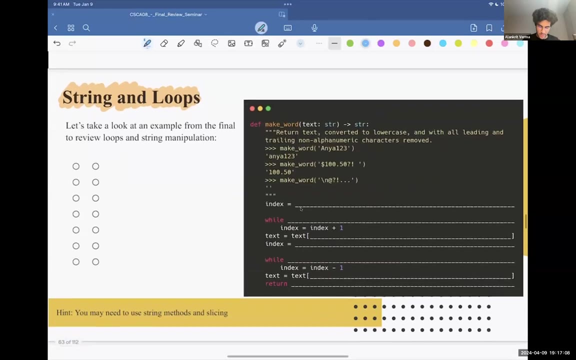 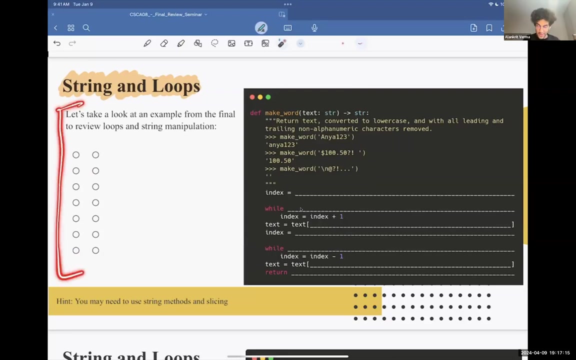 fine with anybody just unmuting if we've got to be fast. no, okay, I will assume that everybody is fine with that stuff and move on to the next topic, which is searching and string and loops. okay, if you guys were in my midterm degree seminar, I like to do one thing: 20 seconds and I want everybody to read. 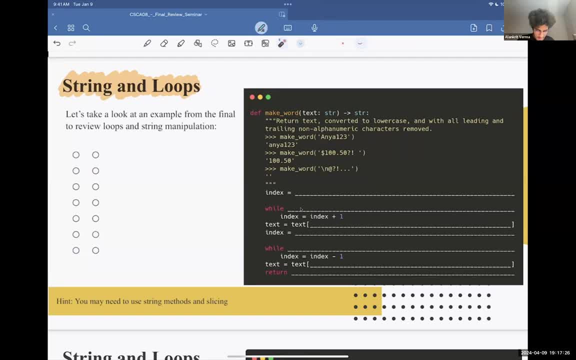 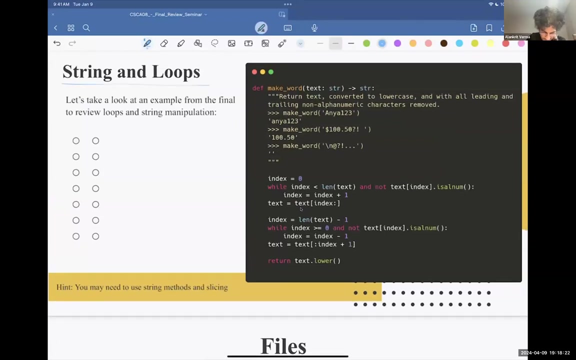 this question just 20 seconds and read this question. once done, yes, in the tag will be you. try it like you have a pen and paper. try it completely. yeah, okay, you, let's look at the solution for this. so what is happening? strings and loops- let's take a look. 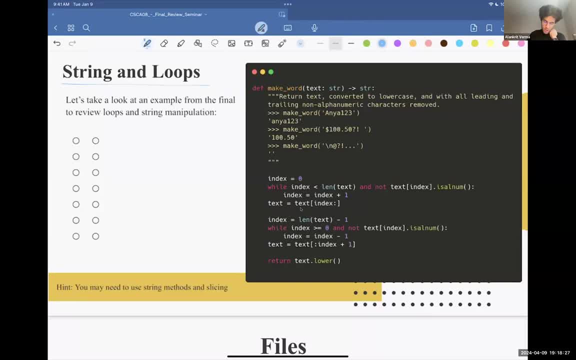 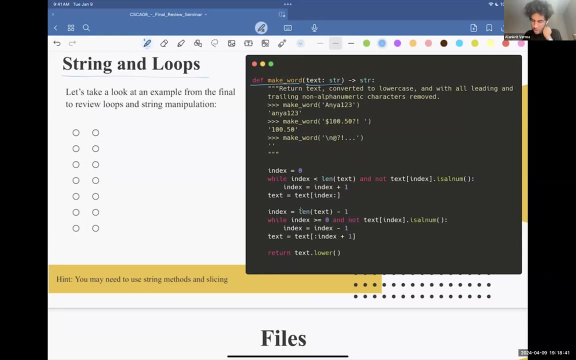 at an example from the final to review loops and string manipulation. so there's a function called as dev make words- which takes in a string which is text, and then what does it do? return text converted to lowercase, with all leading and trailing non-alpha numeric characters removed. 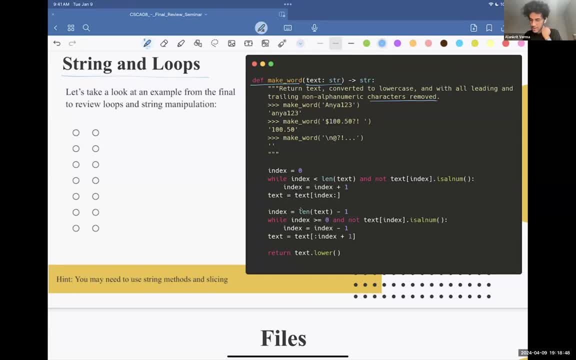 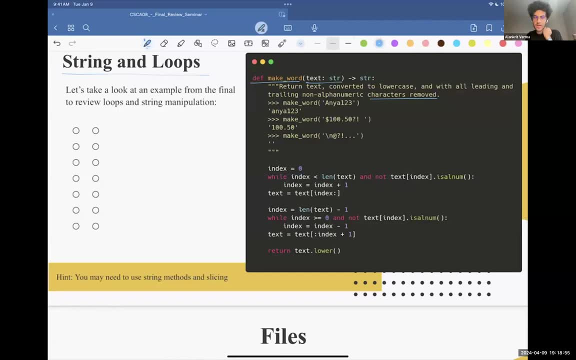 return text converted to lowercase, with all leading and trailing non-alpha numeric characters removed. okay, so what is this doing? it starts with: index is equal to zero. what is this? index is equal to zero is, more or less, in very generic sense, a looping variable. so when you have to loop, 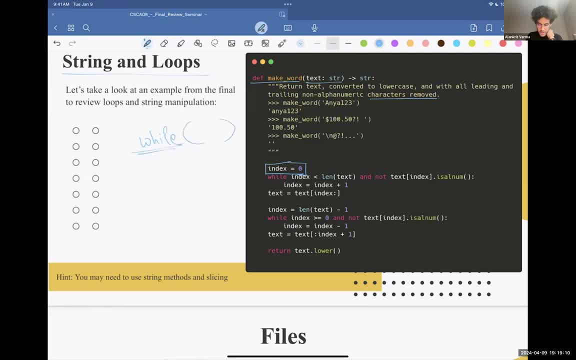 in while loops. you have a condition here and this condition is the terminating condition for the while loop. so if this is false, the while loop will end. it will go here in some percent. this index variable, the looping variable, is the- is the very variable which keep on changing inside the loop in each iteration. so if you can see, here is: 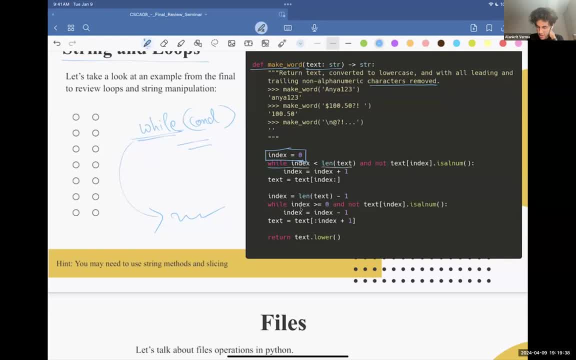 while index is less than length of text and not this, not as important text- the character at index: index. if that is alpha numeric, then what do we do? we increase the index? is everything fine till now. I don't necessarily like this online thing, but yeah, okay, if you guys. 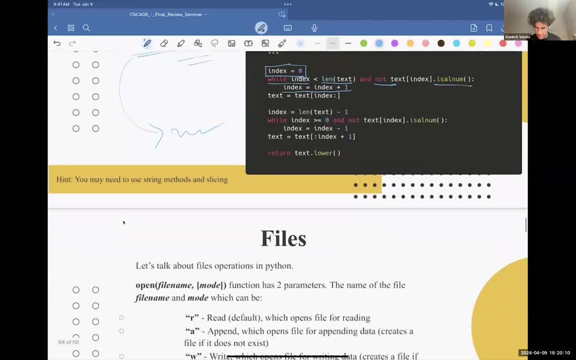 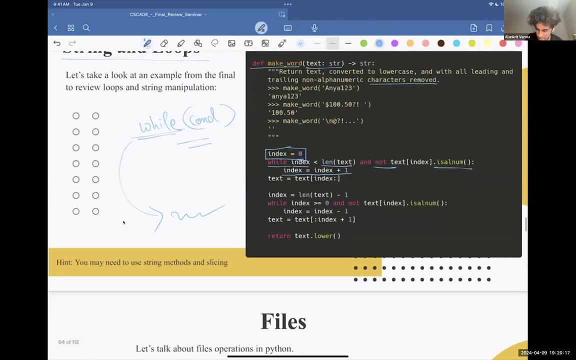 want me to go a bit fast, we can go, but the later sides to be faster, okay. so what did we do? so if we had this as our input? we check: index is less than text, index is less than length of text and at this very index, for example, zero. if that is alpha numeric, if 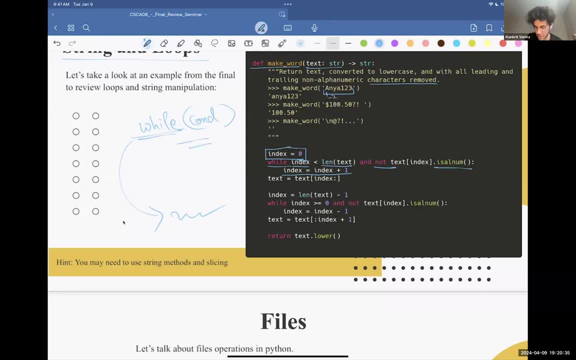 it is, then we move on to the next one. if it is, then we go to the next one, and then we keep on going in something and then we, at a point, what do we have? we have something like this. so this is a string manipulation here, string as ABC, and I'm going to. does anybody want to tell what? 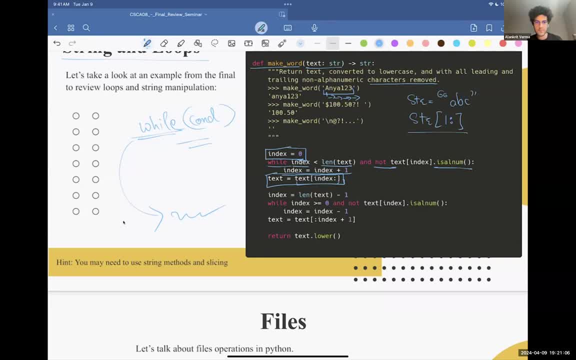 will this give BC? okay, just a quick. I know you guys typed in fast. it's a good way to do it. we've got this one graduated right after the rubrics. it will BBC. that's fine, but it will be this b-scurly or. this thing is very, very important and 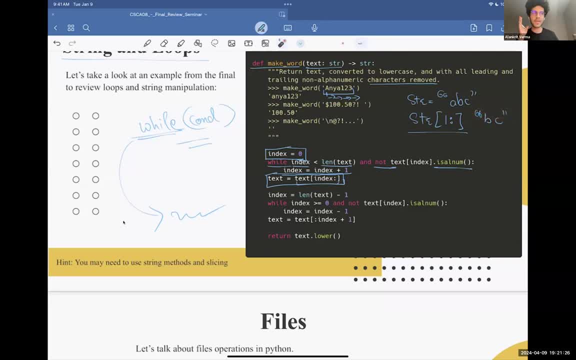 And Submire Trump. this question was in one of these finals. there už, their options were: without achieving, without the cameras. wirklich, pepperasia of text. okay, that's great, The correct answer of that, mano. And ah, last one, I don't understand if it is true or false. not, oh, good question is. 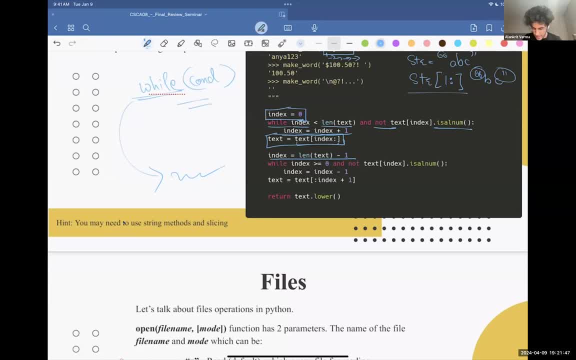 So next part of the answer: in some sense, index is equals to length, text minus one. so we had a particular index which we got from. here we are reducing it by one. and then what are we doing? we are looping in a very similar sense. we are looping in a very similar sense. 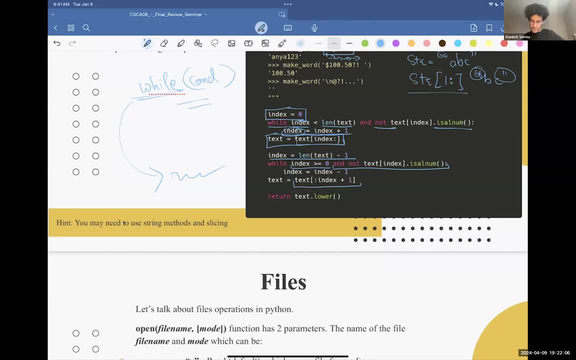 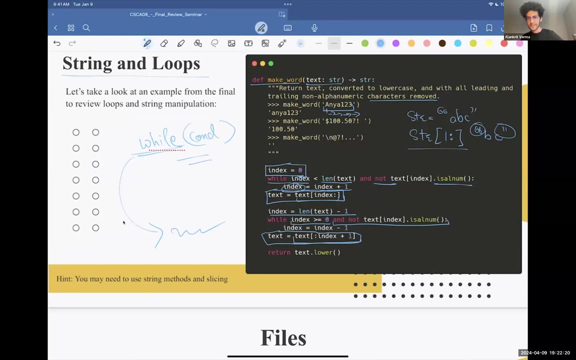 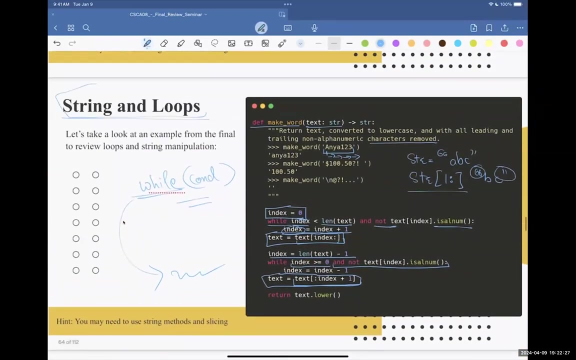 and at the very end, and at the very end, we get something like this: this should be easy. this is more like my thumb syllabus too. okay, it is everybody kind of fine with it, could you sorry? yeah, could you um repeat the part after we made. index is equal to length of text. 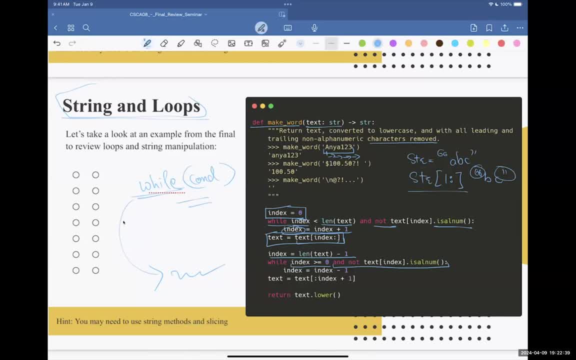 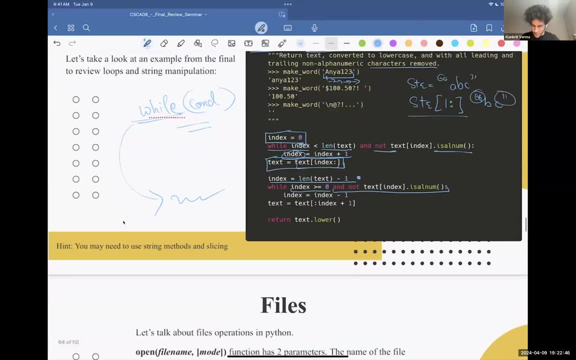 minus one, like that part. could you repeat what? sorry, yeah, could you, um, repeat the part after we made: index is equal to length of text minus one. what? what went down with that? okay, so, uh, we are at length of text minus one, right? and then what are we doing? we are reducing the index. and how much are we reducing the index by? 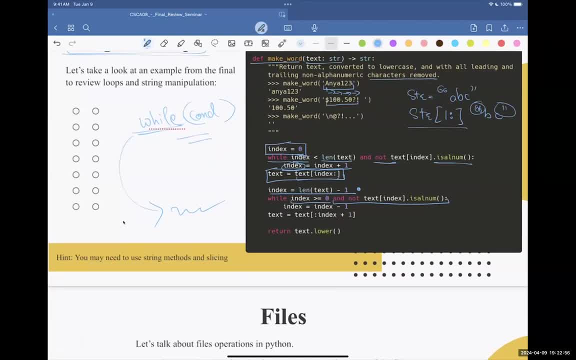 okay. so see, take this, take this example. we reach some index here, for example here, and this is the index which is the last index, uh, that we can consider, so it will be somewhere here. so, index right now is this. so, at this very point, our, uh, the text looks something like this: this is the text, the highlighted portion. 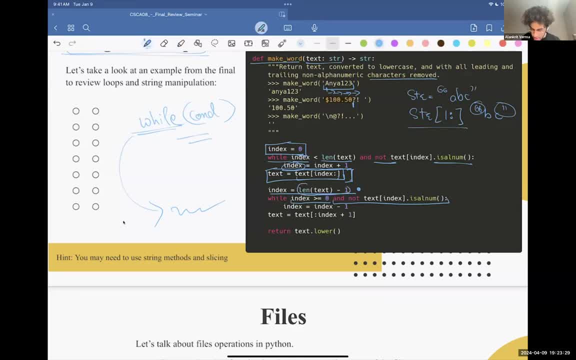 and then in the next part we are trying to reduce it, and then we end somewhere here and at the very end we are left with a hundred point five zero. what is gonna be your font name index stress is that makes sense. so what are we doing is, if we get- uh, 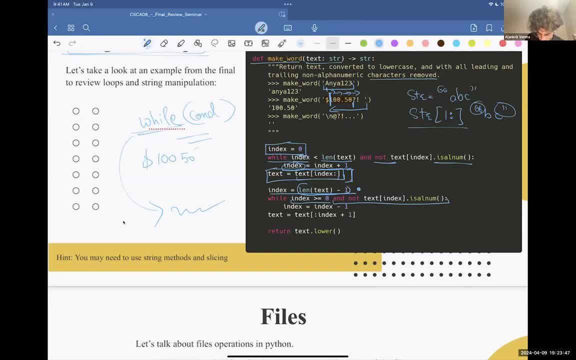 a string, hundred point five, zero question mark, and that this is the string that we get. we first try to find what is the last, uh, but in some sense, which one of this is the first one? so we find this here. so the text then is going to be: 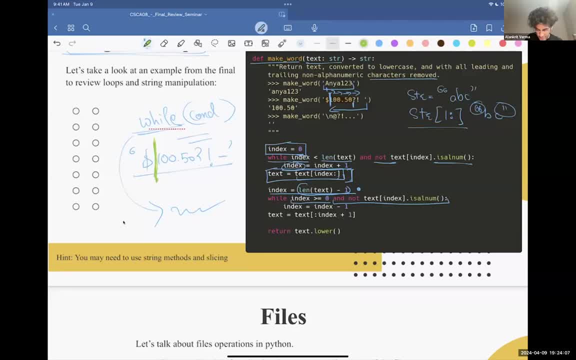 force box. so the text then is going to be: so our, our actual text is going to be five, five common form then. so the text is valid, we won't. and now we're going to take these into question mark with our canva like text. so we're filling these ingredients here like this: this is the very important part. these three recommend you it will take here. so the things which you can do in there, for example, are really the you get to the question mark. 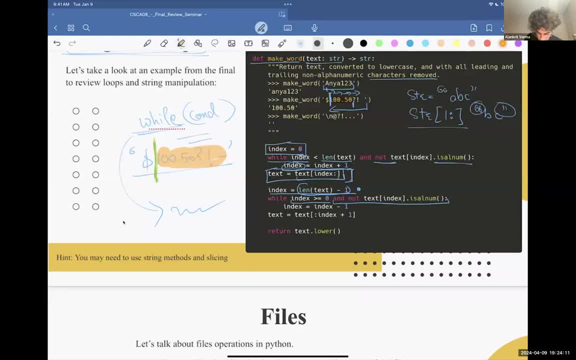 text then is this: we found the first boundary and then we start from the very last. we start from the very last and we keep on reducing the index until we found a, until we find a alphanumeric character. we start from here. is this an alphanumeric? no, it's just alphanumeric. no, it's just alphanumeric, no. 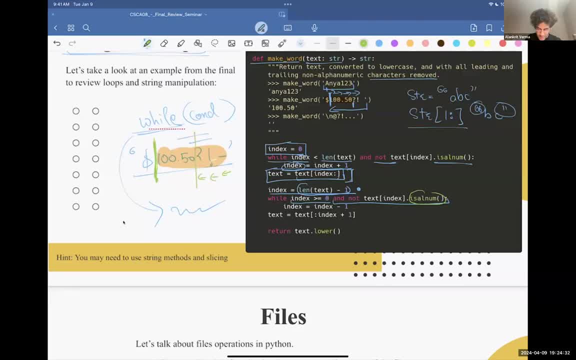 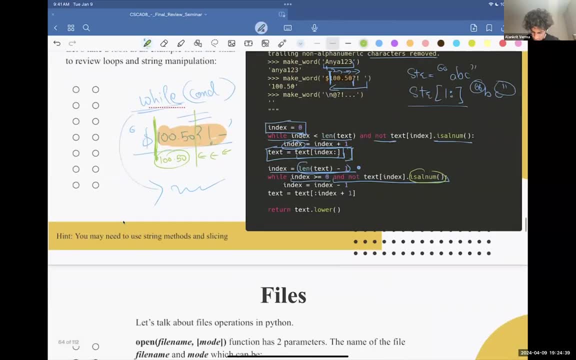 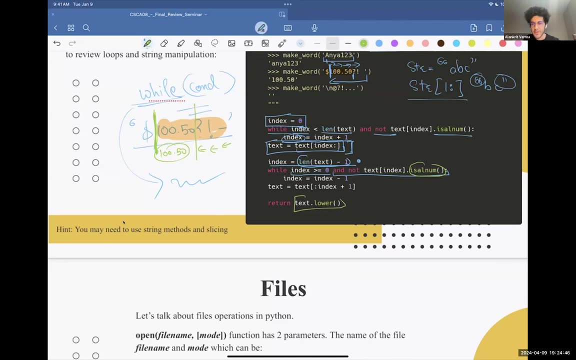 but if zero alphanumeric? yes, it is. so we stop here. so at the end, what do we have? we have 100.50 and we also need to convert all of them to lowercase, so we return this 100.50.2 lower. does that make sense? yeah, that makes sense. but what if we had something with an alphanumeric? 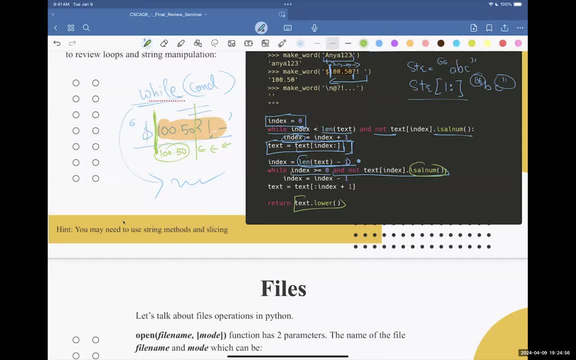 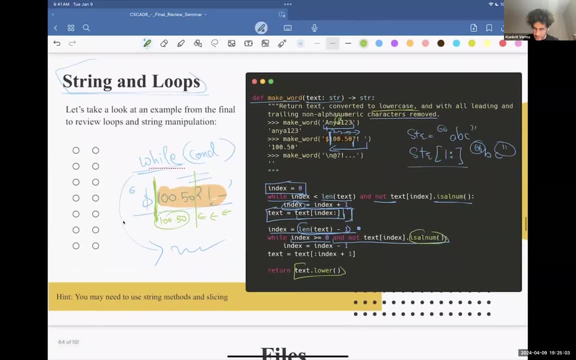 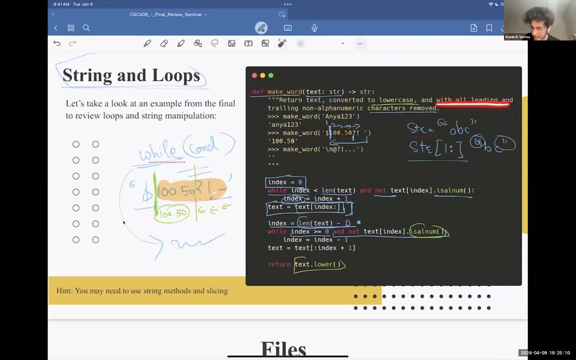 variable in the middle, like, for example, like the first one, like anya one two, three. had like anya at one, two, three, then would this still like work? uh, okay, i want you to read the question for that. so the question says, with all leading and trailing, non-alphanumeric, it doesn't talk. 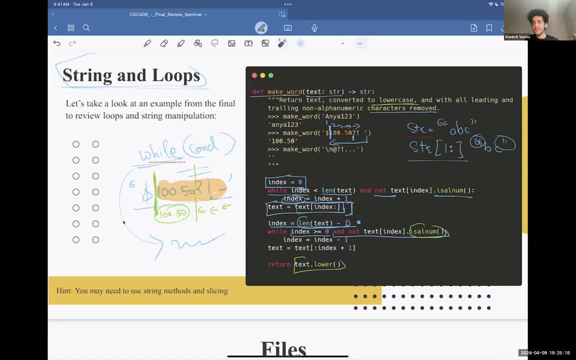 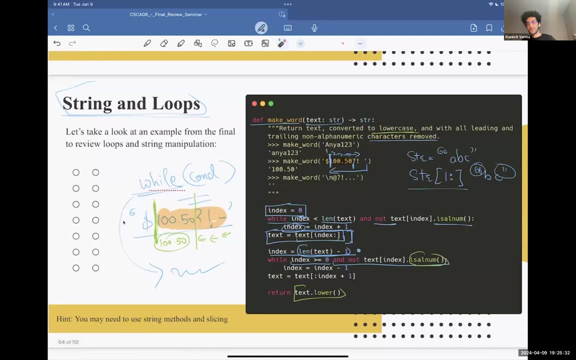 about the ones in the center. so if there is any, suppose at the rate you said this, there is a at the rate here that will still be present in the strength. cool, uh, is this clear? uh, any questions for the strings and loops? we just have one question. so this model is covered earlier through. 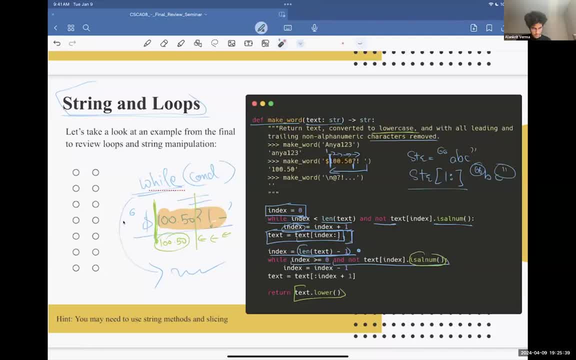 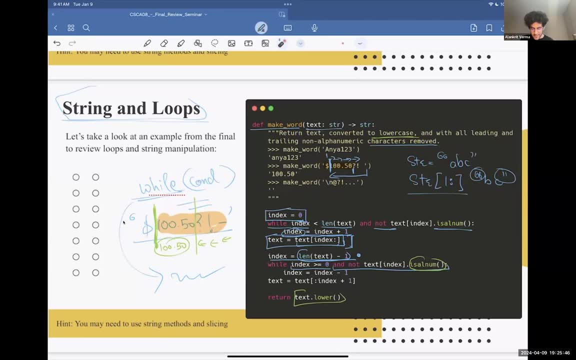 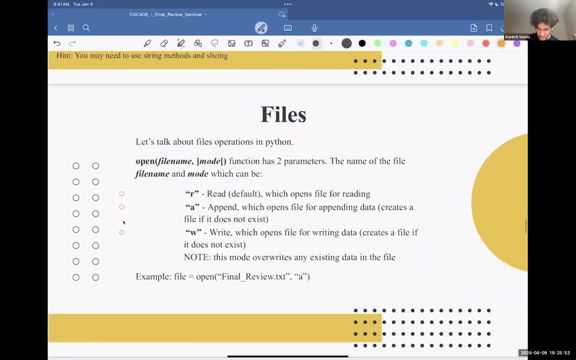 this problem. integration. this is your time. guys like: uh, we not necessarily want the same or similar results as the mechanism, so make sure you understand every single point. okay, if there's no doubt, and we'll move to the next one. the next topic is about files. so what? 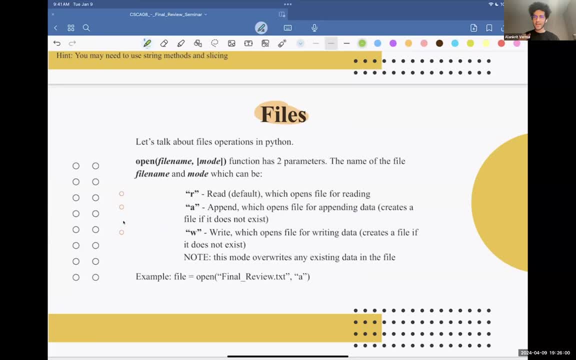 is the file, uh, in a08's language or in the language which you can easily understand and how I tell students who ask me is this? So, in very simple terms, a file is a very long line. It's a very long line with all sort of special characters. 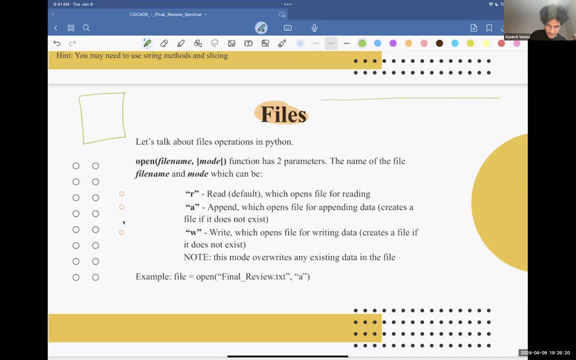 So if on notepad or on a text editor you're seeing hello hi, If you're seeing this, the actual file is something like this: This is a line, just a single line. So yeah, this is more or less how a file looks like. 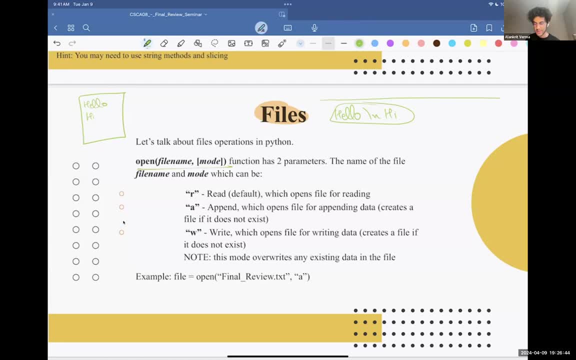 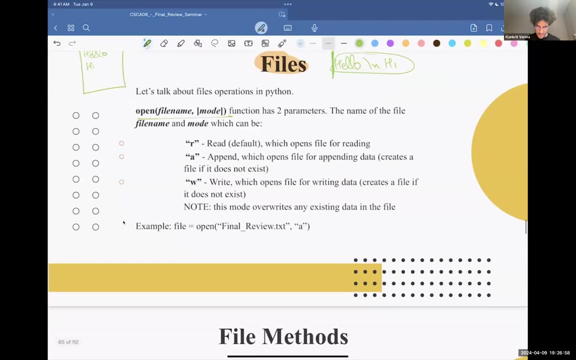 When you do open, when you open a file, this gives you a file screen in some sense, So a file pointer at the very start of the file, in some sense. yeah, And the bigger question here is: how are you opening a file? 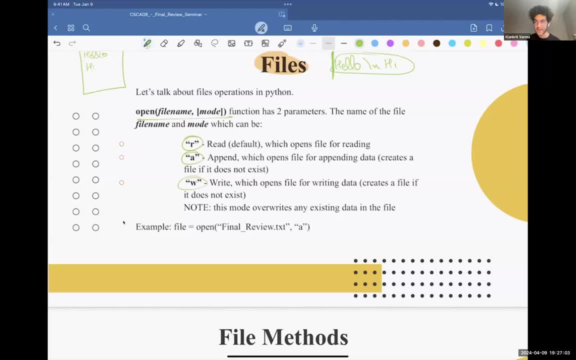 You can open it for reading, you can open it for appending and you can open it for writing. Now there's some cavities. I guess that's to it. This is pretty much simple And you probably have done this in A3.. 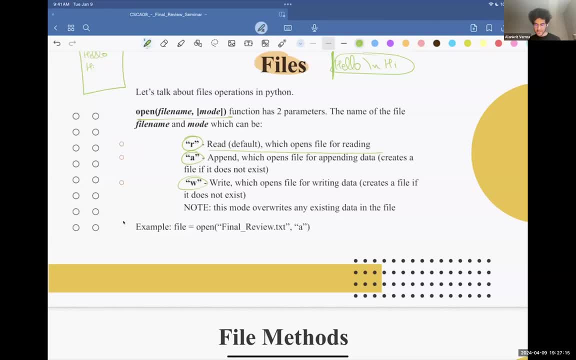 So I won't go over it, but just read it once for the next 20 seconds, And there's something you can't understand. please do ask. Cool, okay, I'm checking the chat. Does anybody want to respond? Yes, no, doubts problems what? 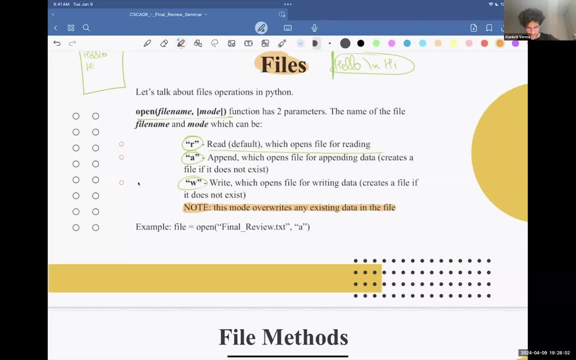 Okay, I'm waiting for the chat. r and w and a all open the file, right, okay? uh, the opening of a file is a bit different. as i said, open of a file is done by this function, which is the open function, and then, when you see, 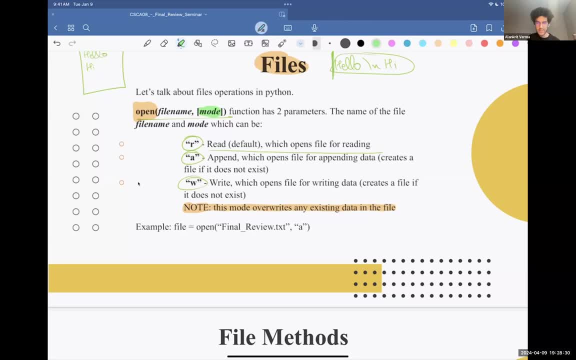 this mode. so this is the type as you want to open the file with. so all of them will open the file. but, uh, how you are opening the file depends on this, and open of opening of a file is not done by this mode, but by this function highlighted in orange. yeah, any other questions? no, we have. 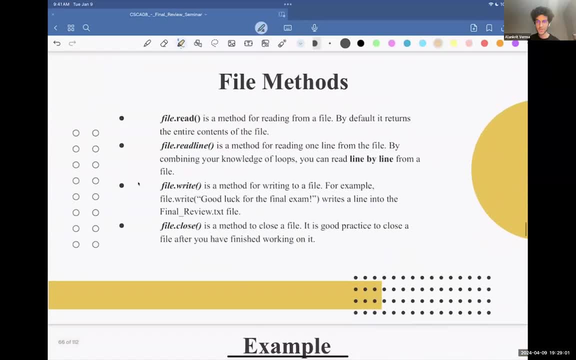 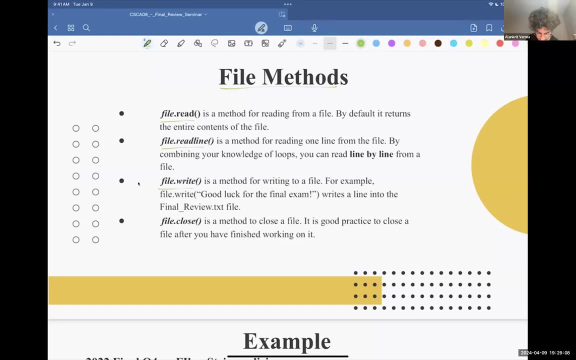 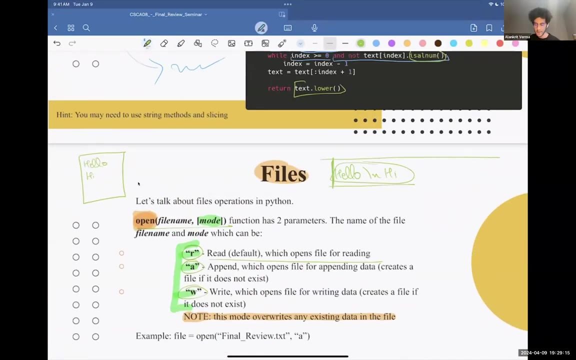 a total of 112 slides and we are still at 66, so we will try to be fast now. okay, file methods: uh, fileread, filereadline, filewrite, fileclose. so i talked about a stuff. this is a file, in some sense a very long line. what does fileread do if this is a very long line? 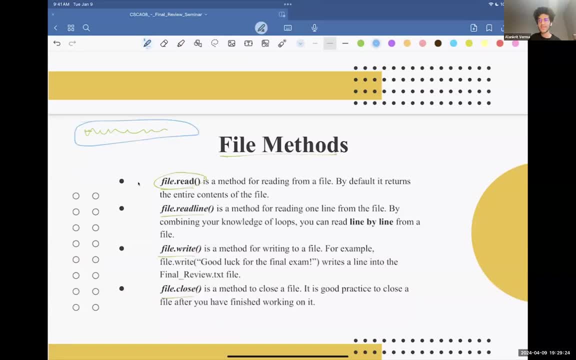 it will read the whole thing as once, so it will open the whole file as once. it will open the whole file as once, the whole thing. it's a method for reading from the file. by default, it returns the content of the file. okay, what is next? filereadlines is a method for reading one line. 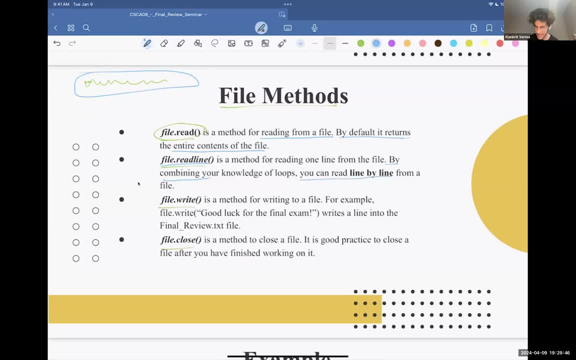 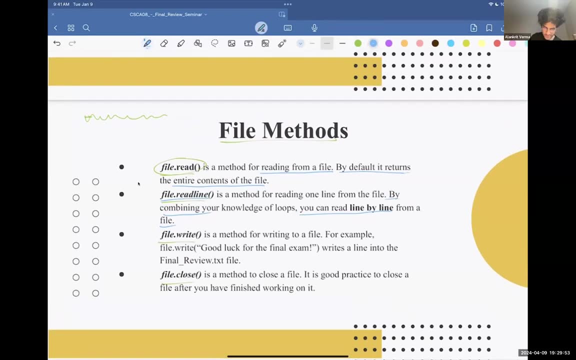 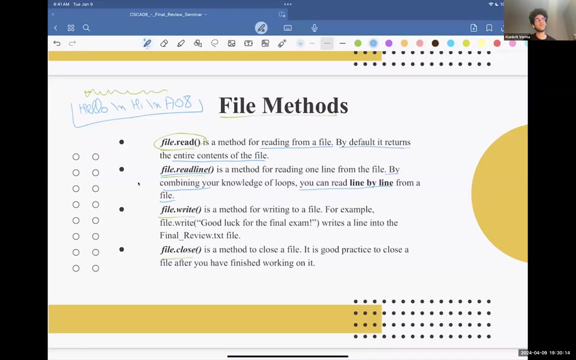 from the file. by combining your knowledge of loops, you can read line by line from a file. okay, so what is it? filereadlines if i'm having? i had that, um, hello back session, hi back session, oh wait. so, uh, if this is the file, what will filereadline return? one, when is it when? when this? 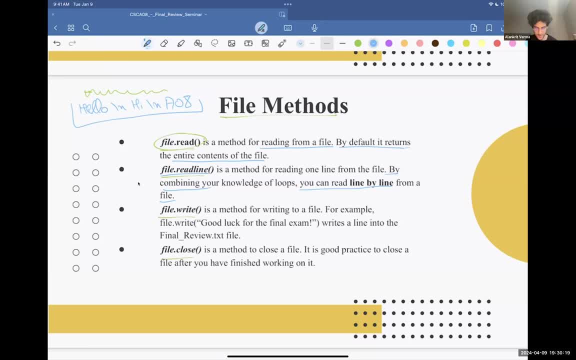 is done the first time, what will this return? filereadline- hello, okay. and what will it return the second time? okay, hi, i get it. uh, good. so how is this happening? so filereadline is having the pointer or cursor somewhere here and it is going through the text. 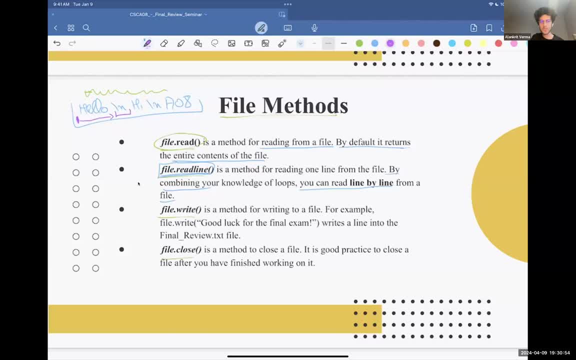 until it finds this backslash. then the moment it finds this backslash in, it will return this. the second time we do it the pointer is already here, the cursor is already here and then if we do file dot read line, it will go until a point. it finds this backslash: n until a. 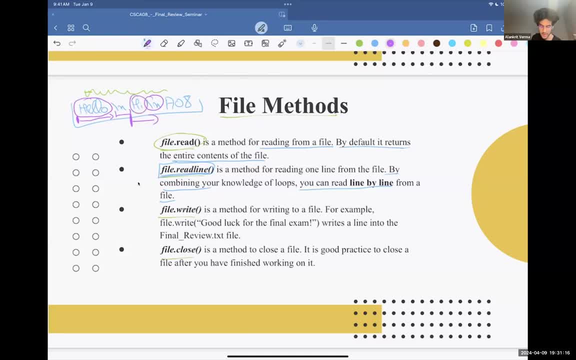 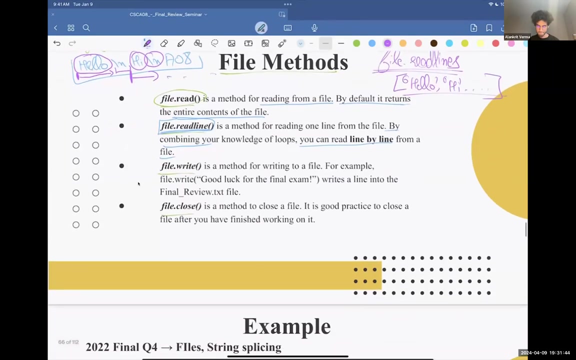 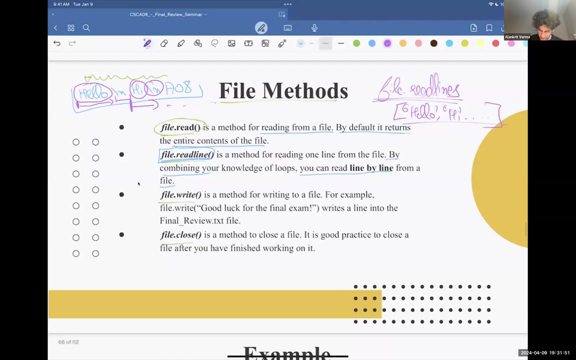 point. it finds this backslash n and then it will return file and then so, on note, there's also a function called as file dot read lines, which returns all of the lines in a file as a string. so that would that would be. this is hello, okay. so this is about reading. what about writing file dot write as a method for. 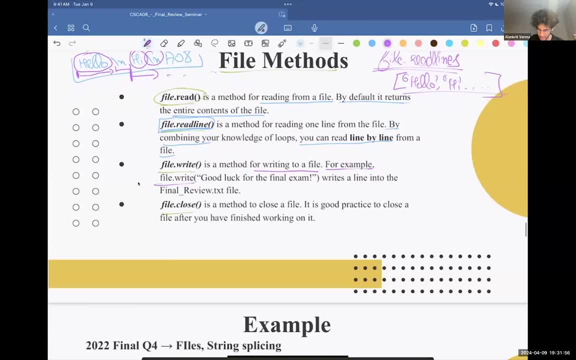 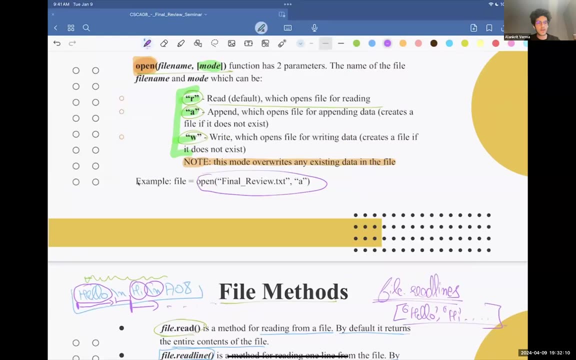 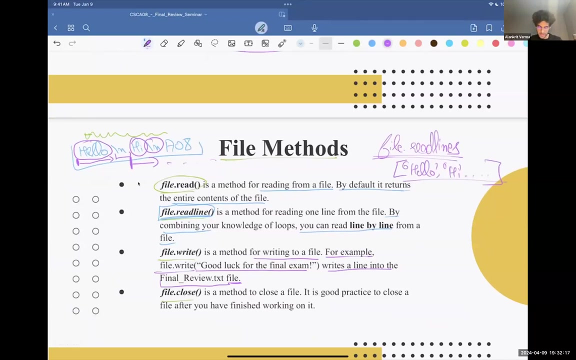 writing to a file, for example file dot. write good luck for your final exam. write a line into the final review dot text file, into the final reviewtxt file. so, finally, we had opened it here. and how had we opened it? uh, is it not? hello, slash back, slash n? okay. so a friend of yours asked: hello, uh would. 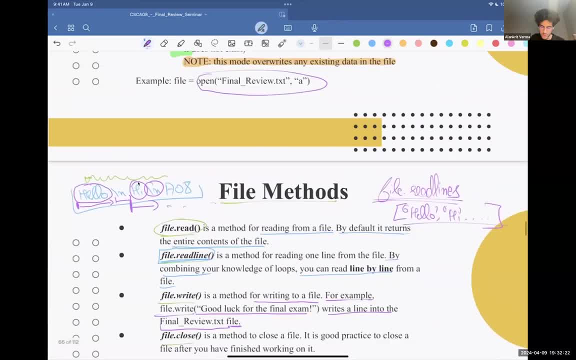 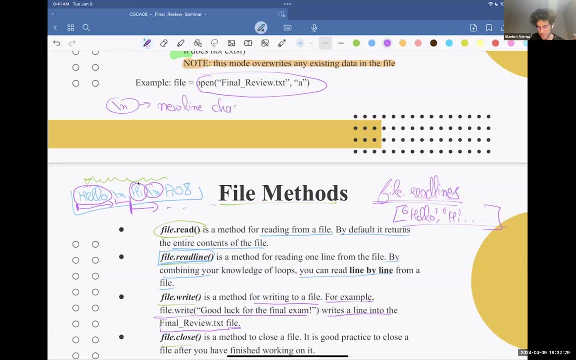 it not be hello slash, back, slash n. so the back slash n is more or less a new line character. this is a special character defined by python itself or the developers of python, which is used to segregate lines. as i said, in simple sense, a line or a file is a single line. 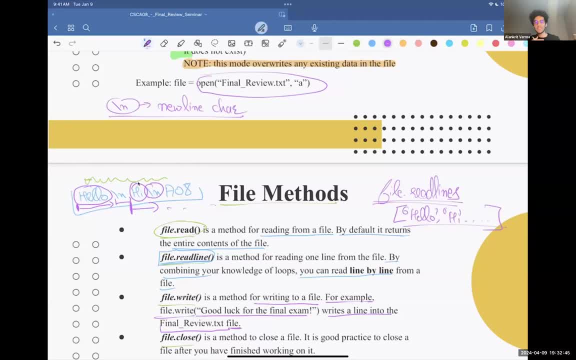 a single very long line which has all these symbols like backslash n and backslash n is used as a delimiter or a separator for these lines. so the question was: is it not hello, backslash n? no, because backslash n is just a separator, it's not part of the string. 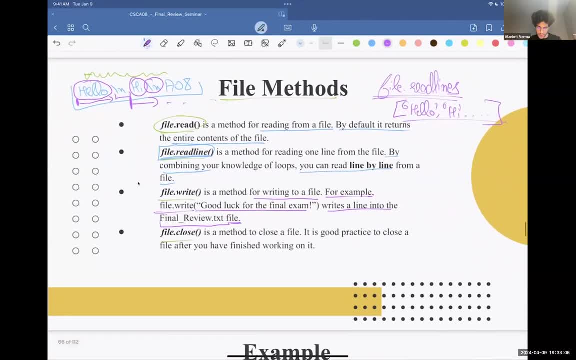 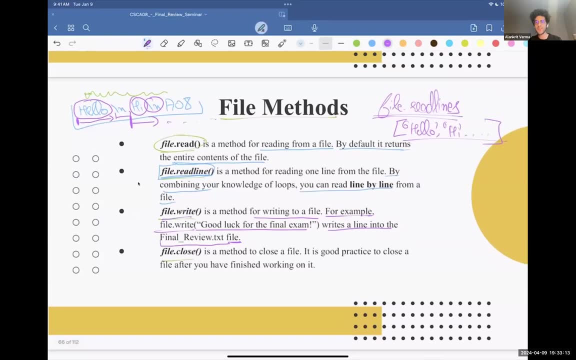 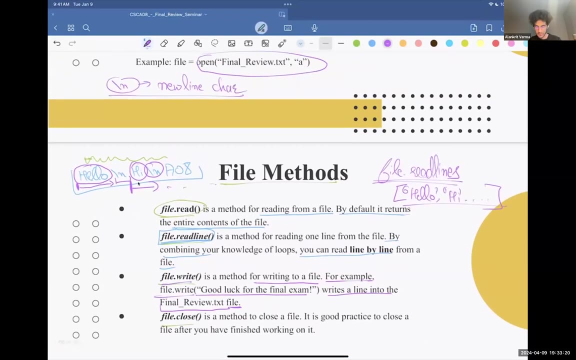 okay. um, then we have filewrite. now can anybody answer as to where will this write to the file? will it be at the start or at the end, or in the middle somewhere? okay, it's gonna be at the end of the file content because we had already written the file content and we had already written the file content. 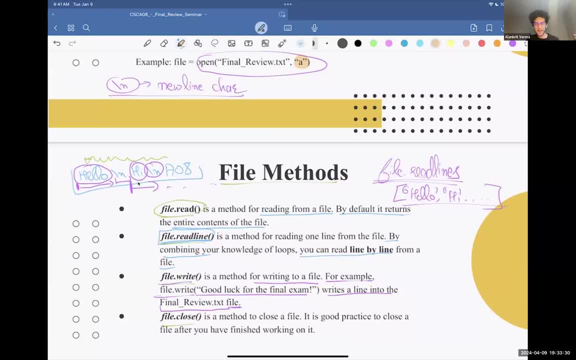 open it because we had earlierly opened it with append. if this was w here, then it would be from the start. if this is not w, then uh. if this is a, then it would be uh at the last character of the current file. so like appending to the current content. okay, fileclose is. 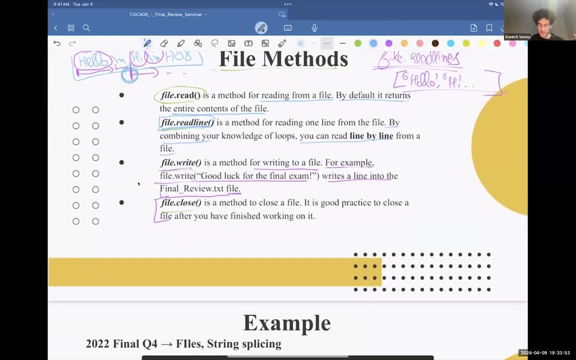 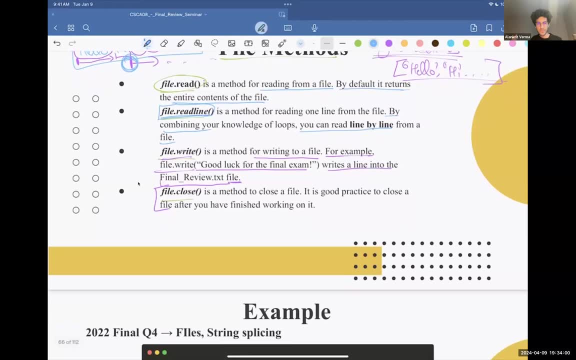 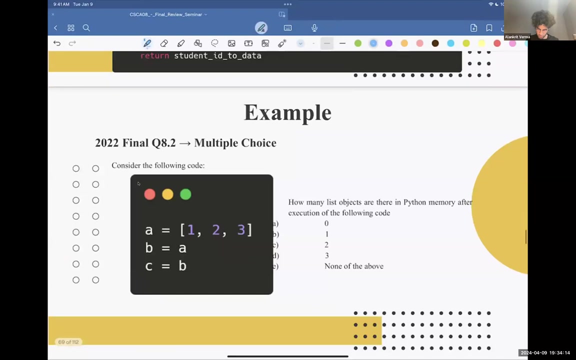 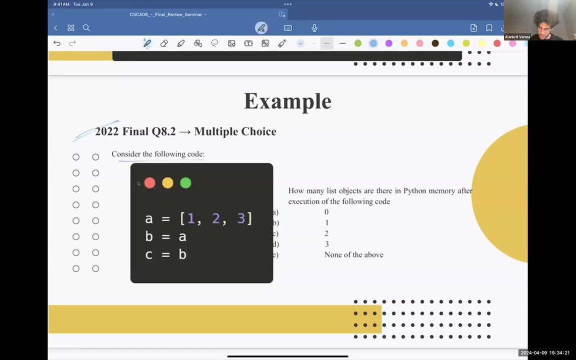 more or less deleting this pointer. you remember we had this pointer which is helping us move around stuff, so we don't want to keep this open forever and we would uh, return this file. we will delete the file pointer or like: close the file. okay, fileclose. okay, let's go over this. first, consider the following code: how many list objects are there? 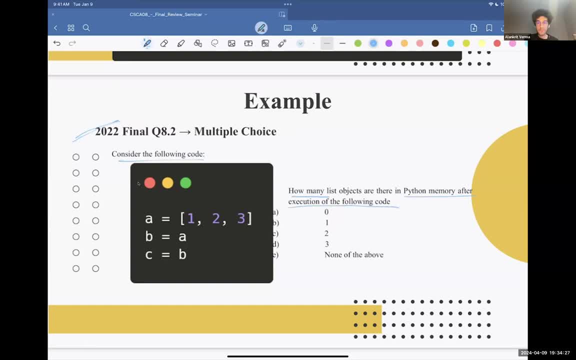 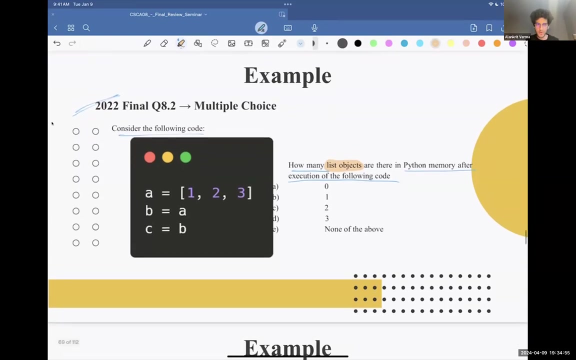 in the python memory after execution of the following code. consider the following code two: okay, let's, we can now search for a third variable if I just want to keepyears long until reading the full text report. ten seconds if anybody wants to answer the topic. a lot of people are saying one. there is a lot of people are saying one. 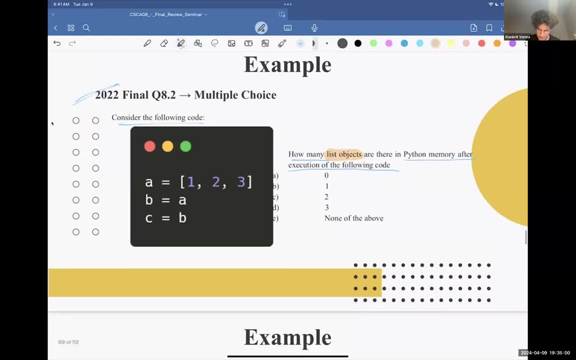 uh, no, it's not. it's actually one, um, it's not three. so what is happening here is, when we are doing, a is equal to this one to three list, this is initiating a list object for one, and every other time we are just uh making the other variables, like if a was equal to id1. 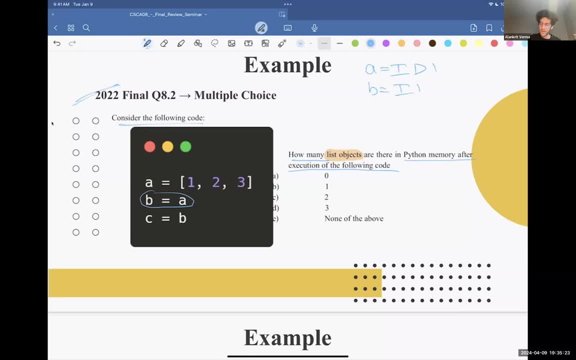 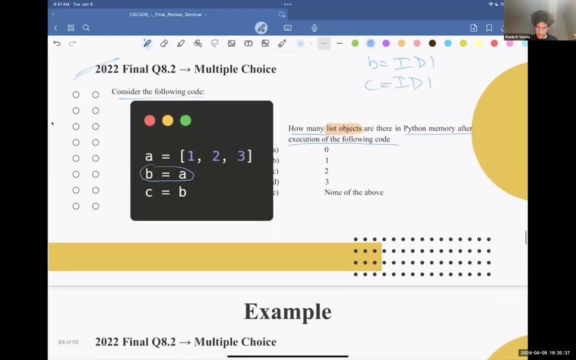 b also became equal to id1 and c also became equal to id1. it's not like we're creating those ids again and again. if you remember, we had something called as a memory model. uh, yeah, that's like an older topic. you should know this by now. 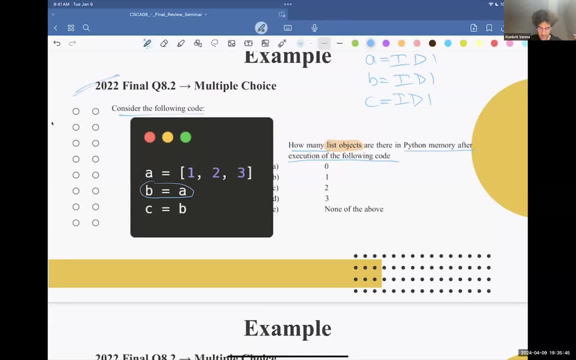 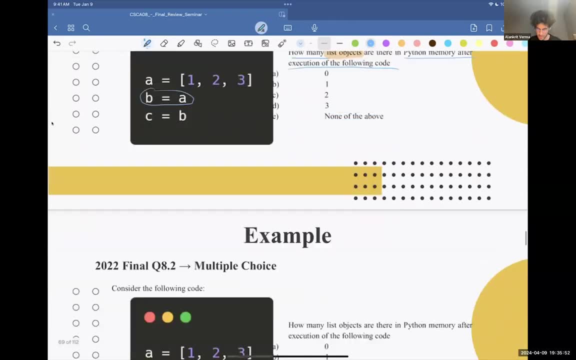 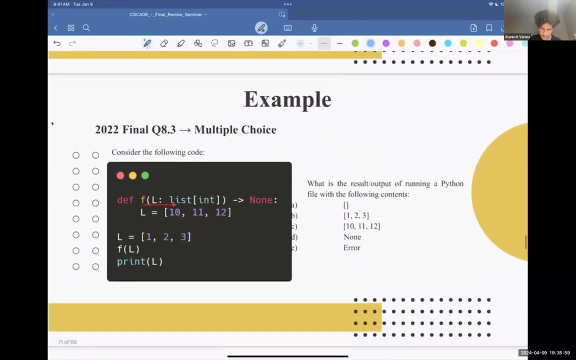 so we create this for the first time at a, and every other time we are just assigning the value of a to b. we are not creating it again. okay, cool, uh. okay, we don't have the answers- math here- but one is the answer actually. okay, let's see this. this is the following code: what is the output? 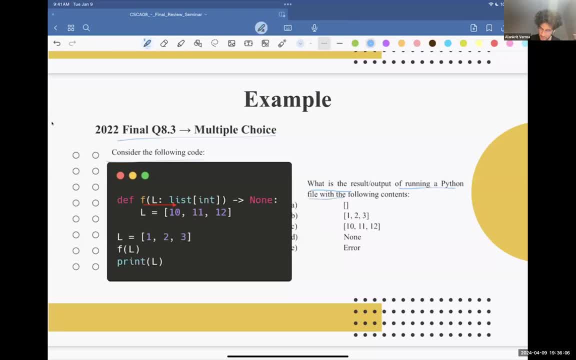 of running python 5 with the following content: 10 seconds. i want everybody to at least go through it. um, so, there's one percent. so, uh, there's dd coming in. okay, this is not. uh, okay, uh think mode. is this d or is this c? so, 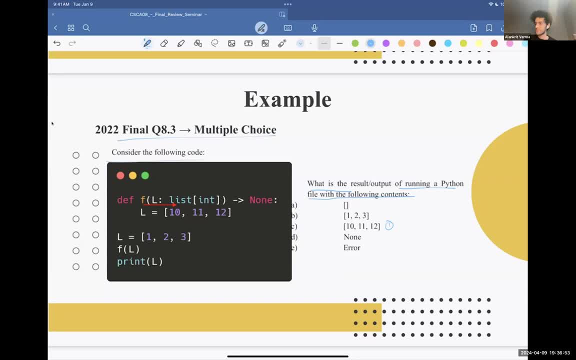 okay, there's confusion there, B or C. so you go, you start from here. so L is one, two, three, you go here, you go where, you go into the function. so you're here now. this is what. line 1, line 2, line 3, you make a new list: 9, 4, which is 10, 11, 12. 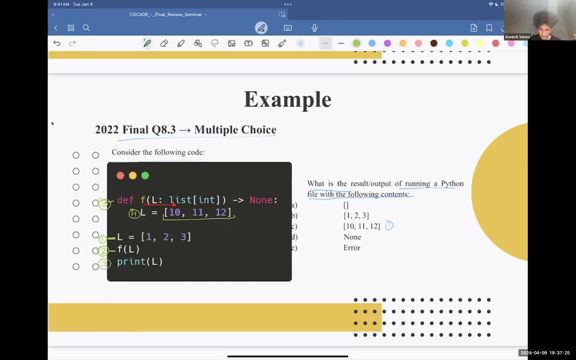 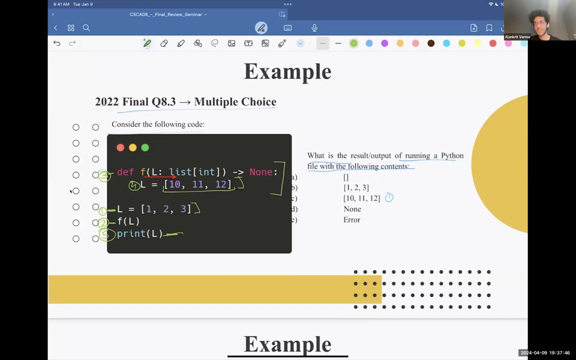 then you come back to the. so what is L at this very point? is it this or is it there? that's one of these two. okay, I think now people have time for it. the machine this week. okay, it is B, because when you're working in this very function, the memory of the function is local to itself. you're not passing a. 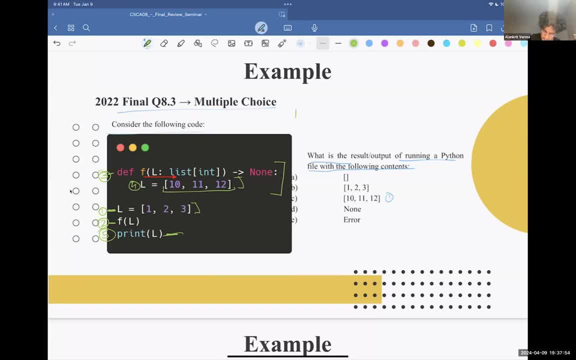 list like that. for example, if you would have something like here, if this was: l at 0 is equals to something like 1, then that would change things. but right now, when this is saying l is equals to 10, 11, 12, this is creating a completely new object. 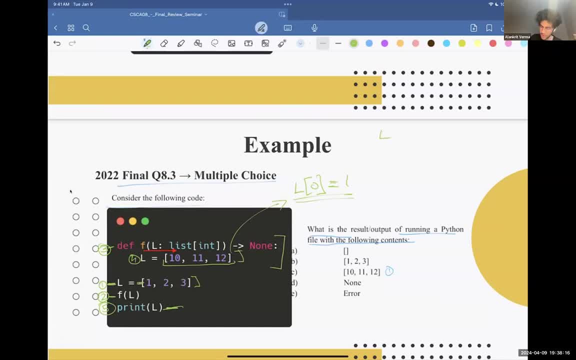 so earlier when we were here, l was having id1. then we went in the function and then l got assigned a new id. the l got assigned a new id which was id2. why did it get assigned a new id? because of this equality or equality assignment. 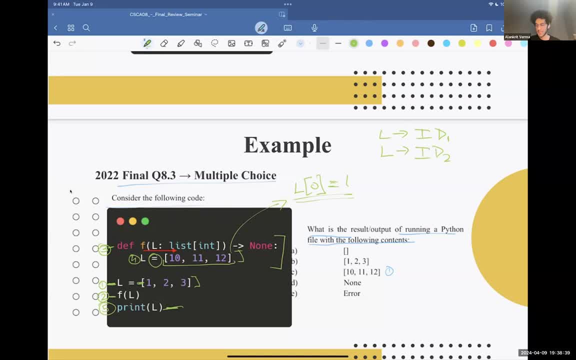 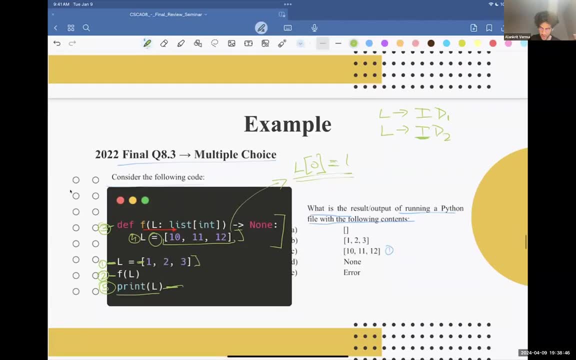 operator. sorry, this assignment operator created a new list, so then that becomes id2 and then you're back at line five and then you're trying to print l and this will always print which l this is. this line will always print this l always. the trick would be: 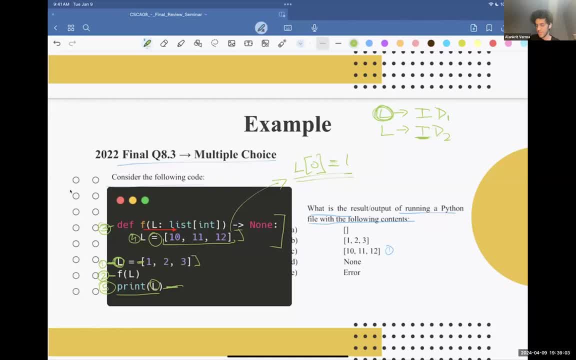 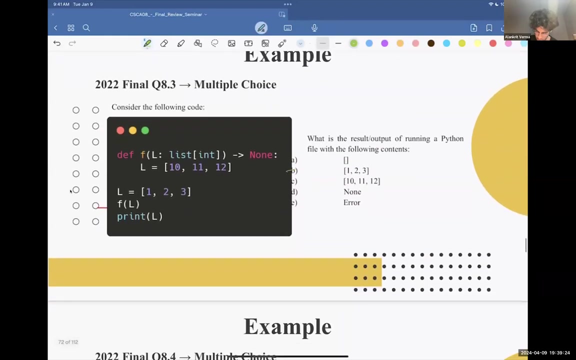 if this very l got changed itself and we change the values in id1. this is a bit confusing. this is also, you know, i'm not wrong, but yeah, is this clear now? finally, i hope so. if anybody has any questions, please do ask now. okay, uh, assuming not, this is the correct answer. 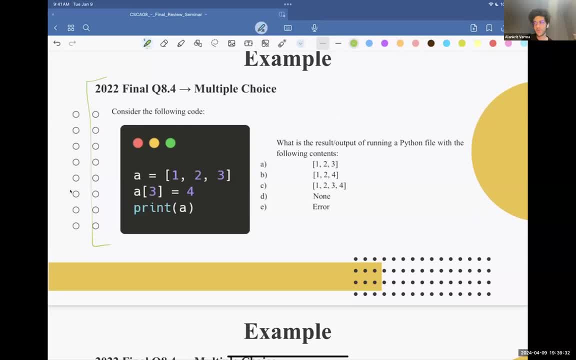 yeah, what is this? five seconds. we're gonna be quick with it, so i need three more uh answers and then we'll move on. please be quick, okay, okay, okay. i can't wait more. this is gonna give an error. why will this give an error? because we're 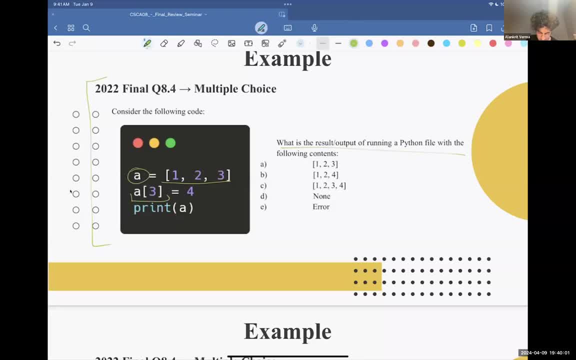 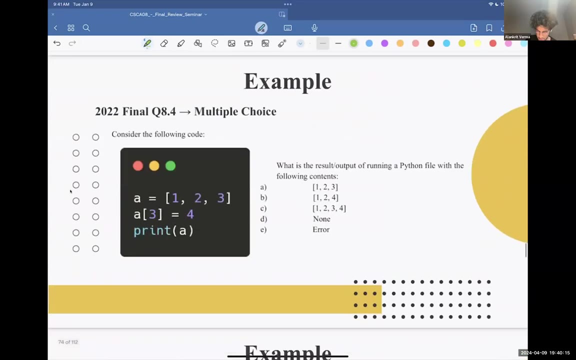 having a is equals to one, two, three, and then we're trying to access three, so a is having zero, one, two, because these are the indexes. there is no third index in this. so this will give an error because to access something which is not already present. so error is there, right? okay, because of the time. 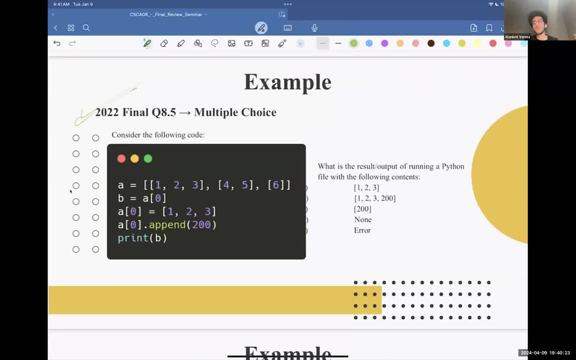 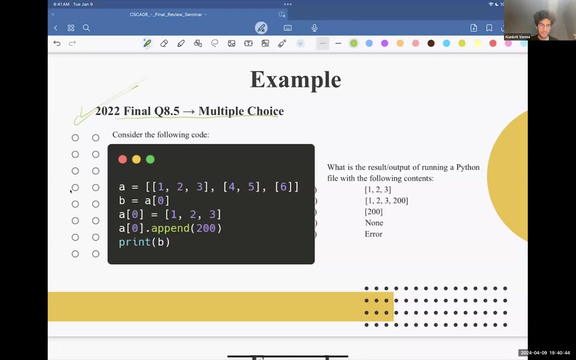 next question: these are all past paper questions, which means we are very similar to the ones you'll probably have in your family, so take them seriously. you yeah done. what is the solution for this one? anybody? okay, we are getting b and c. think, think, just think before you write. this is a good one, i guess. 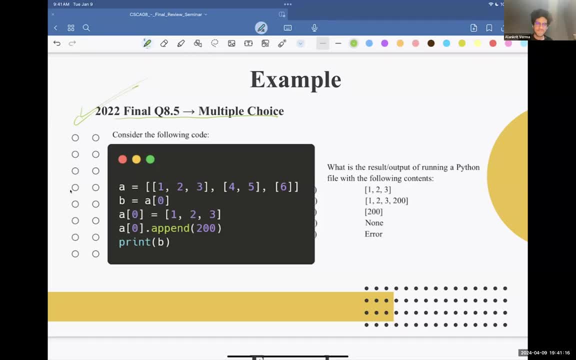 somebody said a. okay, people are saying a now. okay, some people are still on b. think this is a good one that i'm spending time on this. consider the following code: what is the output? so this is a line one. we initiate this. okay, initiate this line two. 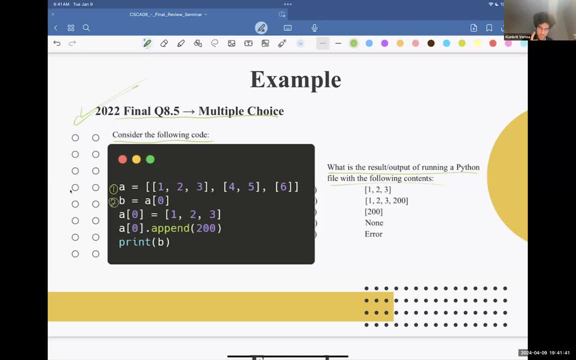 we change. we change the value at index zero in the lift of a. no, i'm lying. we change the value at index 0 of a, which is this now, and then we append 200 to this. to what? to a? so now i need some. they can't comment on something like b, so we just we have to. 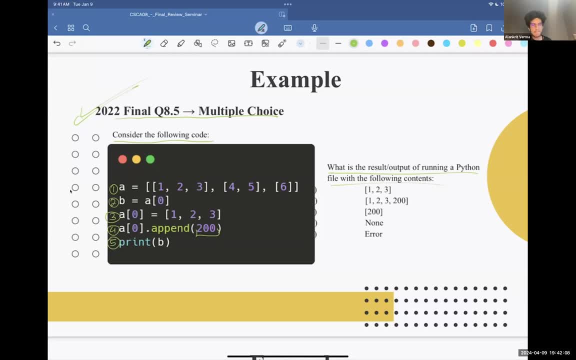 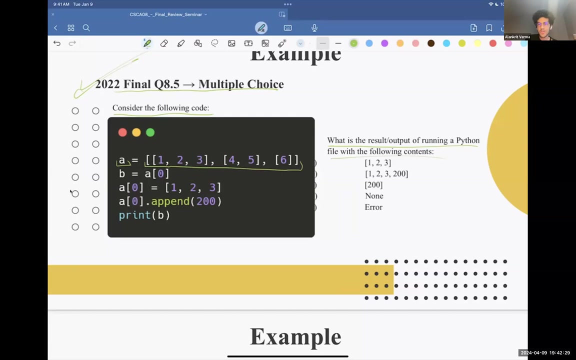 break this one. in subBER we can't comment on anything, but you can'taran the last one. let's let this be the deciding factor. world is the solution for this one? storing these lists as lists then we make. uh, b is equals to so if a is having one, and then this id1. 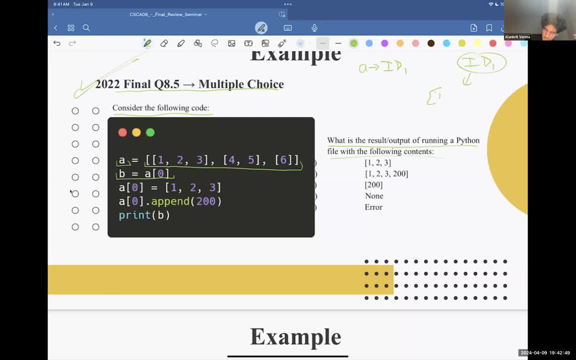 here is storing a list of id2, id3 and id4. what did we do? we made b is equal to id2. we made b is equals to id2, the first element in the list. okay, that's fine. what do we do next? we took a 0 and we changed it. we didn't modify it, we assigned a new id to it. so then what happened? 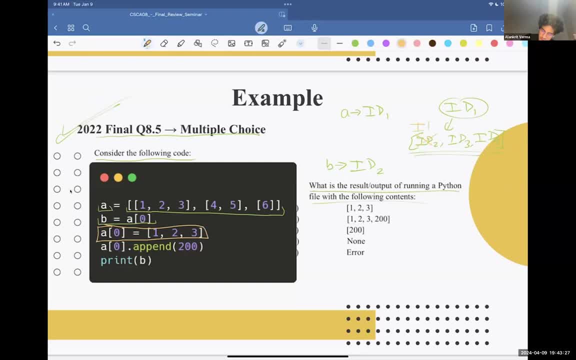 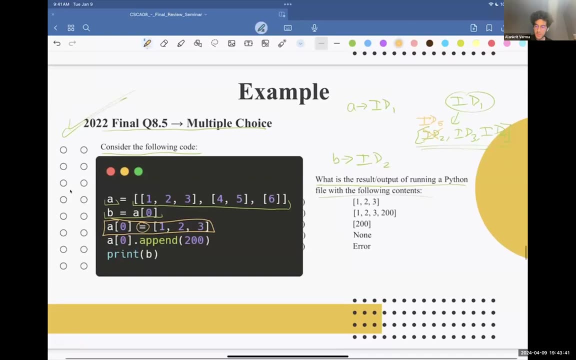 this id changed and this became id5. why did this change and not modify? because we were using the assignment operator. we were using the assignment operator, okay, uh, so this changed here. this remained the same. id1 still remains the same. we're not creating a new id for a. we're just changing the id for the list in the list. 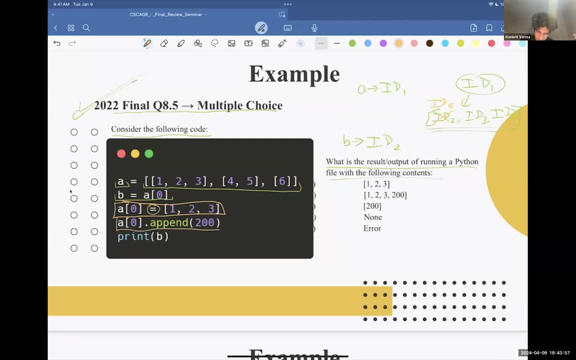 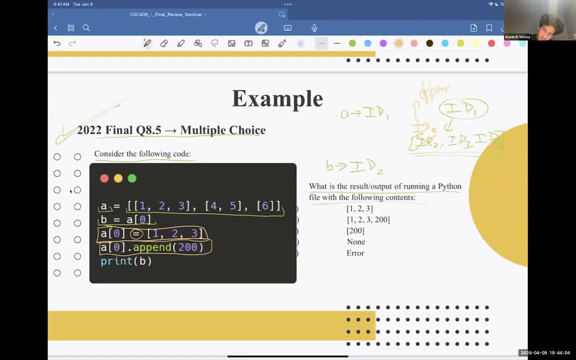 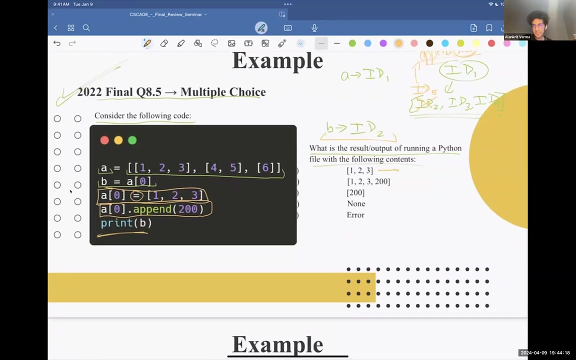 what do we do next? we appended this with 200. so what is being appended? this one is appended with 200, and then we're saying print b, but b is still id2, which was not appended. how will you modify it? okay, that's a good question. uh, so the answer for this is this: how will you modify it? so can you see, i did. 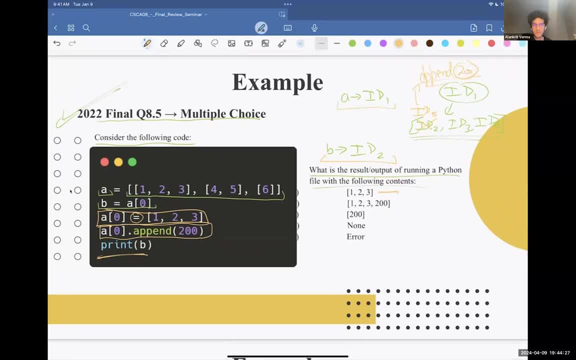 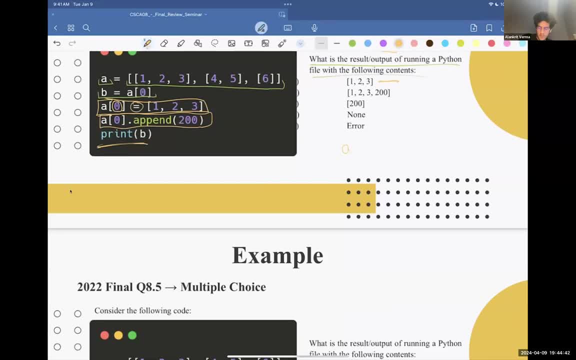 so you have a dot like: basically, a is equal to some. uh, you can like, if you, if you do something like this, that would not change the value or id of a but will only change the actual id inside the list and that makes sense. so the actual id of a will remain the same information. 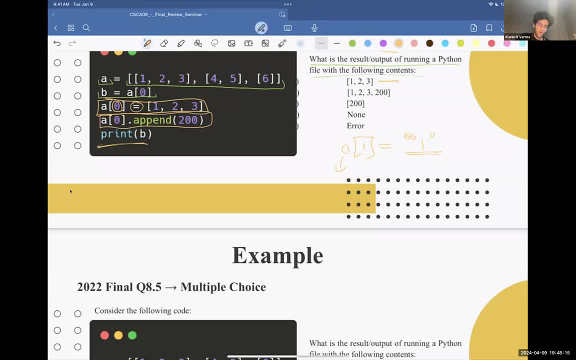 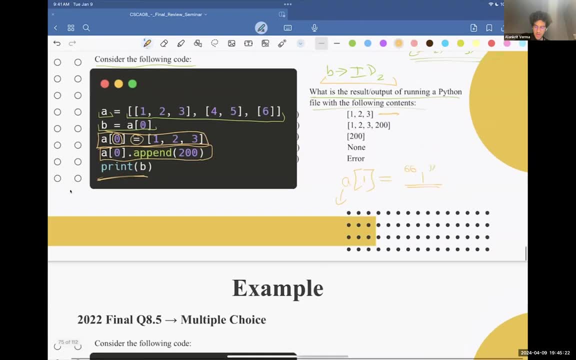 that answer your question. on a generic note, what happens here is, if you are using proper python functions- python functions- then the value is modified as and it's been changed. but if you're using these equality operators, then this is actually changed. why there is a different id? 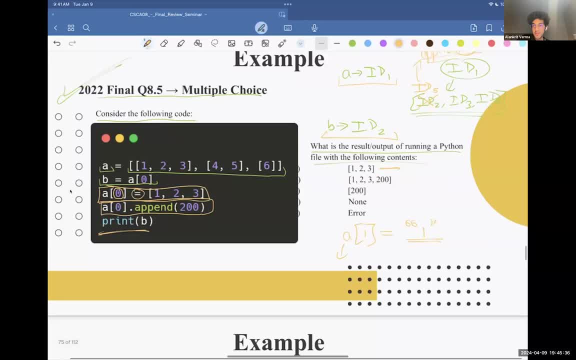 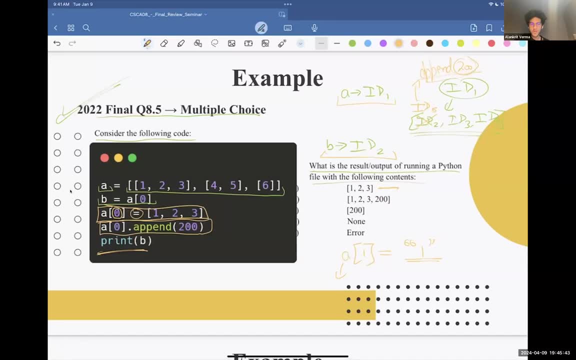 with the same value. okay, uh, why there is a different id with the same value? that's also a nice question, uh, and my counter question to you is why there can't be a different id with the same value? the id don't have. um, in some sense a value is not corresponding to an id. it is an id which is. 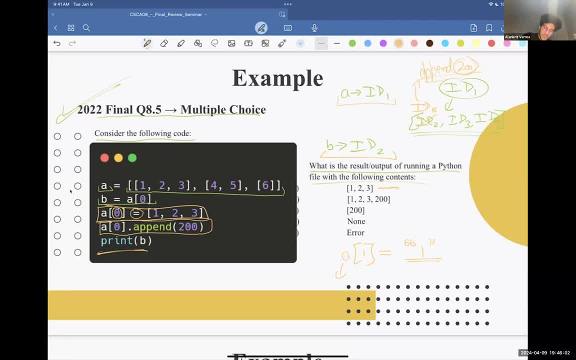 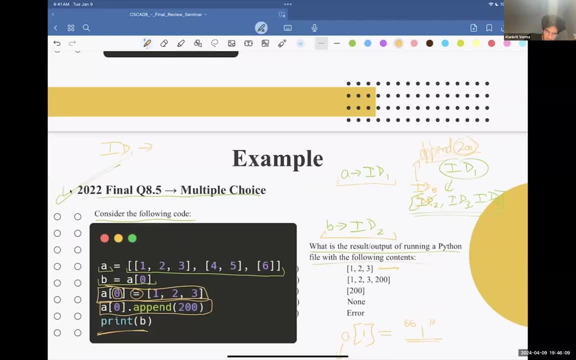 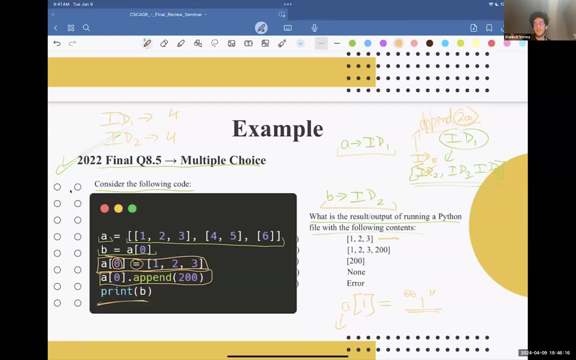 corresponding to a value. so this all right. so if this is id one, this is number four. id two can also have the number four, and these are completely different from each other. they don't have to relate the numbers and the terms they are using. they have to relate the terms and the terms. 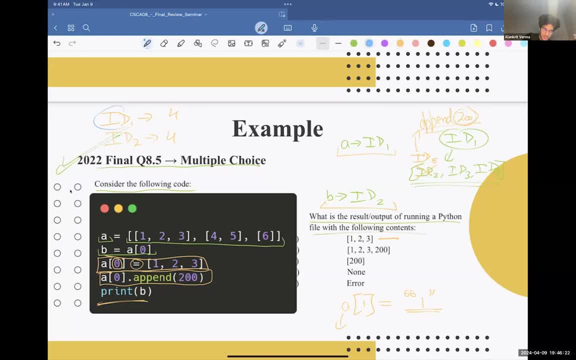 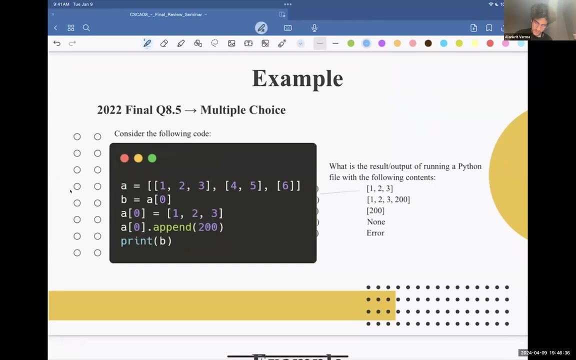 relate to each other, because the program deals with this. it doesn't care about this thing, it only deals with id. so, yeah, more or less this is just a convention that they have made in a very big picture. okay, we need to be quick guys. so, yes, this is q1, and then 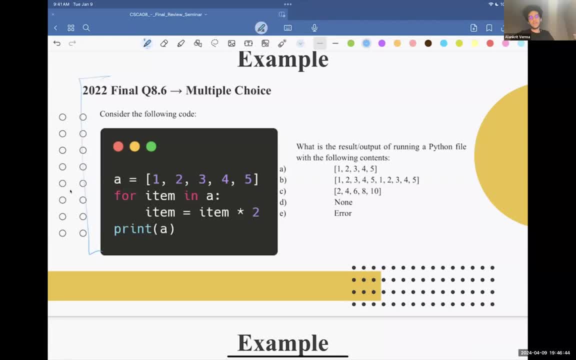 this now. i want everybody to answer this correctly. you have like 26. okay, there's one guy from a another person. okay, yeah, this is the correct answer. okay, i think everybody got that now. yeah, okay, i'm moving on to the next one, because i think now you guys have 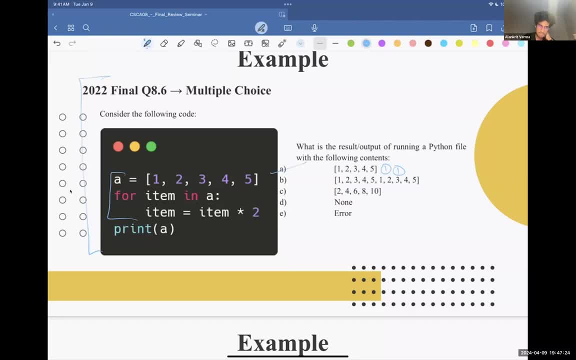 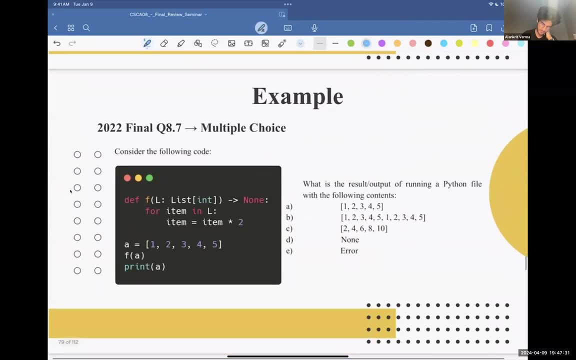 properly understood what is happening. okay, i think everybody got that. yeah, this is the correct answer. yeah, let's go on to this. what about this? if you guys have any doubts, please do just unmute yourself and ask it on spot. okay, somebody said c and then somebody said a. i don't know, people are saying c, okay. 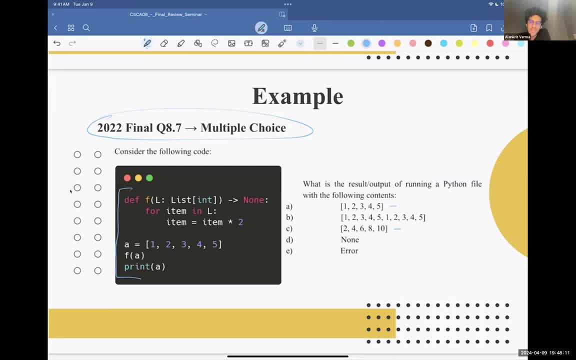 think, think. what is this? is this a question equal to? is this creating a new id or is this changing the id? is it actually changing the id? what is it, guys? is it creating or changing the id? it is creating a new id. the equal to always creates a new id. we have been discussing this. 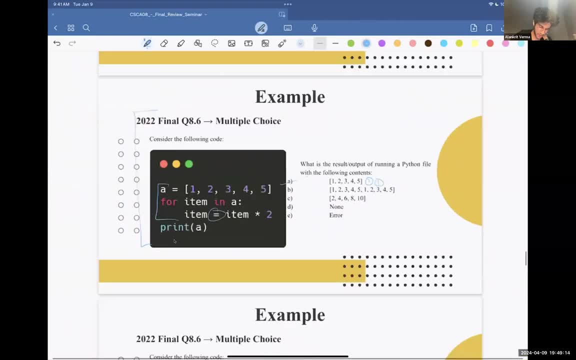 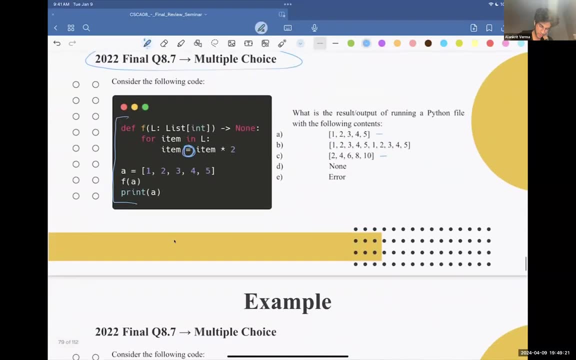 since this uh equal to create a new id. uh, equal to create a new id, equal to create a new id. so it always creates a new id. so when you're changing this, this will still remain the same and what i told you earlier: when you're printing a, this will always print this thing. 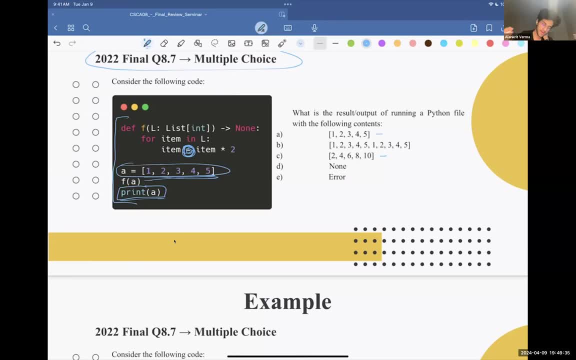 if this got changed in the middle, then there's a, then that's a different case, but in this case, uh, it did not get changed, because every time we try to change it, we created a new id for that. so this is the original zosten in the theme. okay, so this is gonna be 123.5. 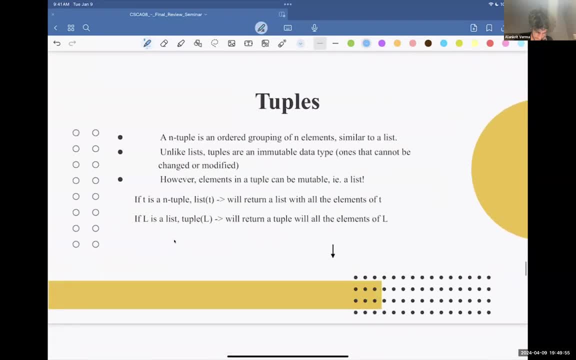 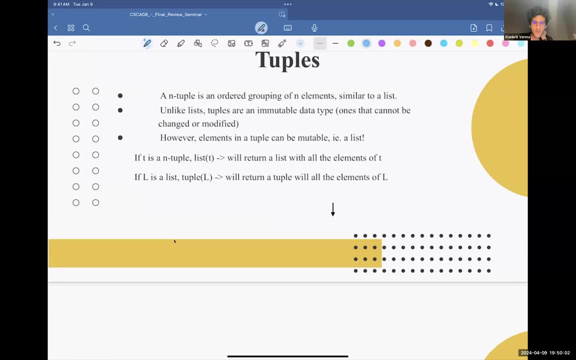 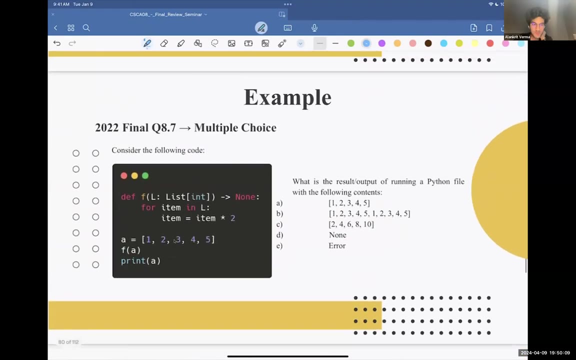 any doubts in this one? no, uh, yes, no, can see reactions. by the way, if you want a reaction with hyloblock and mustache cryo, no, so this is going to be 123.5. uh, yes, no, okay, and that's it. let's see you guys next time. 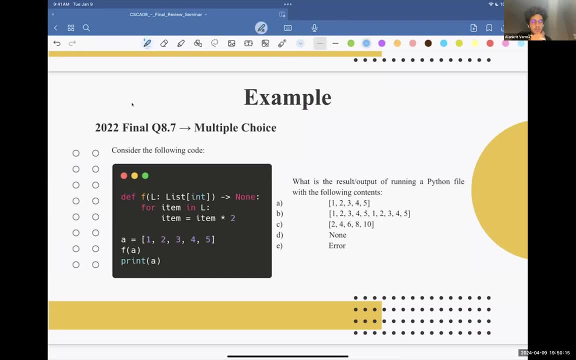 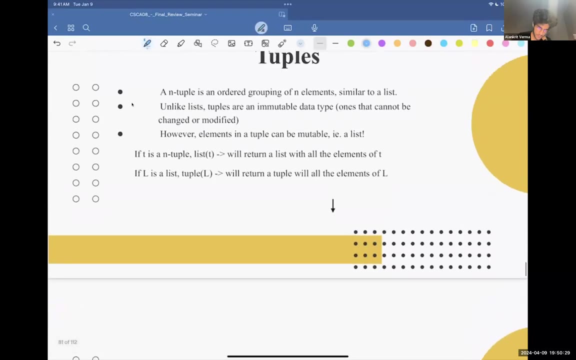 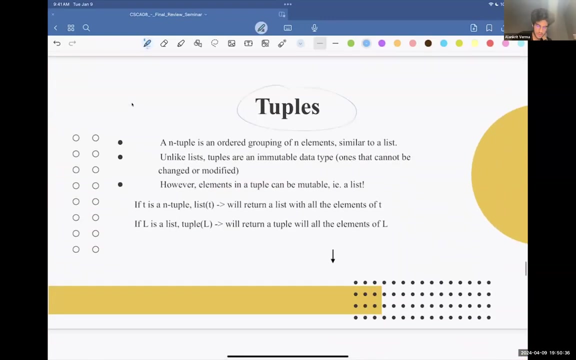 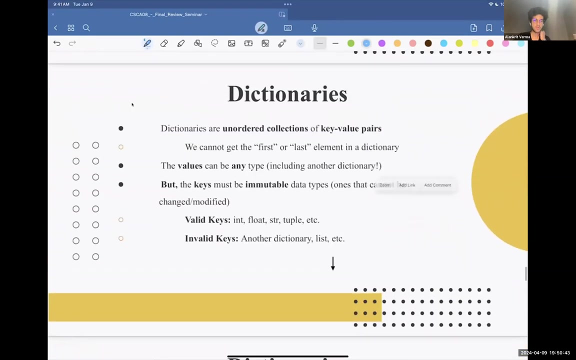 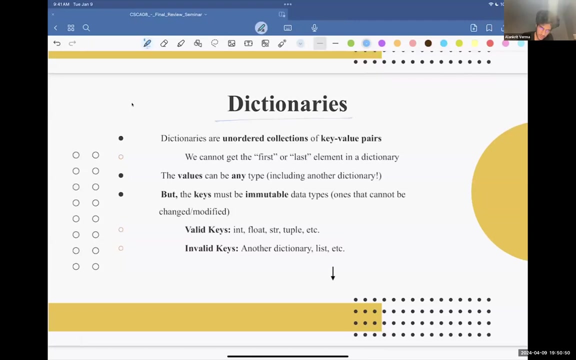 uh, yes, you are type. if you want to interact, type it in the chat. there's some questions about the couple. we will go over this. but I want to cover the other stuff. but this, yeah, the questions about the tuppers and take that are later on. let me cover dictionary first. wait, did we did a dip? 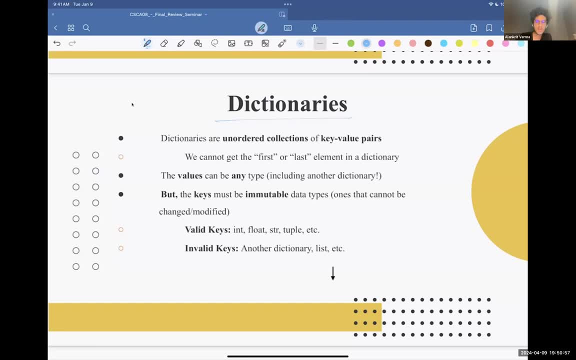 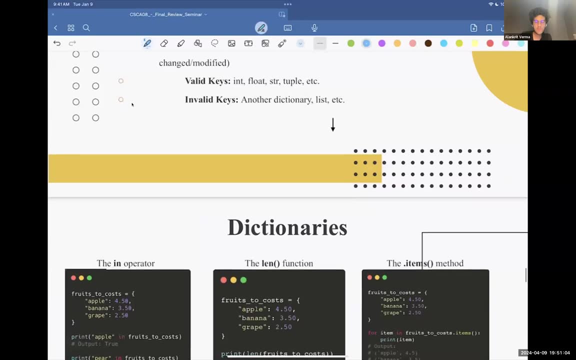 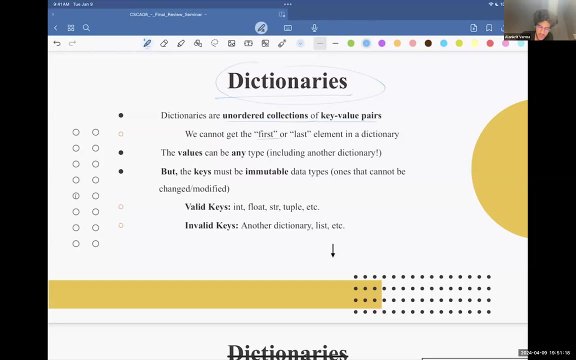 cover dictionaries in the last hour. anybody just confirm that? yeah, only briefly. okay, so dictionaries are unordered collections of key value pairs. we can get the first and the last element in a dictionary. the value can be any type, any type including another dictionary, so you can have a dictionary in a dictionary. 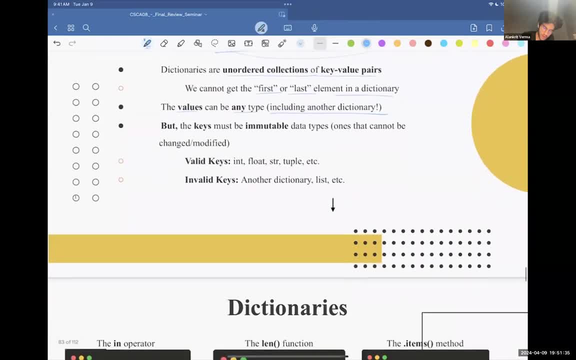 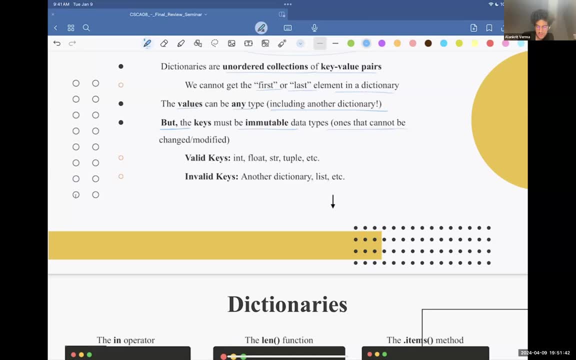 like infinite. yeah, we can go on. okay, that's one thing, but the keys are immutable. data type one, one that cannot be changed or modified. yeah, this is basically just a Szeneburg. immutable means valid keys are int, float, sings, couples, etc. and invalid key that another dictionary, lists ticket. you can't have a list or another dictionary. 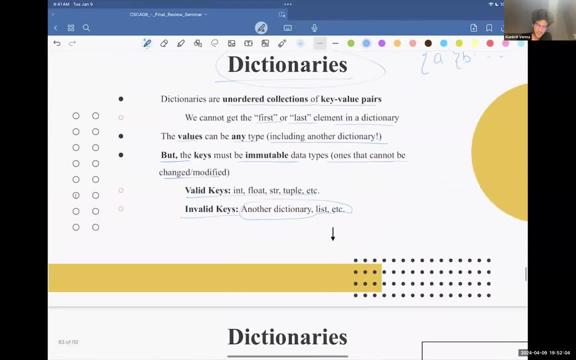 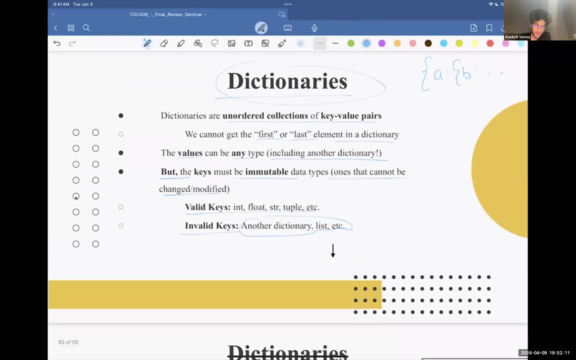 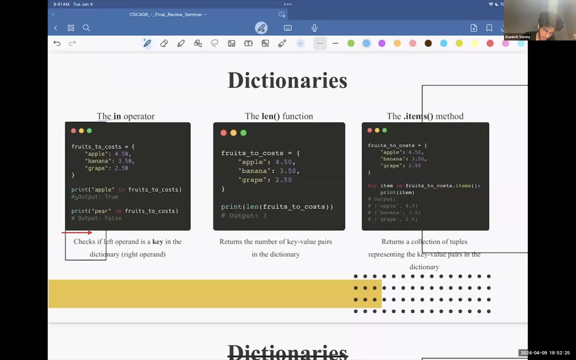 as a key. this is easy any doubt in this time and other sense. is everybody clear? clear with this term, the general introduction. okay, assuming that as a yes, let's move on to some functions with dictionaries. so we have the in operator, the length function and the dot items method. so the in operator checks if a. 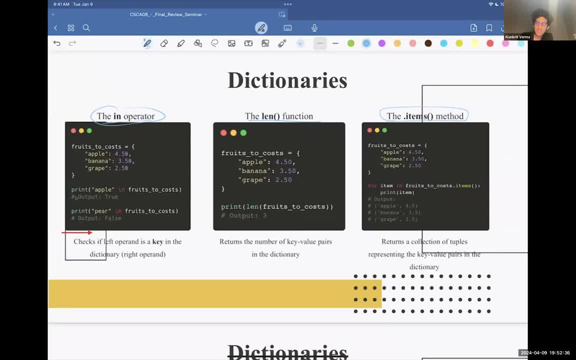 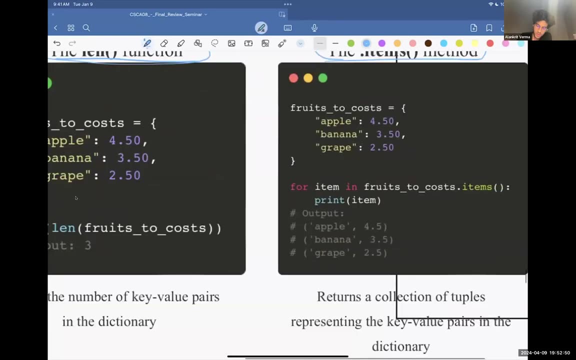 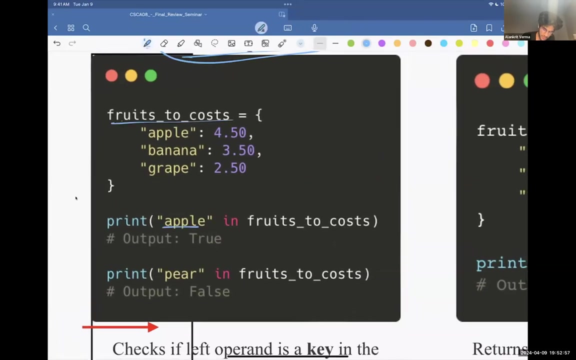 particular key is in the dictionary. the length of the length function gives you the length, the number of key value pairs in the dictionary and the dot items method is something used to loop for all the items in the list. so we go to one of them, truth cost, through truth cost, and I'm doing apple in truth to cost. 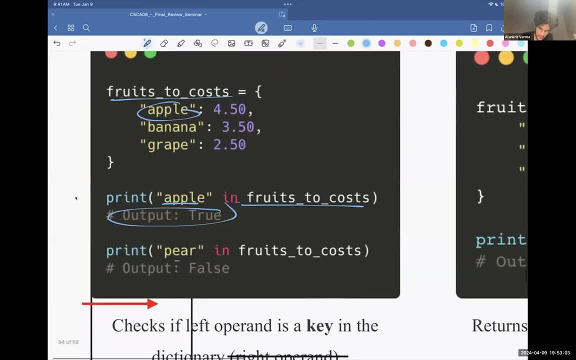 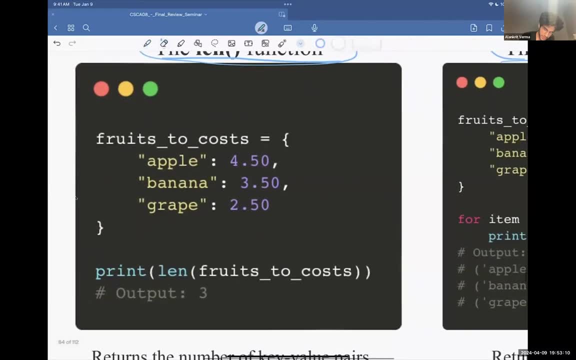 the answer is true because this thing is here. if I do peer in truth to cost, the answer is false. okay, then another function is okay, then another function is: this is a dictionary and I'm trying to do length of truth because this will return me the number of key value pairs. This is first, this is second, this is third. 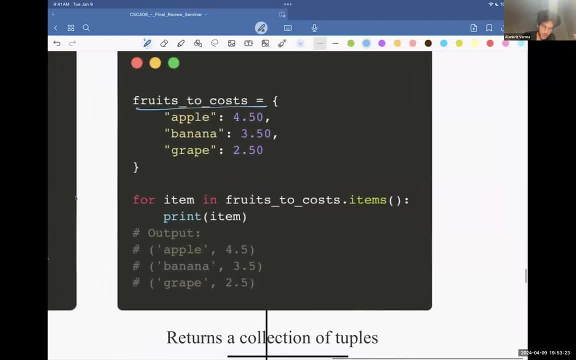 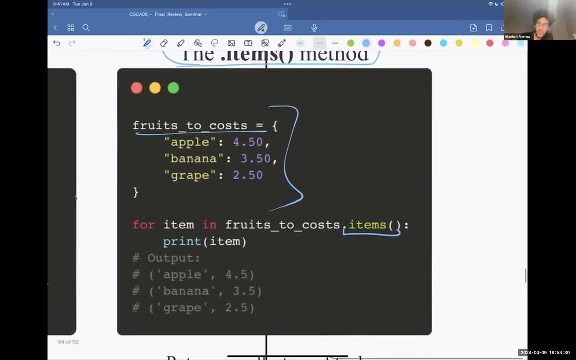 So output is C, Another one is truth: a dictionary, and then I'm looping through all the items in the list. So you can't really loop through a dictionary, but you can only loop through its keys or items. So if you do this instead of this here, you will be looping through all the keys in the dictionary. 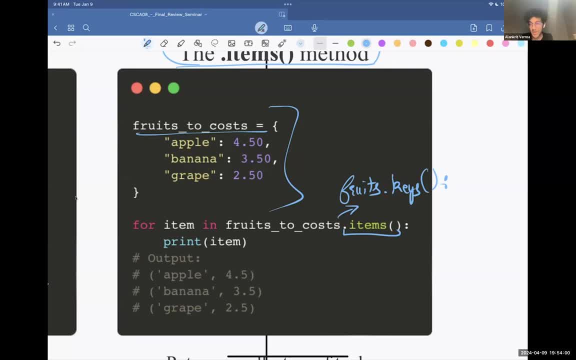 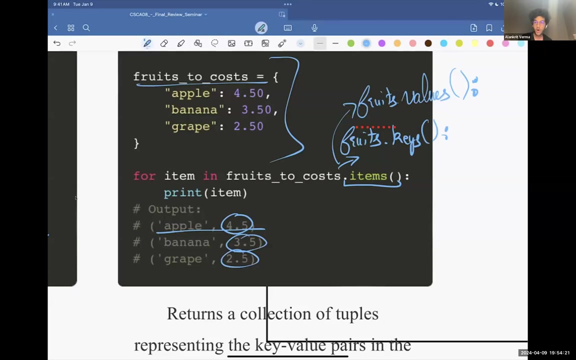 So that would be in some sense, or no, the items. sorry, the items would give you the whole thing. Then there is something as keys and there's something as truth dot value. So that would only give you this thing: 4.5, 3.5,, 2.5.. Also another way of dealing with. 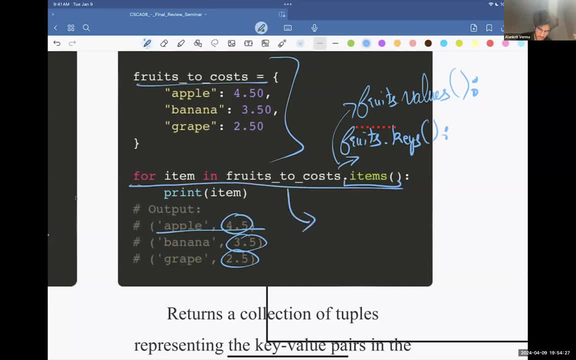 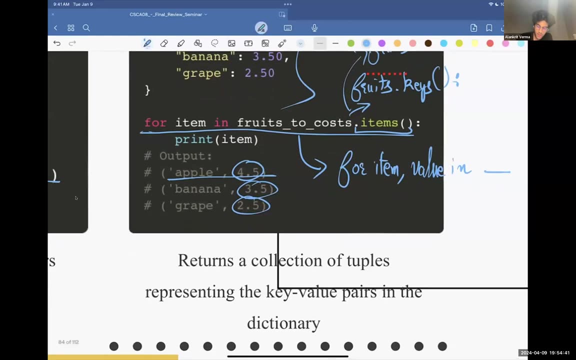 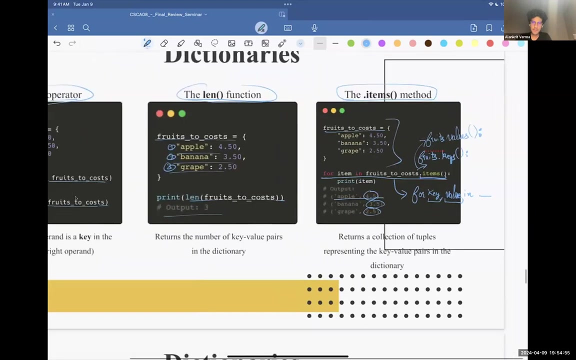 these items is, rather than using a loop like this, you can change it to make for item comma value in the same thing. So then that will mean your value value is directly initialized to this variable and your item is directly initialized to this. yeah, it's just a variable. that is this clear. 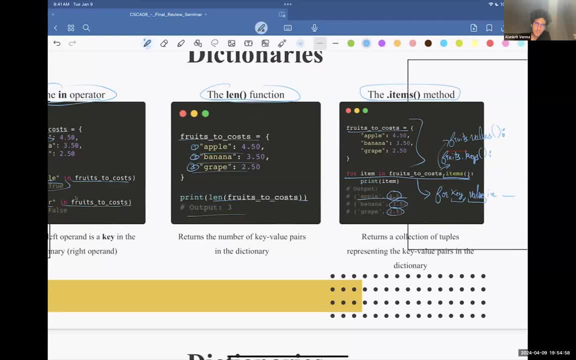 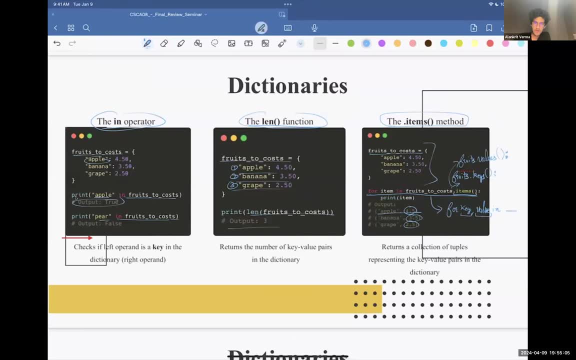 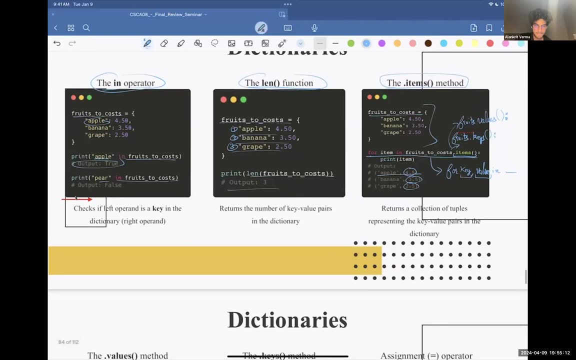 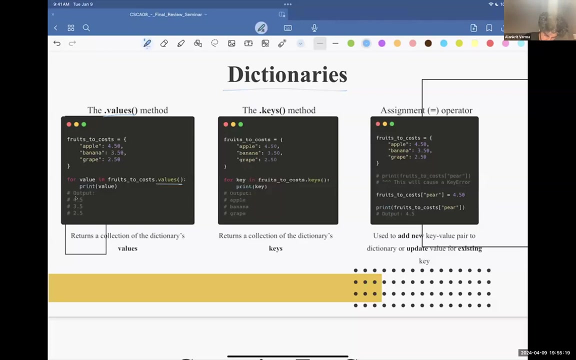 yeah, if this is not clear, do you have any doubts? just unmute yourself and please ask them. if not, okay, let's move on to the next one: dictionary. dot values, as we discussed, allows us to loop through all the values. dot keys: allows us to loop through all the keys. 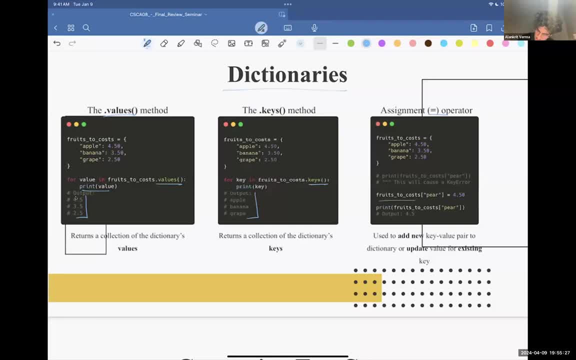 accessibility Assignment operator checks if this thing is having or creates a new item or creates a new key in the dictionary with the corresponding value. So if I'm doing something like here with 4.5, then what is happening? I'm adding this key value pair to the dictionary. 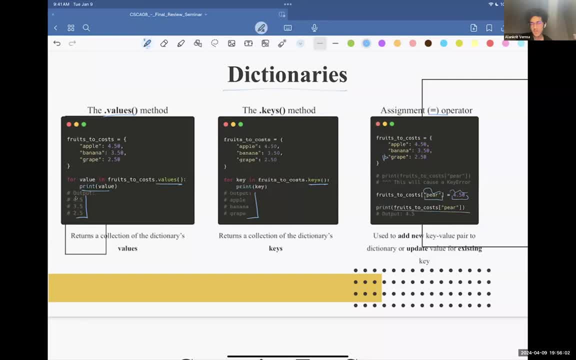 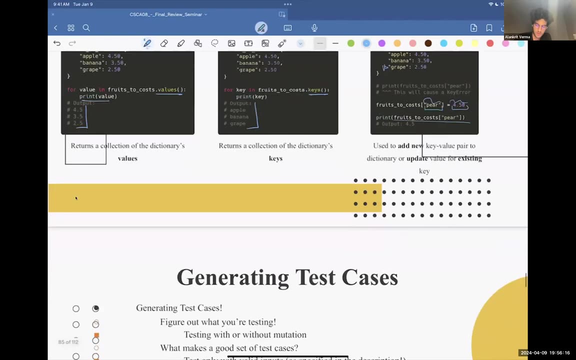 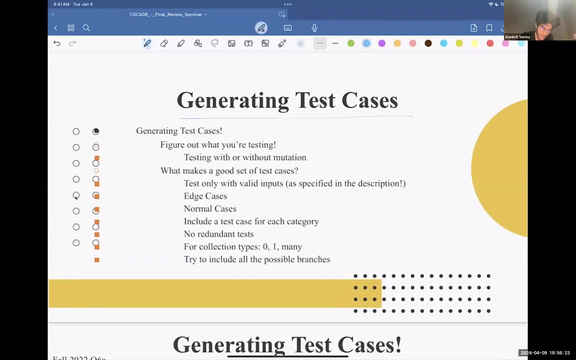 and then I'm trying to print it later on with the key here. The value for this would be 4.5.. Is this clear? It's touching close on something. OK, I'm assuming this is clear, hopefully. OK, test case is this should be quick. 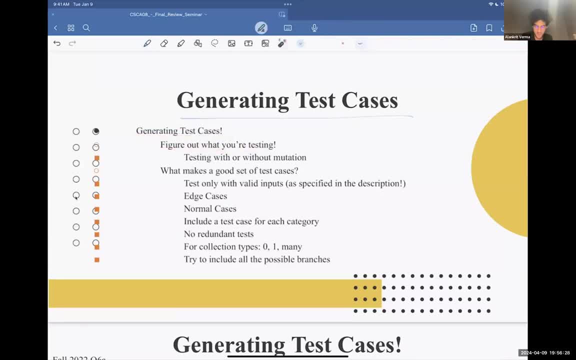 Generating test cases. figure out what you're testing. that's the first thing: Testing with or without mutation, what makes a good set of test cases? This is just text and I want you all to read through this in 30 seconds. 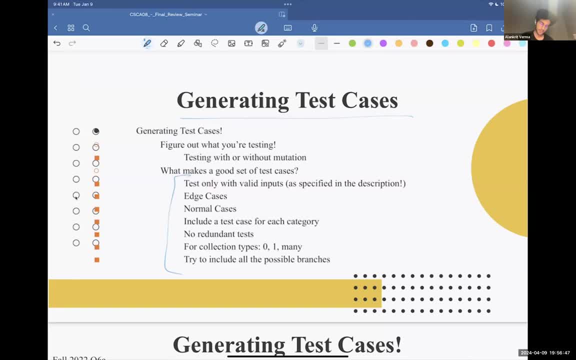 There's no point in me reading it and then? OK, so what I'm going to do is I'm going to upload this test case And then I'm going to stand in front of the camera And I'll be doing the same thing, like this. 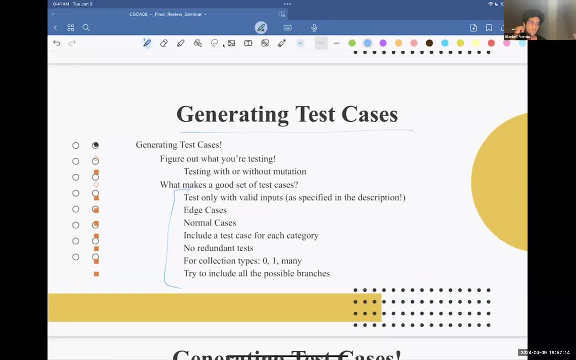 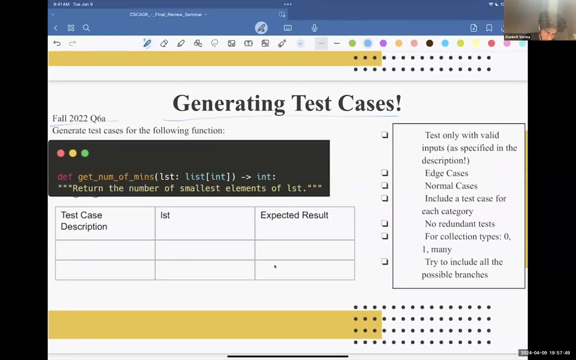 And then I'm just going to move this And that's it, And then I'm going to have this test case installed And then I'm going to go ahead and launch this. Done. let's move on generating test cases. this is a old test person generating test cases. 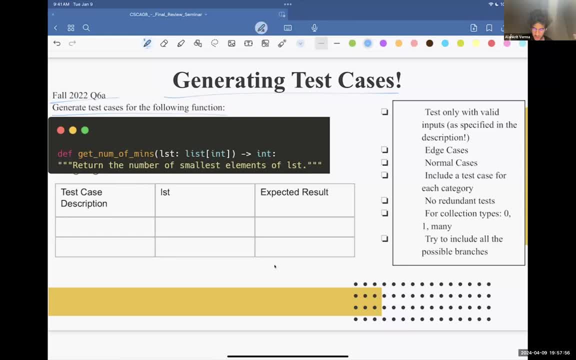 try this for the next, uh, one minute. let's think as to what can you write here, and this can be a template that you can follow for your test cases. okay, a person asked me: would we be requested to write unit test as well? uh, not, like you will just be asked to write the generic test cases. 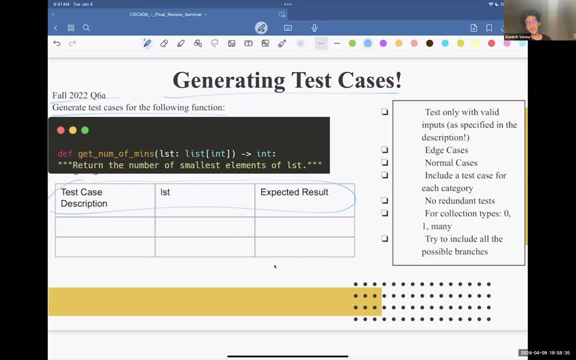 in which, uh, in some sense we can cover the edge cases for that very question. so, yeah, we'll go over the edge cases, edge test cases. this is a very important table, so let's take a screenshot of this if we want. this will be posted. yeah, this will be. 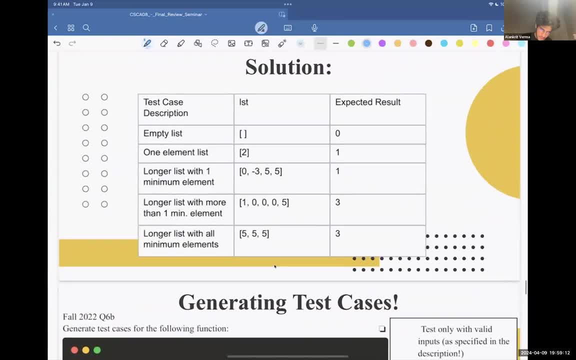 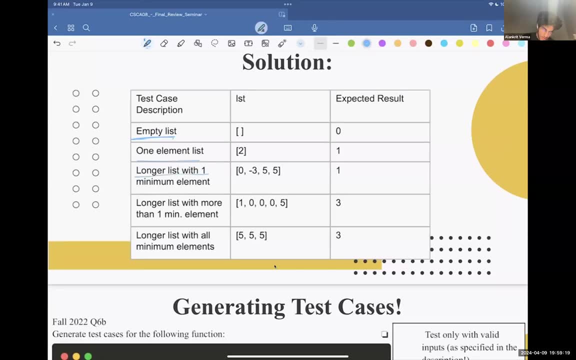 probably is the only thing you need to know for testing. okay, uh, this is the solution. we consider an empty list, which is always there. one less longer uh list with one minimum element. okay, yeah, with more than one min. so, yeah, three, that's one, and with all of them as you can. so see, this is a good test suit out of three. 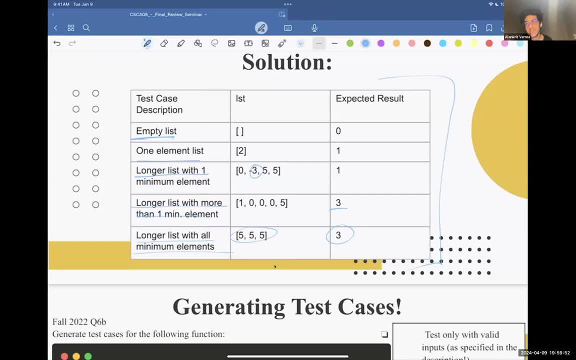 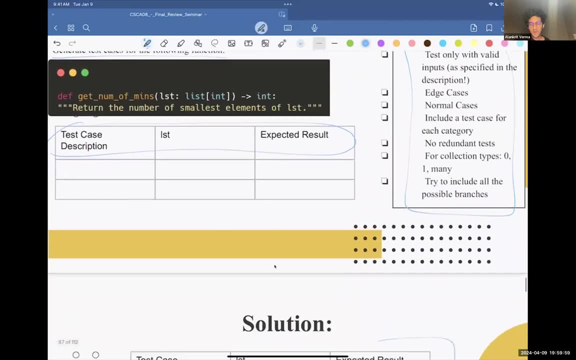 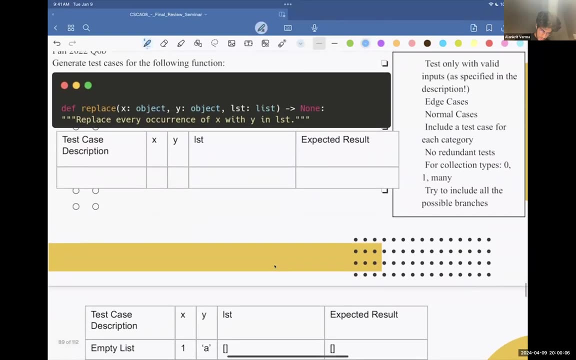 yeah, the thing with test cases is like it's probably the easiest question. on the final, if you understand this table and you're able to like think on spot, you should be good to go. just make sure you're uh writing the description very properly. okay, uh, you can go over this. 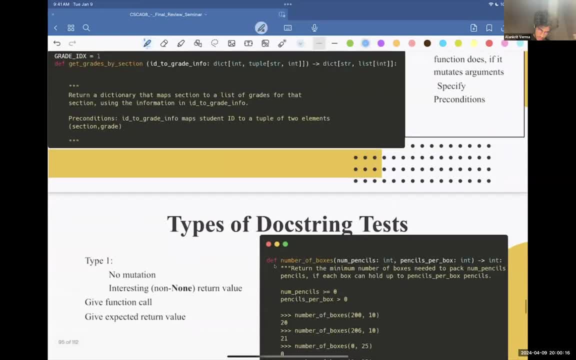 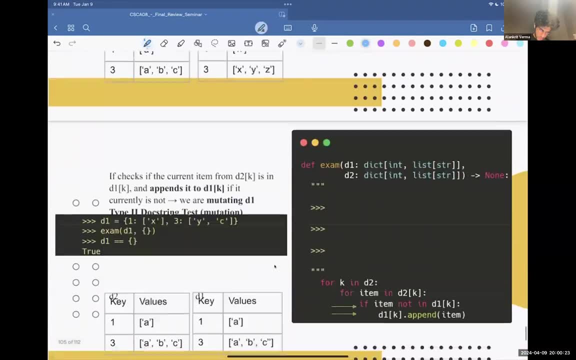 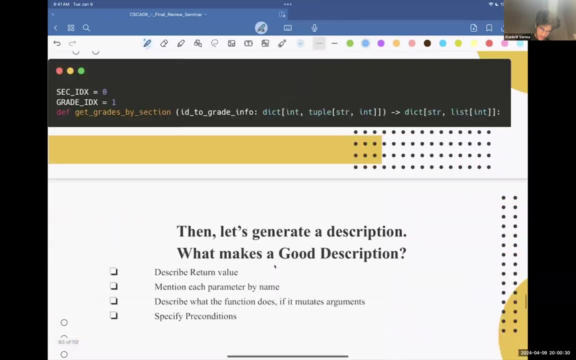 quickly. this is really easy. so the first thing you need to do is you need to go to the table, here, here, under the table, and then you need to do this like this: okay, that's about it. okay, uh, okay, oh, okay. always stop before the next time that I go down time. yeah, okay, this is the last. 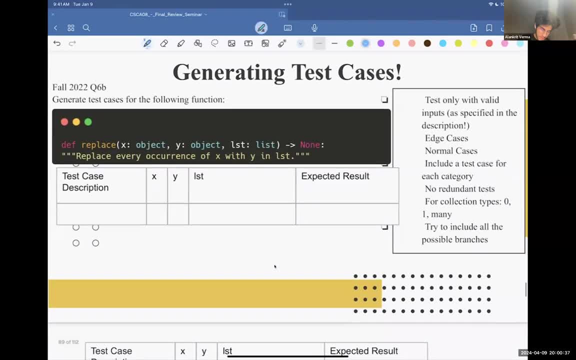 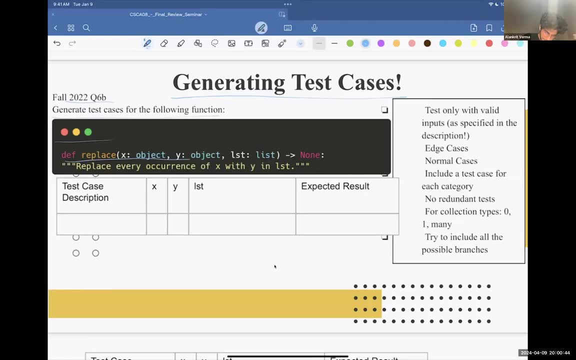 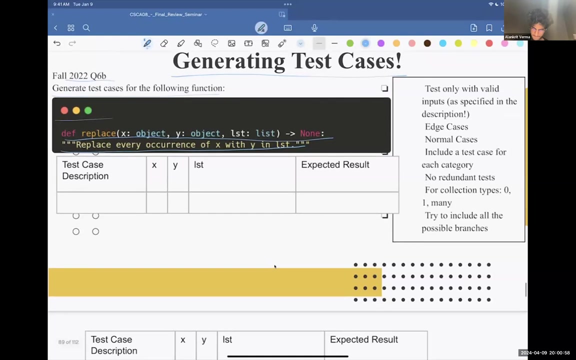 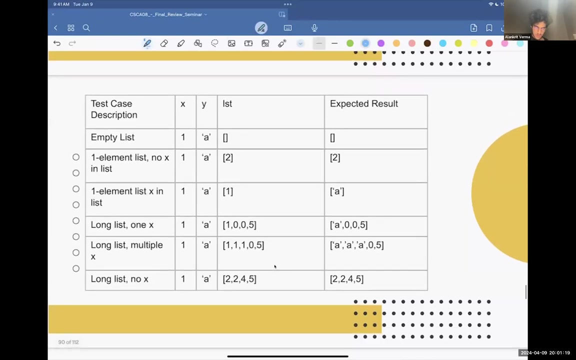 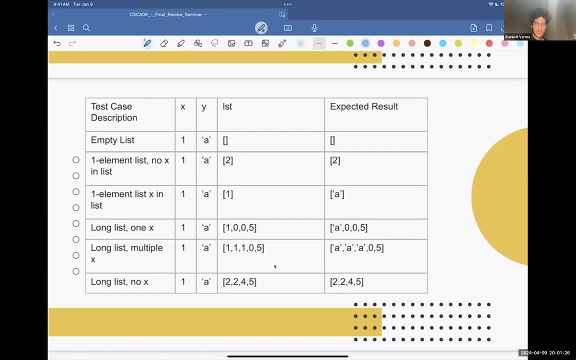 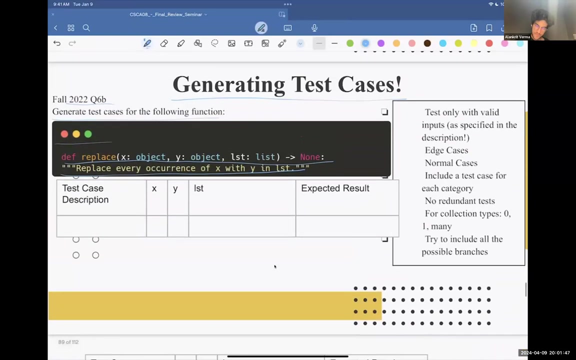 question often the generating test cases. try this one and take a screenshot and remember this thing. okay, we are on time. let me just share the solution. this is the solution. does anybody have any doubt for the theme? yes, no, could I see the question? so the order is basically same. you Always have a empty list, one list with no x, 1 list diligently depends on how high you listen to this. 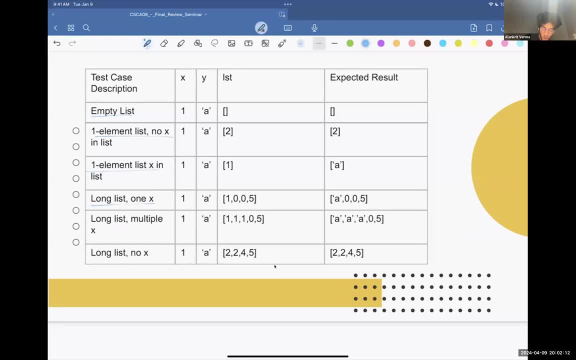 suffering. so the order is basically same. you always have a empty list, one list with no x, one list for the x and 2 longer than x long list. multiple x long list, no X. so the if it you clear the logical wishes, swear to god and yeah, that's accepted. then the handset course, you still have an empty list. currently. take the list you wish, you can do it any number as many your aks. so, yeah, you have to do a new listing day one to put a new list a few times, and you always do it against yourself. if you dare even think so on this next week or even to find the next question from is helpful. V mentor. 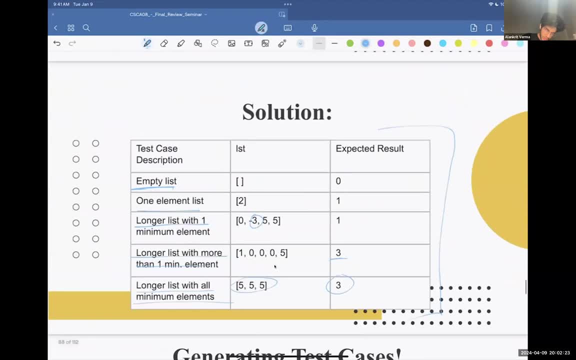 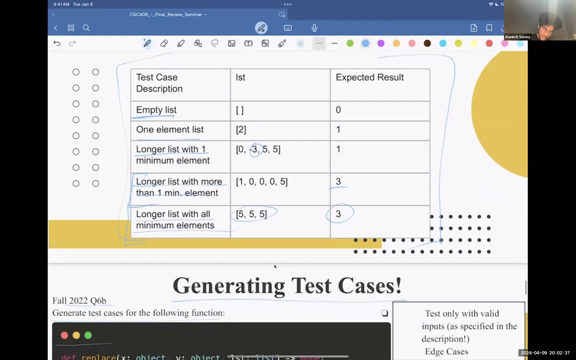 if you, if you compare this solution with the solution here, empty one more than one, and then this is a special case with longer, with multiple mins, and then there is one with all of them as mins. so the generic idea for writing test cases remains the same for all questions, which is something like this very important. 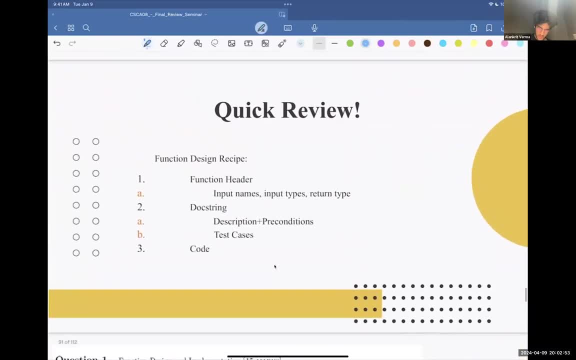 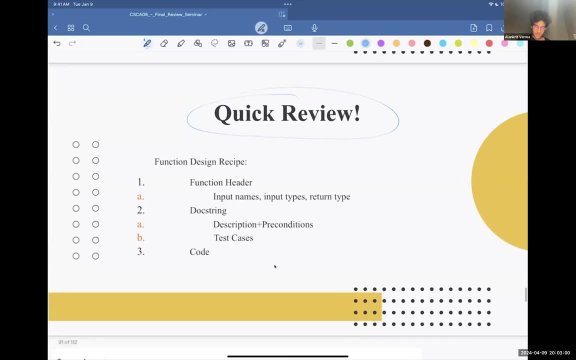 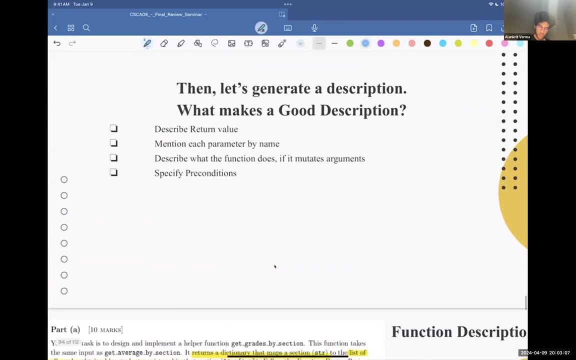 okay, now we have more stuff here. this is all about your mix-and-one syllabus. you're not only gonna cover this right now, but the slides will be posted and you are recommended to go through them. the answers are attached to it. yeah, we covered, doc sprinter. a lot of people have. 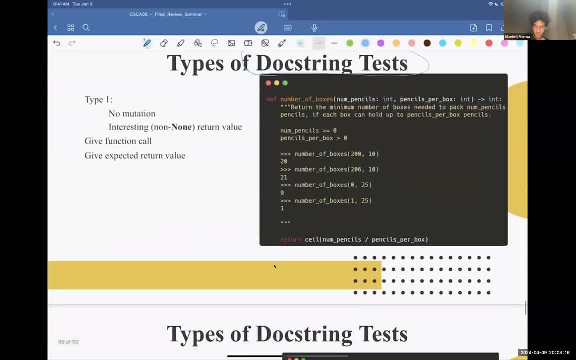 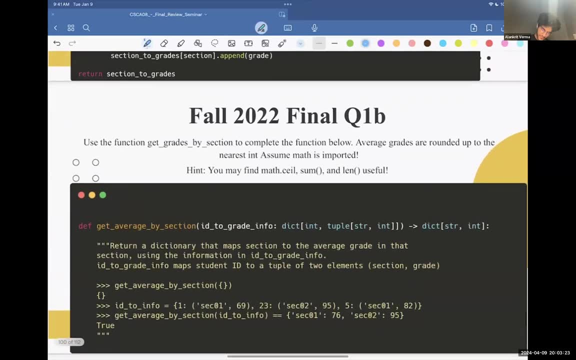 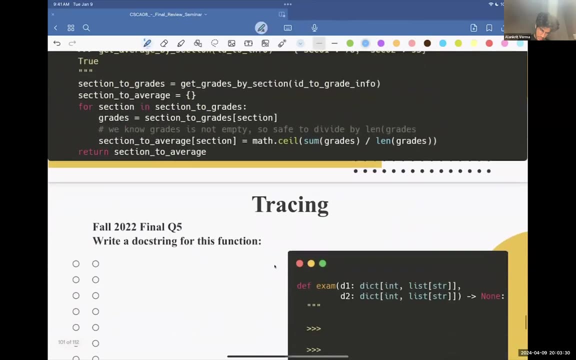 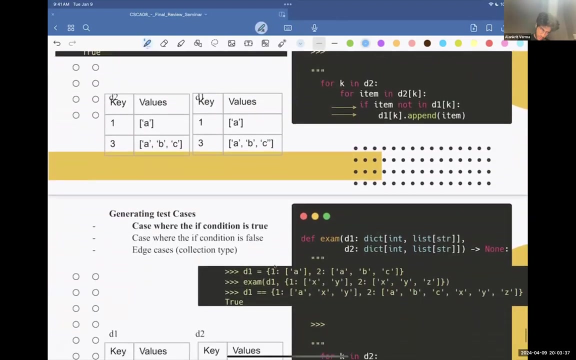 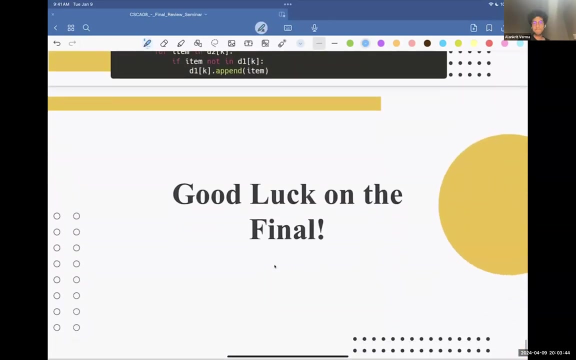 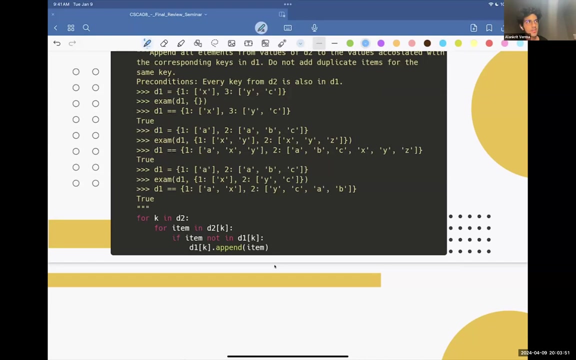 questions about options, as to how to write the options, so this should serve the ultimate attempt at writing the options. let me see if we have any good questions here. all covered earlier. yeah, okay, so the slides will be posted. review: the quick review slide and the last ten slides because we didn't cover them properly. but other than that, good. 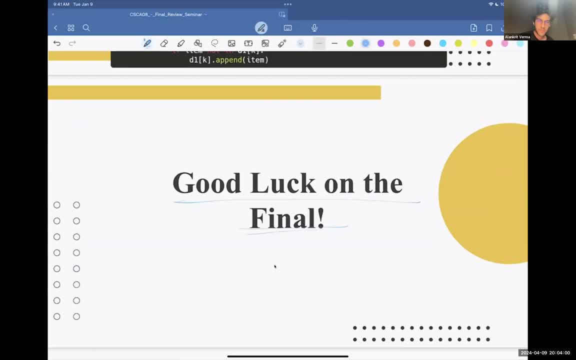 luck on your final. remember the passcode for this zoom meeting, which was: I hope everybody gets this- everybody just say 100 and final right now, and not in chat, but in voice: yeah, no, 100 and final. yeah. and more people said the thing is a wait. final is gonna be this: 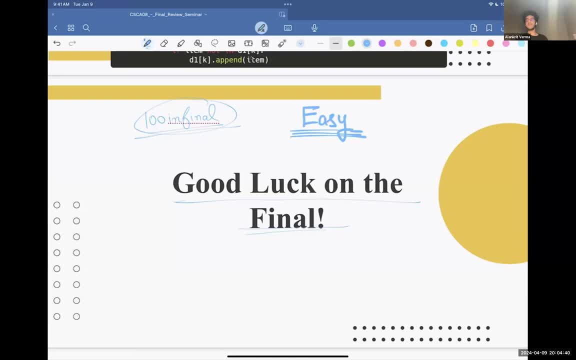 it is very easy, but you need a very good presence of mind if you review your midterm solution or not midterm solution. if you review your midterm feedback on your midterm, you'll realize you know most of the questions. but in the exam you sit there, you think about the solution and you're like I 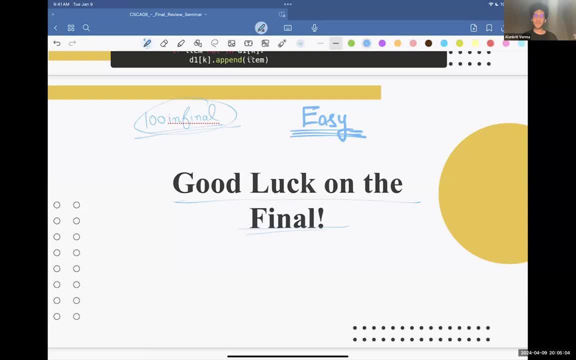 don't know this, but if you think twice, you think thrice for the same question. sometimes just reading the question helps. you'll get this: yeah, and testing 100 and final. oh yeah, and we have more 100 in the final right now. this is the last. 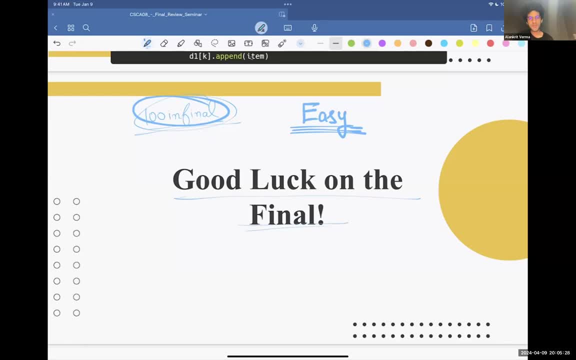 component of the review seminar. you guys should think better of yourself and keep that presence of mind in the final- and I will just post the slides right now- on piyadja. the slides will be posted on piyadja everybody, So keep a check on that.